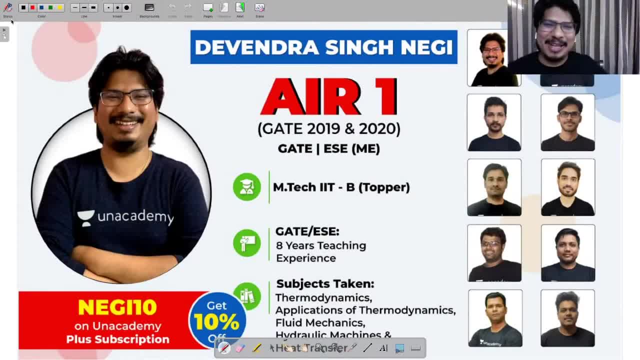 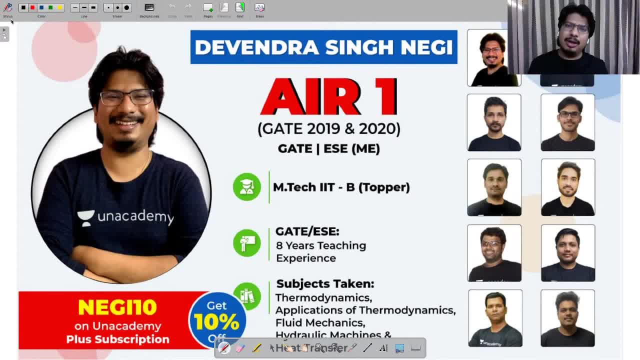 Those who are coming first time to our YouTube channel, my friends, let me introduce myself. I am Devendra Singh Negi. I completed my MTech from IIT Bombay. I was a topper of my batch. I am teaching for Gate and ESC since 8 years- The thermal and fluid sciences part. I am teaching And if you see Gate All India Rank 1, 2019 and 2020 in engineering sciences paper as thermodynamics and fluid mechanics as subjects. 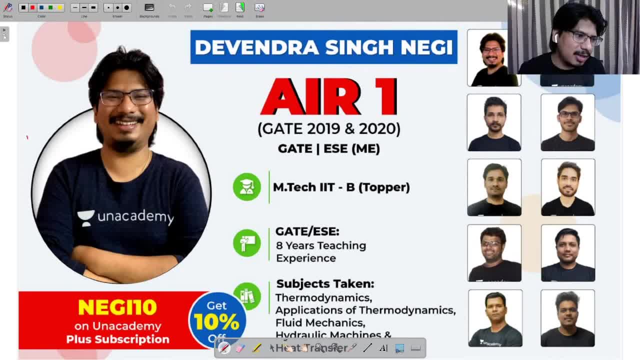 So I am leading this team- You must be observing, my friends- is the best and biggest team right now on youtube channel: total 10 educators are serving you. so i'm leading the team of an academy brands mechanical. okay. so, uh, today we are going to start convection. 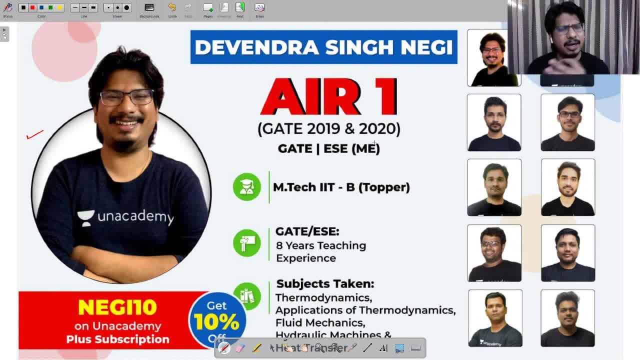 part. so last month i have discussed thermal radiations. now, today, we are going to start convection part, according to your demand. so many students message me, sir, convection is very difficult for us, so can you explain? so can you explain? so definitely, my friends, i came forward. 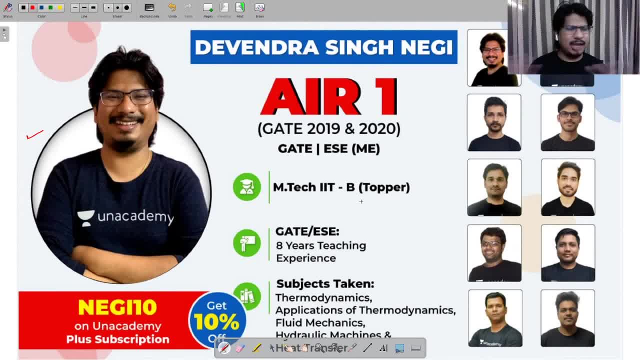 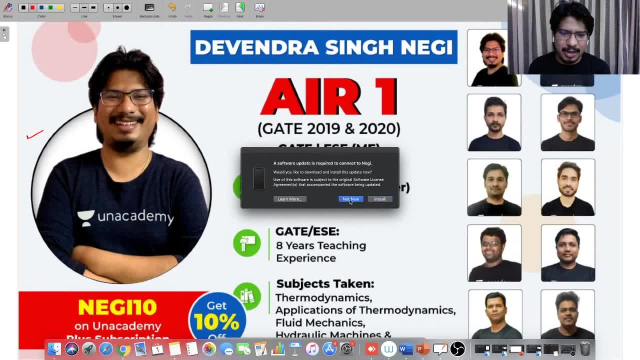 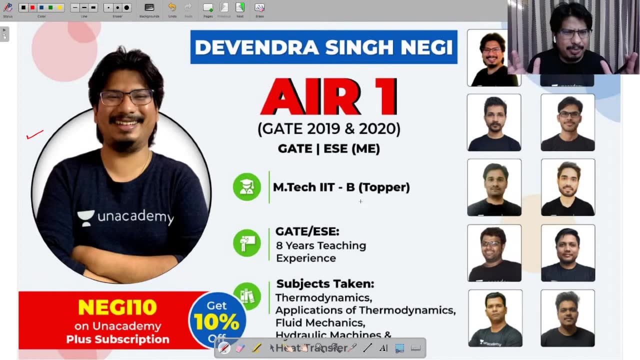 as per your suggestion, i'm starting convection and, whatever you will say, we will do that. the only thing is what i want. i want the support from you people. this, this free education, should be free to each and everyone. okay, okay, okay, let's start. let's start, so, as usual. as usual, those who 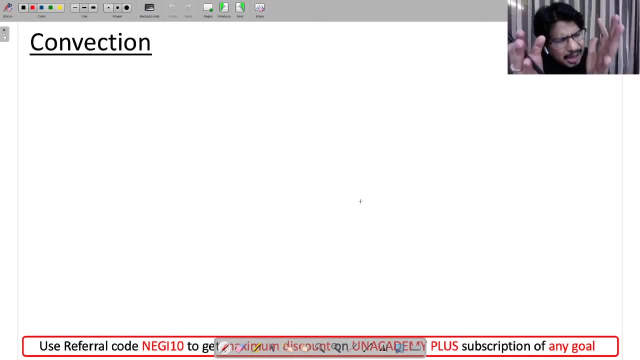 are live. please hit the like button. i i request everyone to hit the like button so that we can move forward. we can move forward. oh my god, oh my god, so many students are live. hit the like button. hit the like button. thank you so much, vikas. thank you so much, vikas. thank you so much. 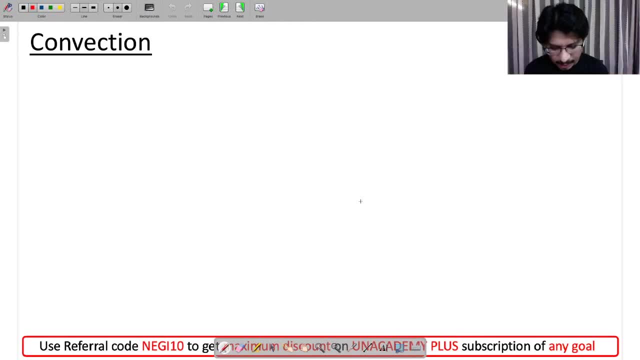 a lot for me. the moment you are saying I am your biggest fan. it means a lot to me. let's go. let's go. let's start the convection. let's go. I hope everyone hit the like button. let's go. everyone has hit the like button. those who are coming first time, kindly. 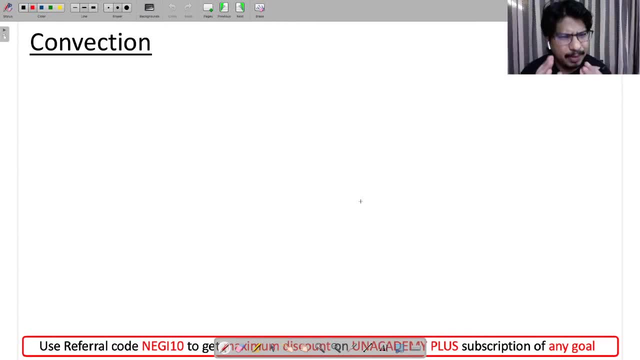 subscribe the channel and hit the like button. let's go now see. before going to convection. before going to convection, I want to discuss a little bit about conduction, because I will try to correlate. so first I want to ask you when someone is saying conduction? 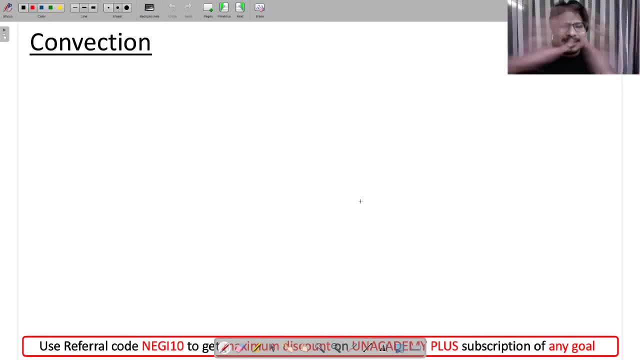 when someone is saying conduction, what comes in your mind? type in chat box. type in chat box. I am observing. I am observing type in chat box. when someone is saying conduction, what comes in your mind when someone is saying: when someone is saying conduction, what comes in your mind? first thing. 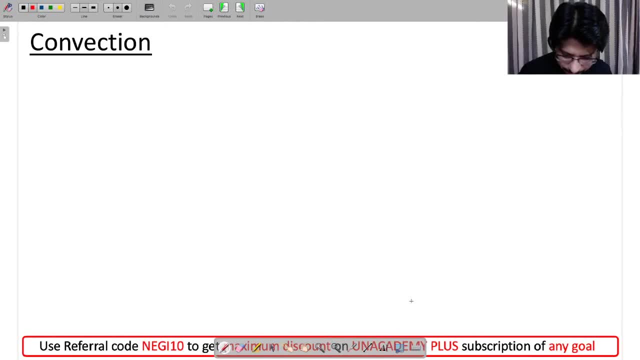 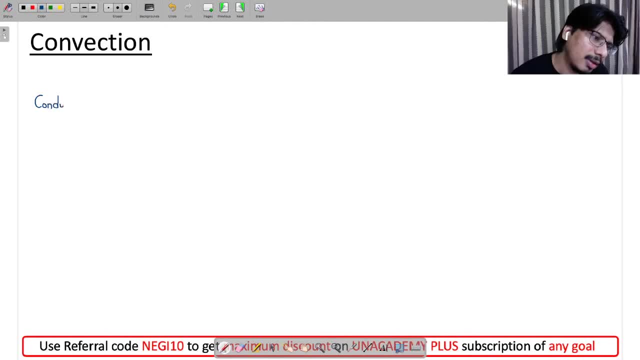 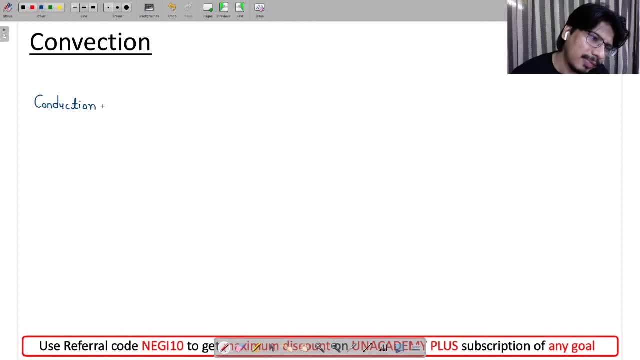 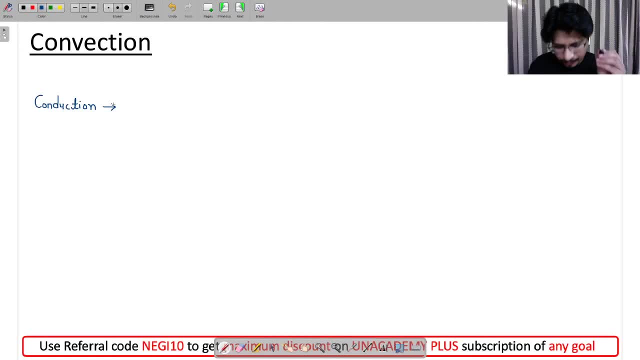 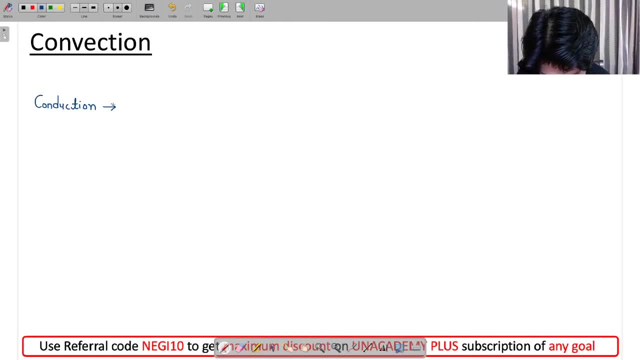 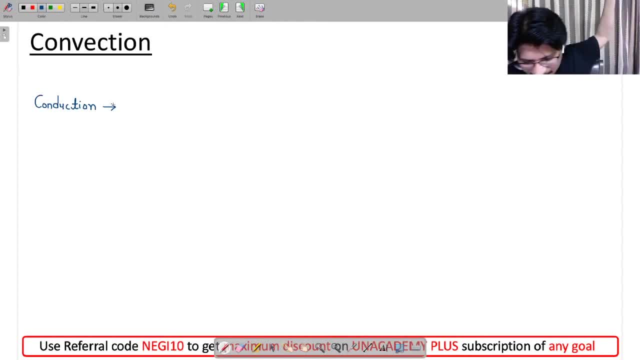 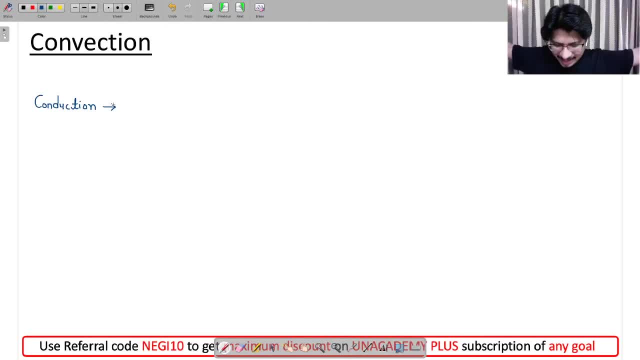 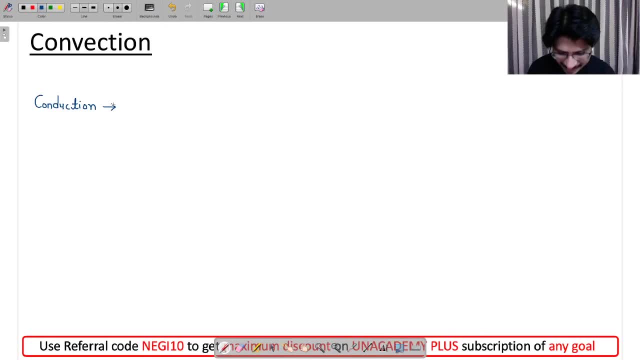 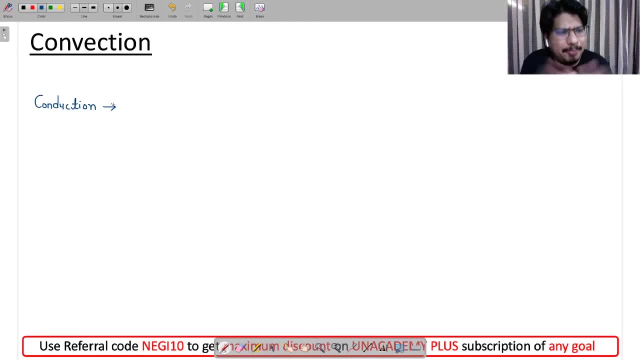 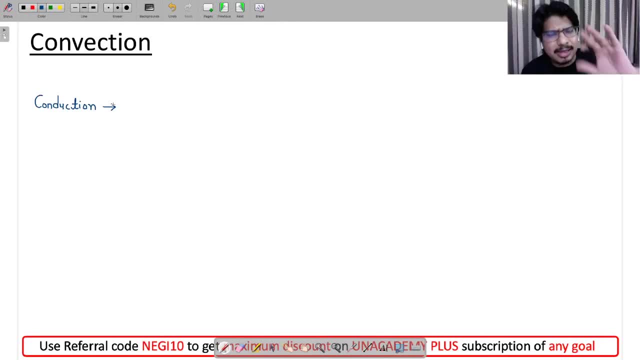 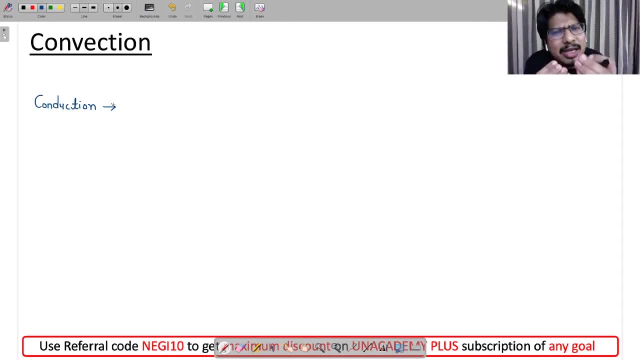 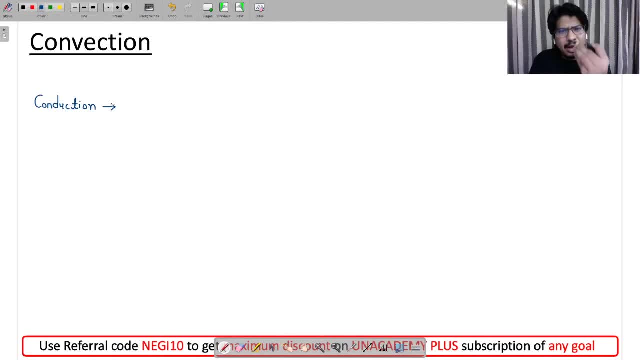 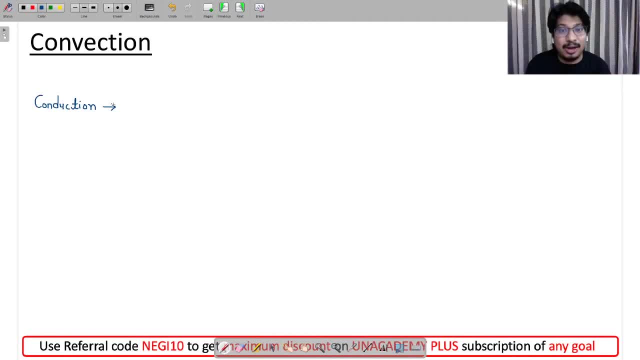 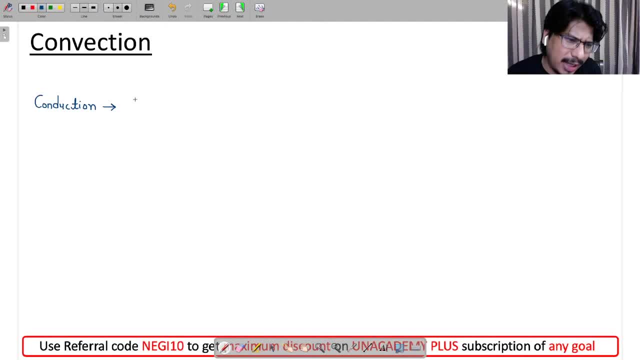 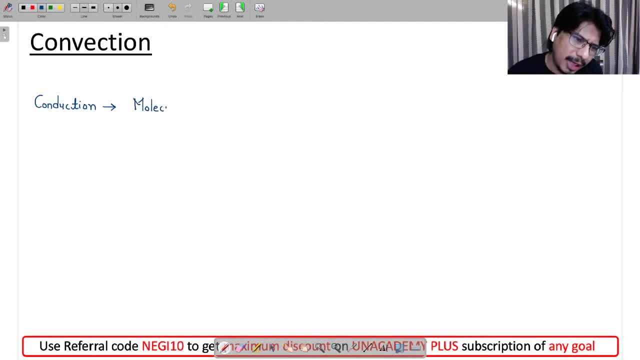 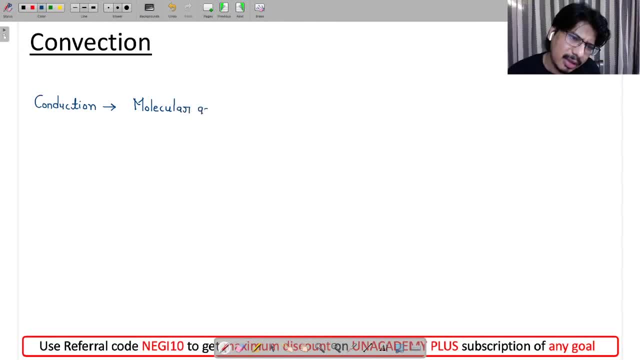 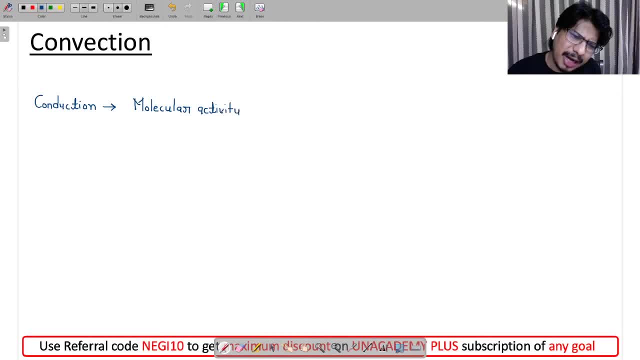 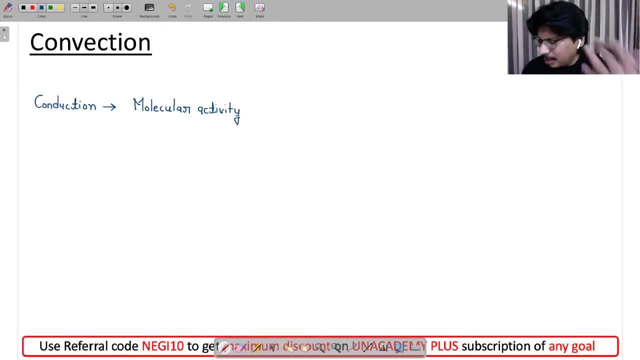 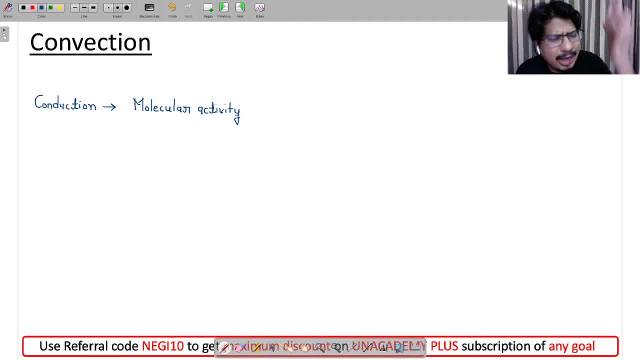 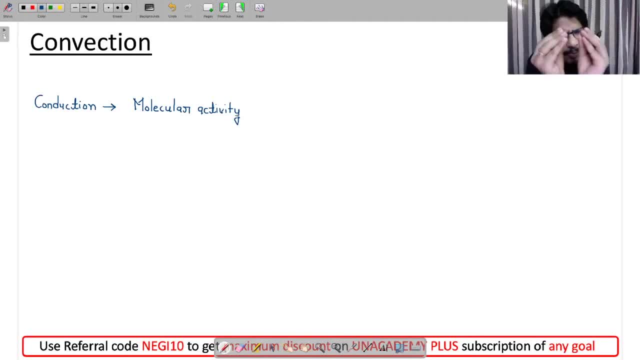 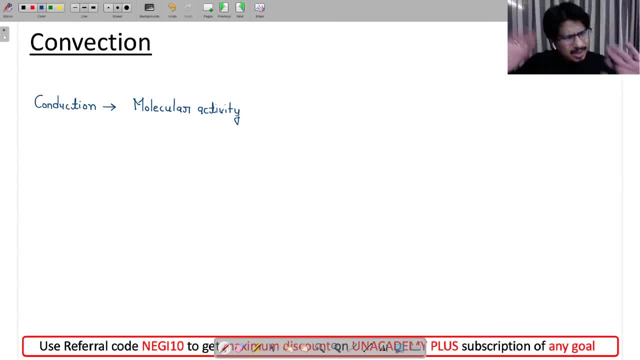 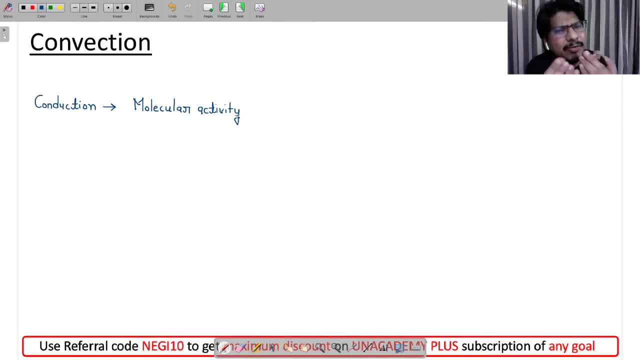 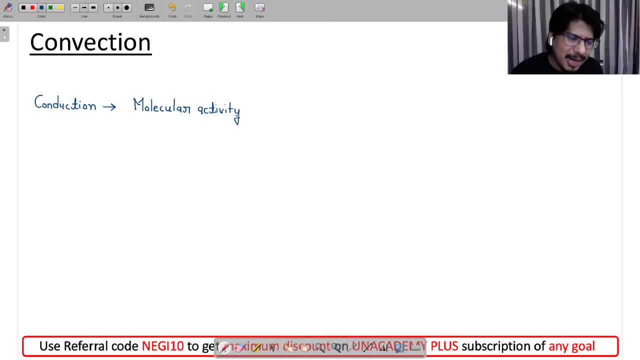 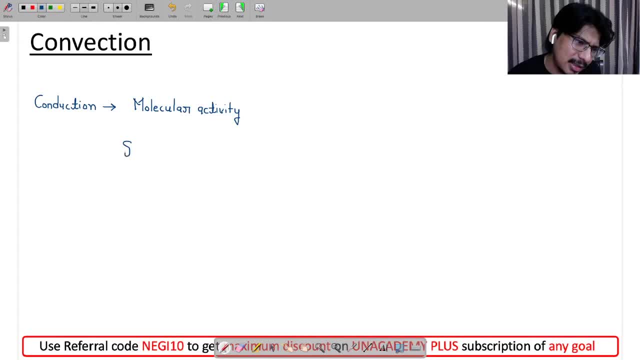 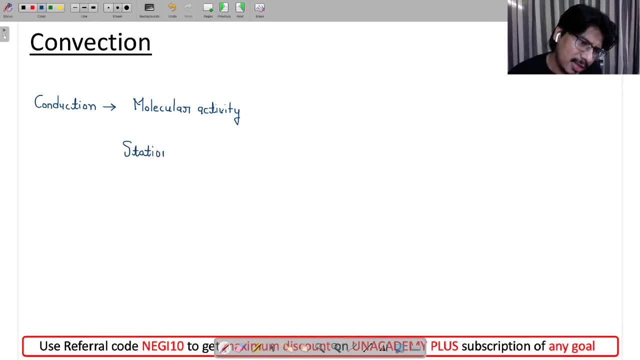 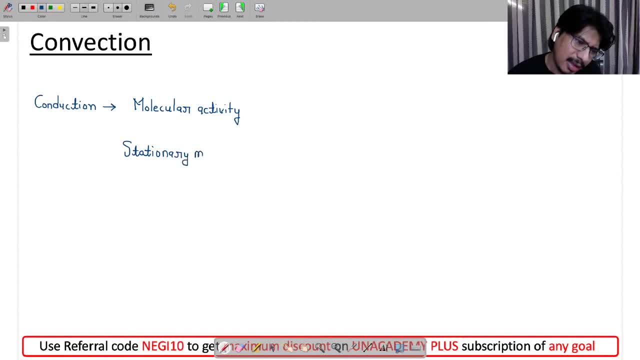 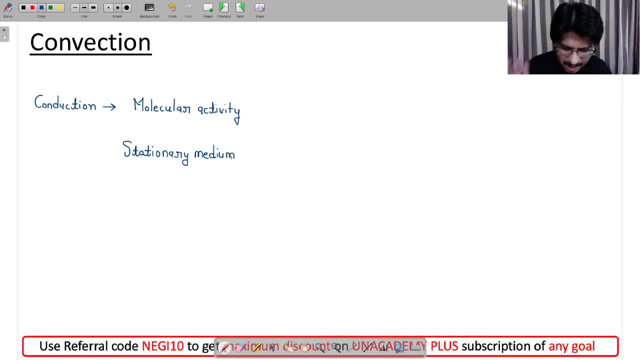 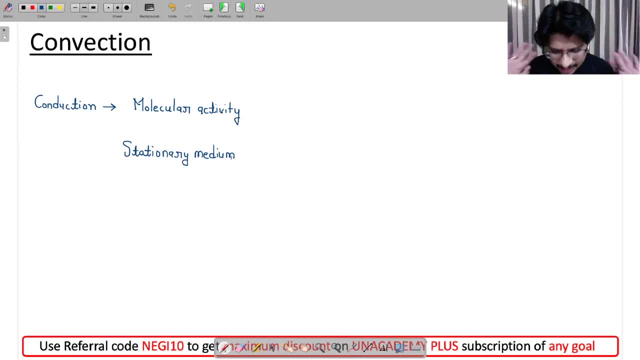 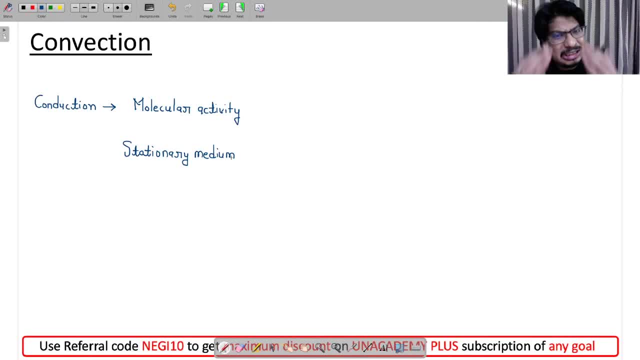 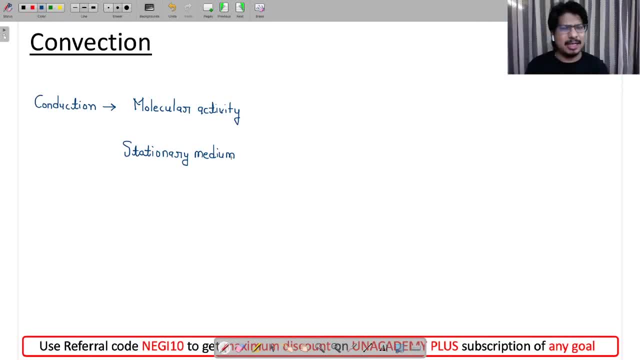 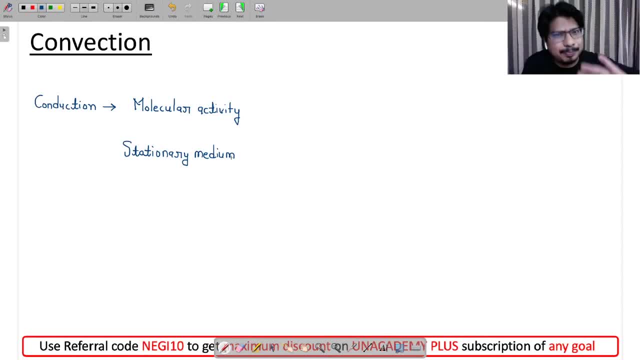 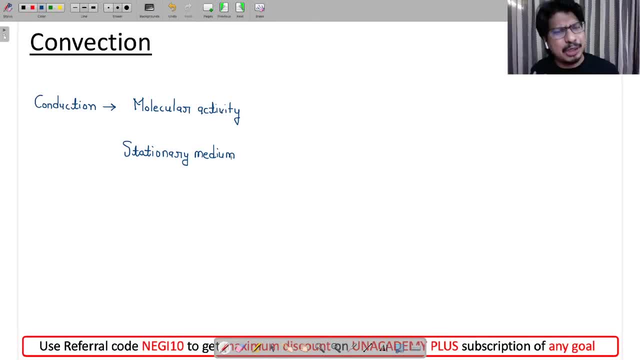 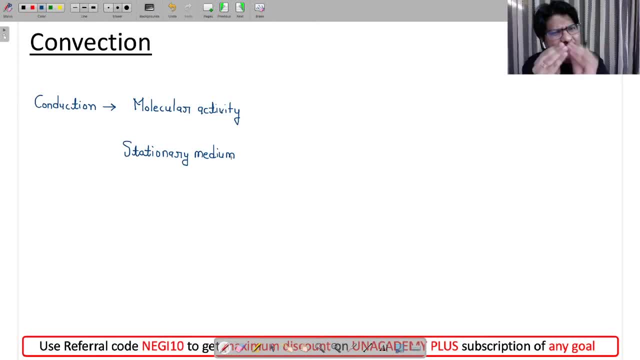 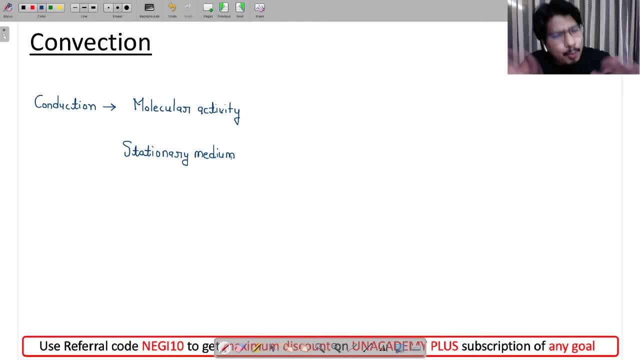 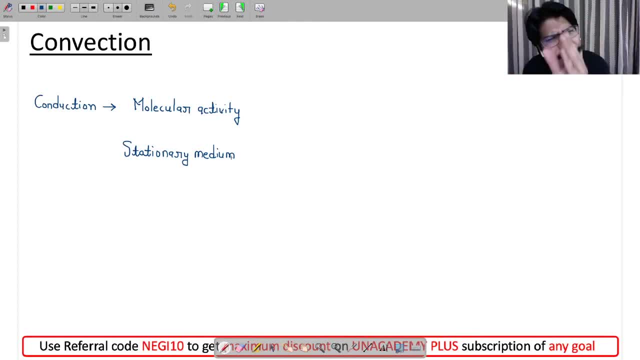 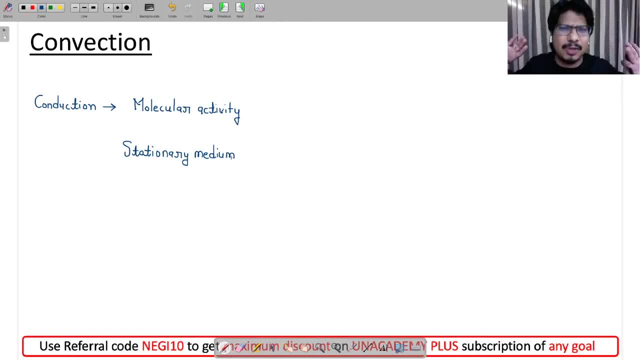 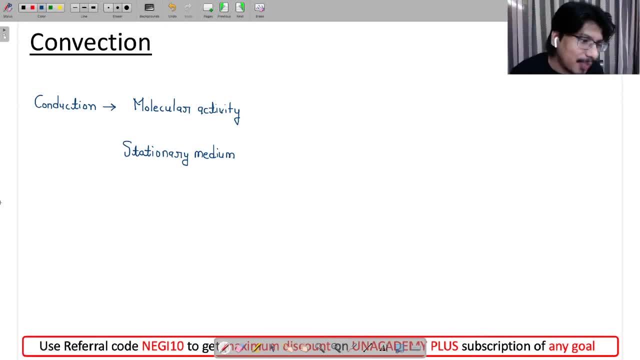 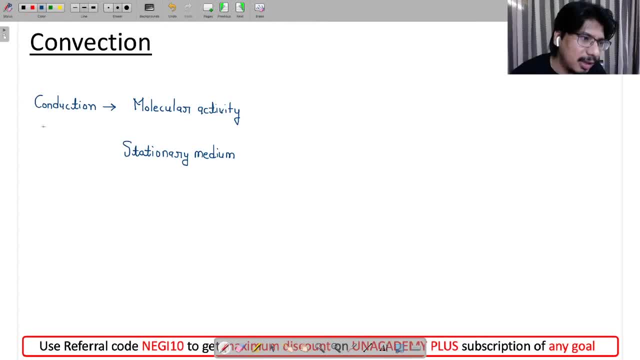 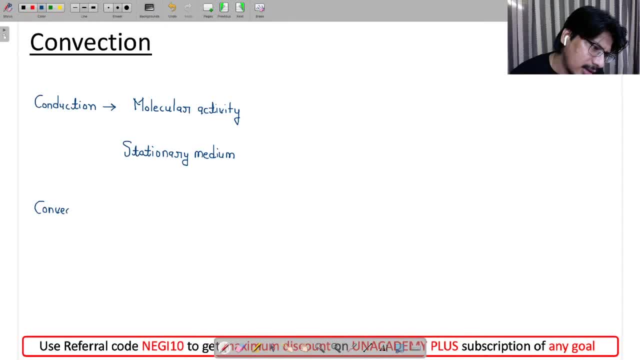 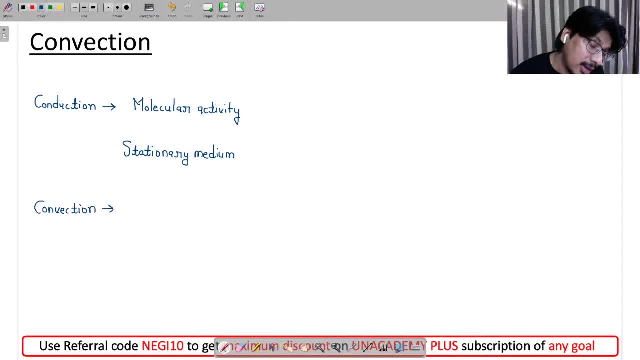 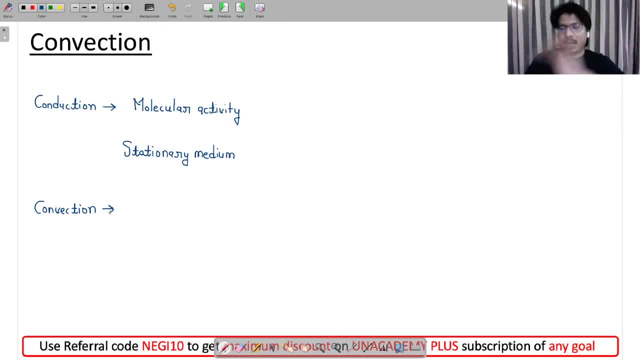 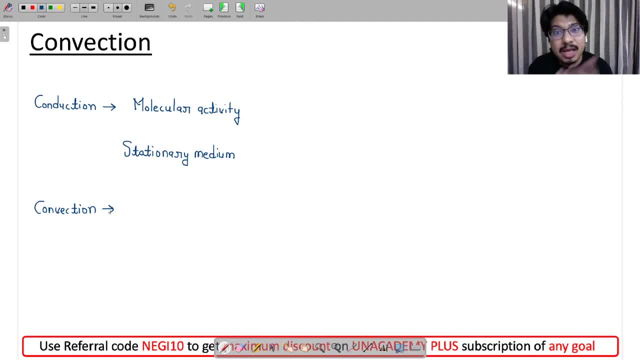 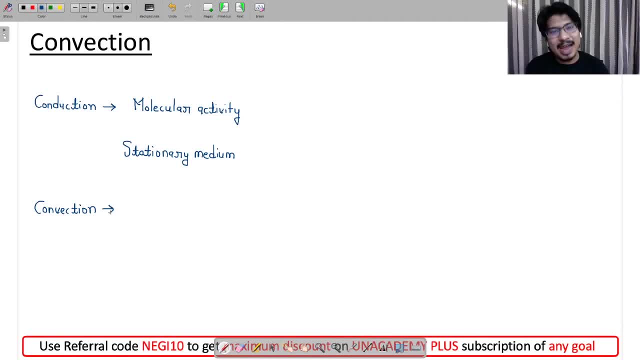 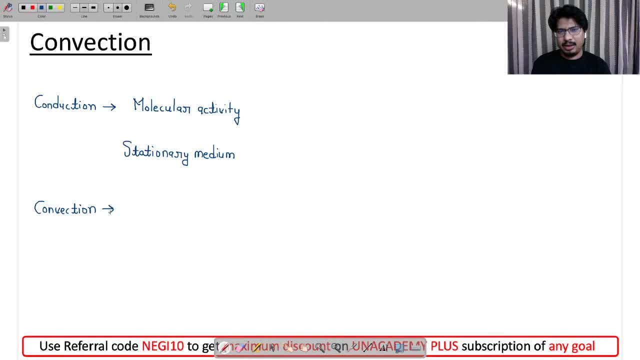 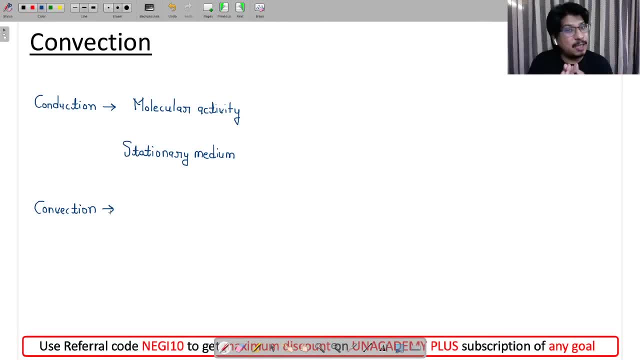 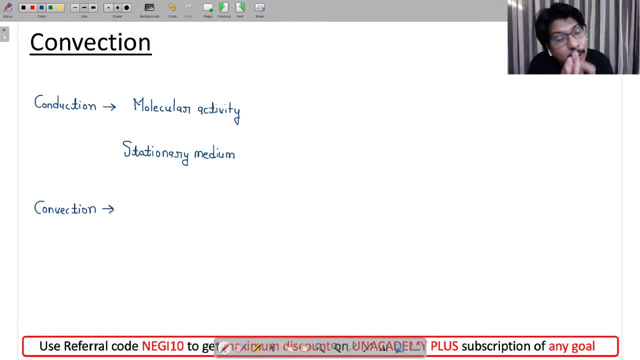 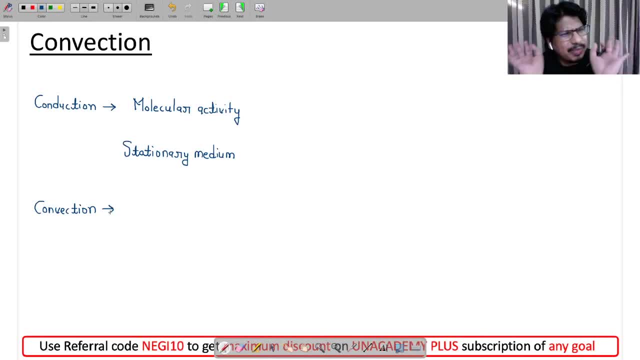 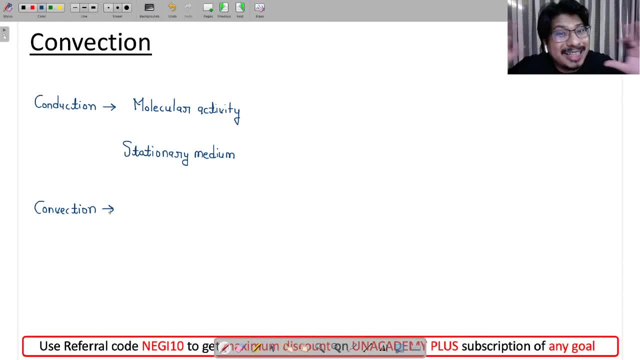 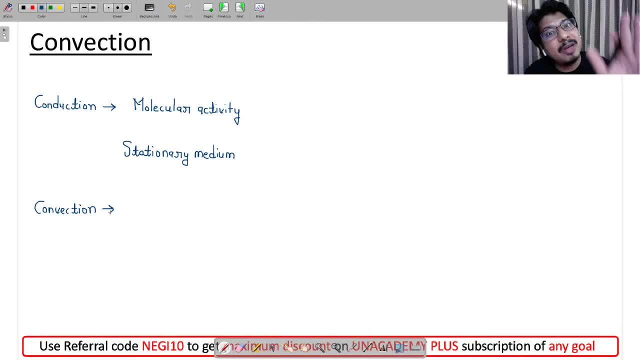 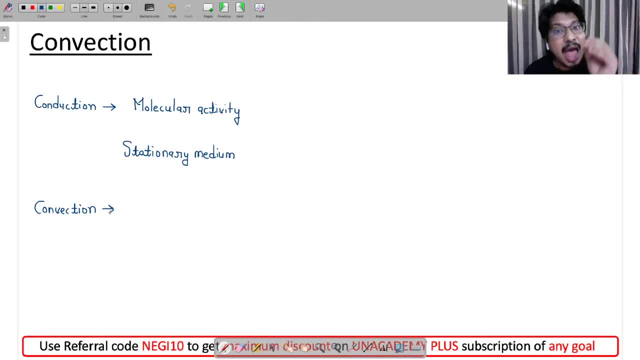 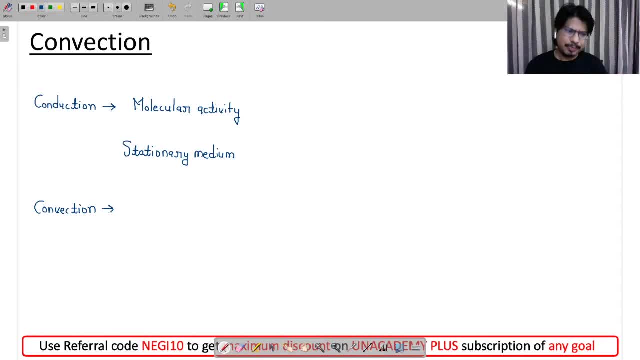 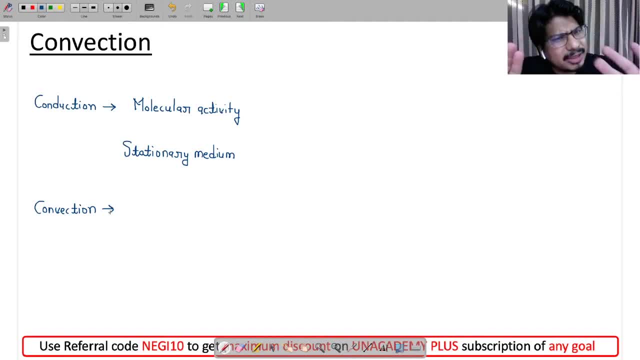 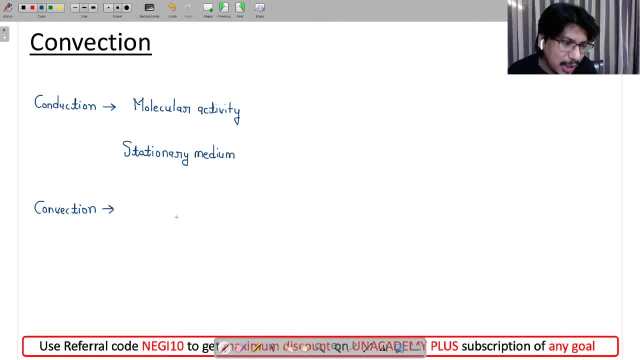 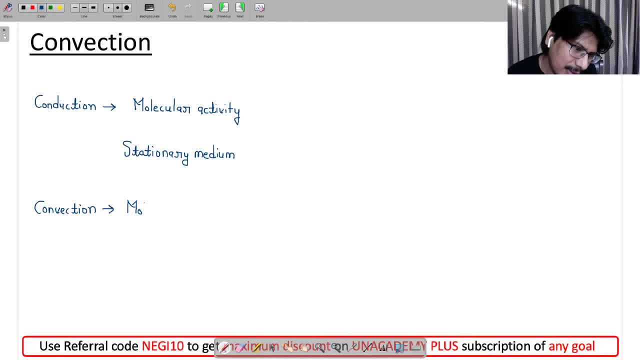 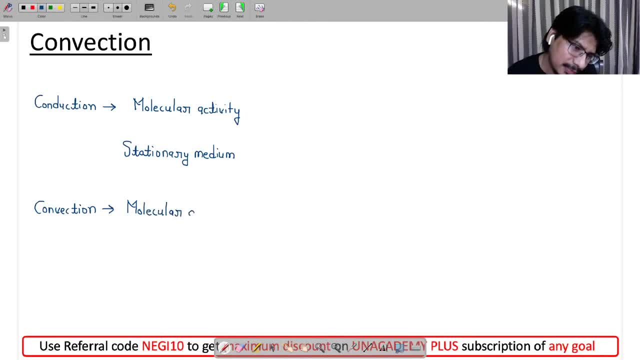 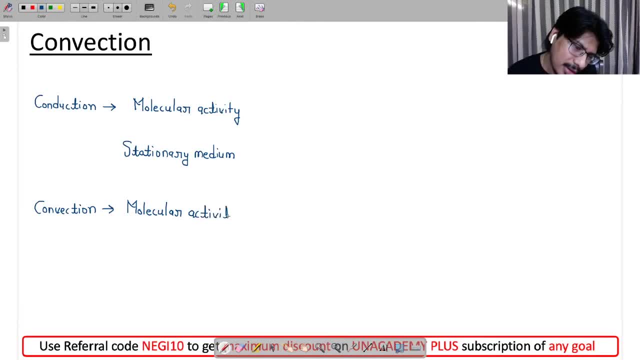 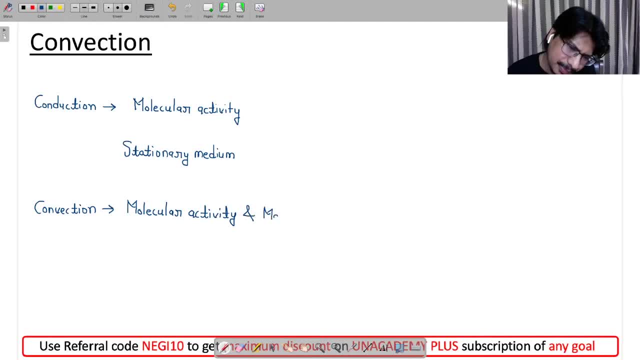 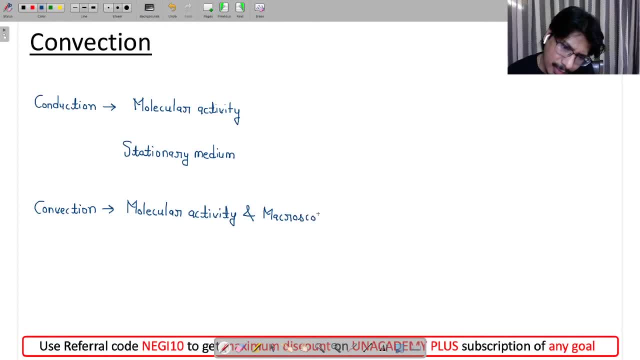 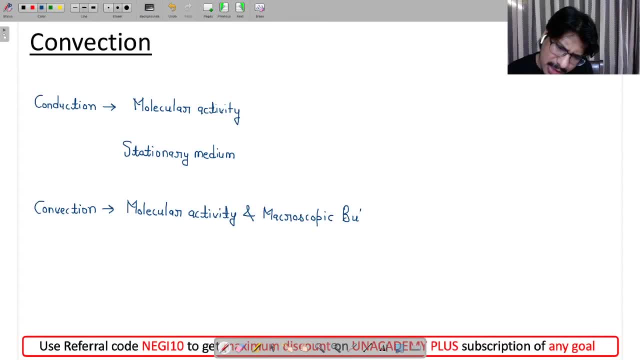 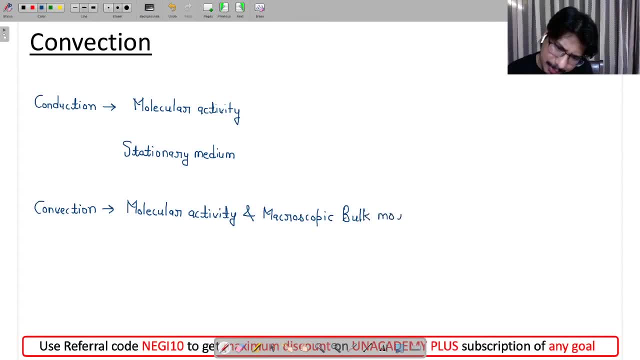 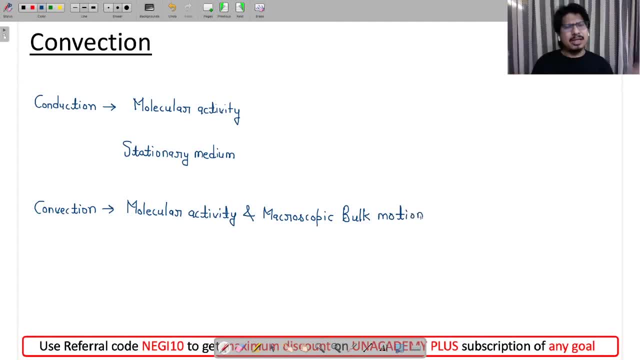 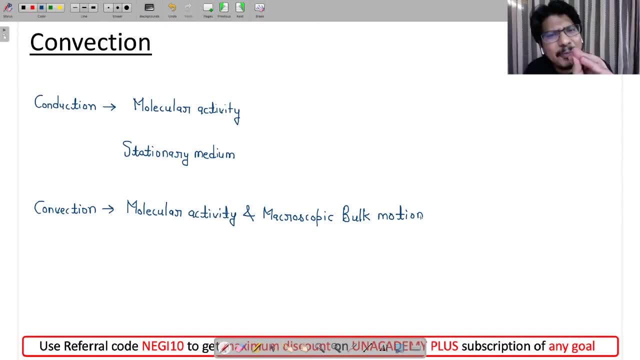 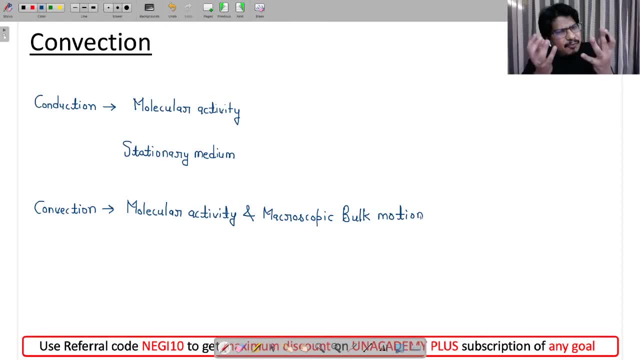 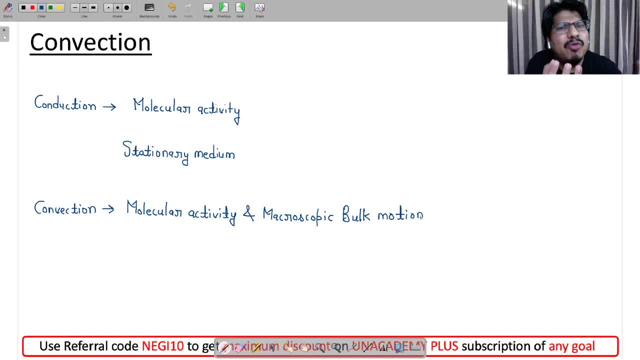 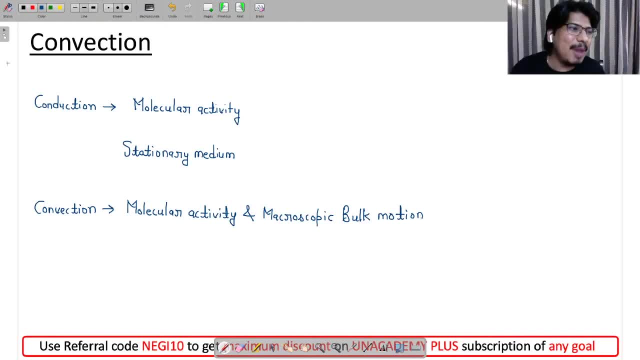 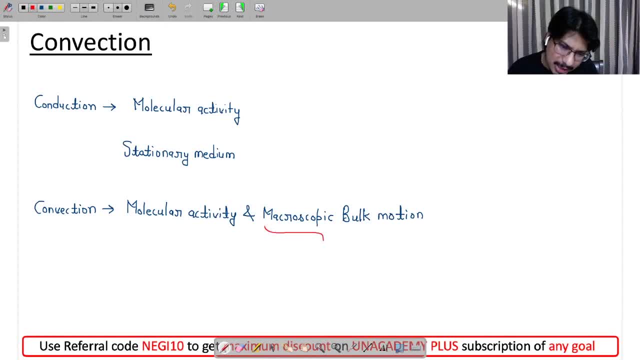 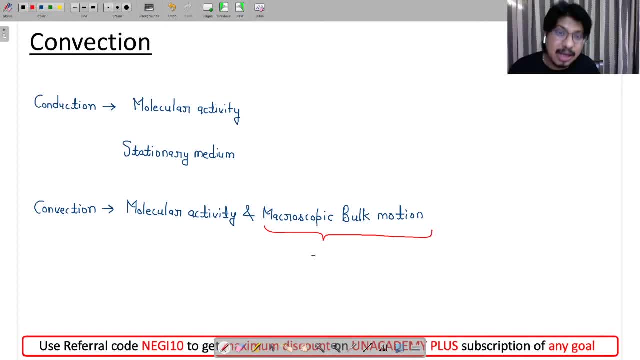 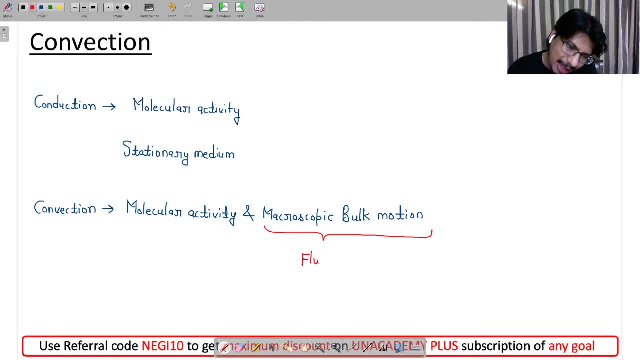 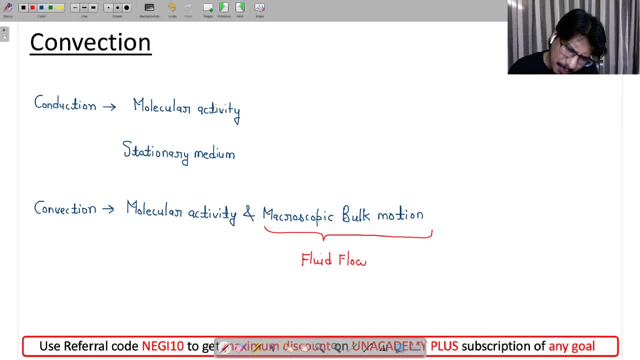 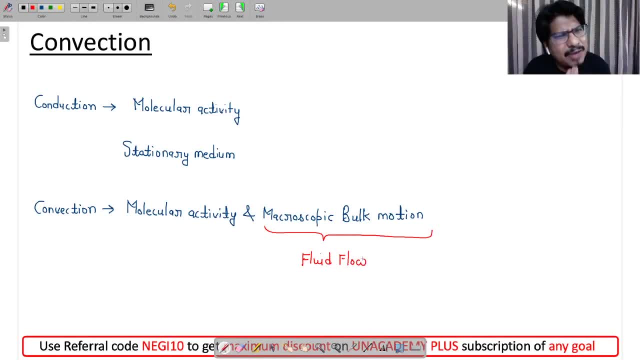 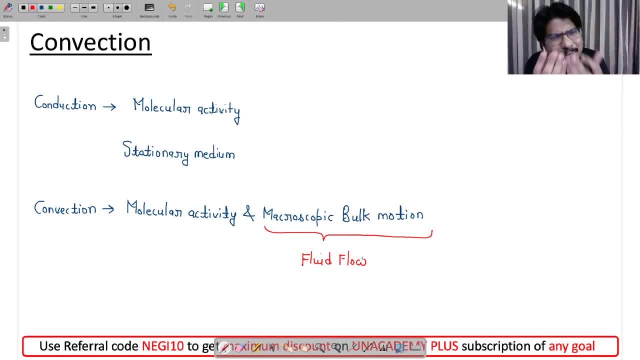 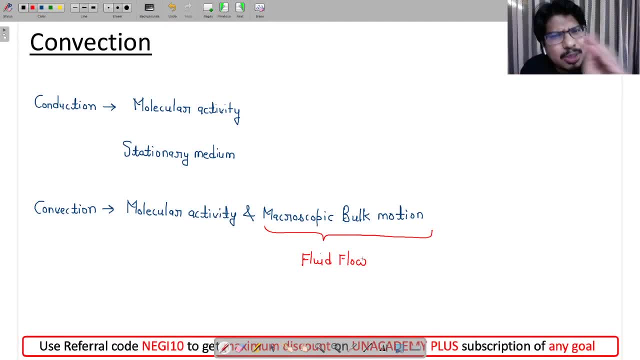 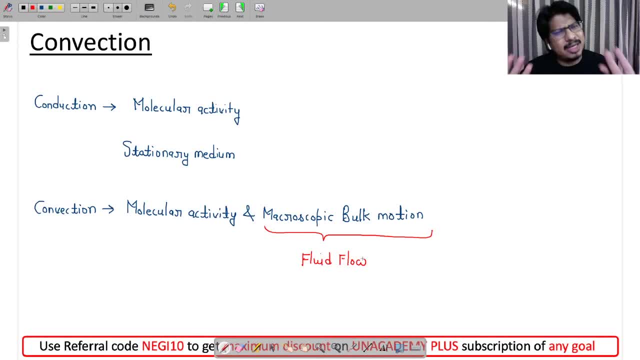 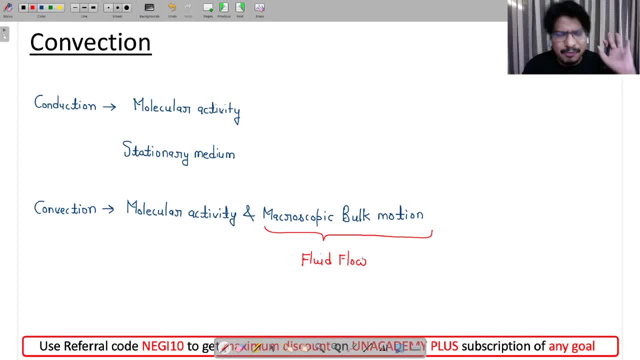 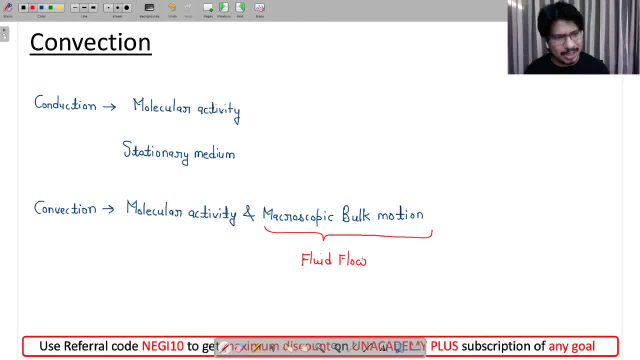 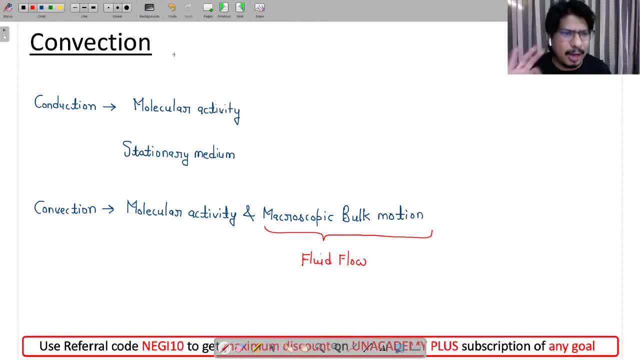 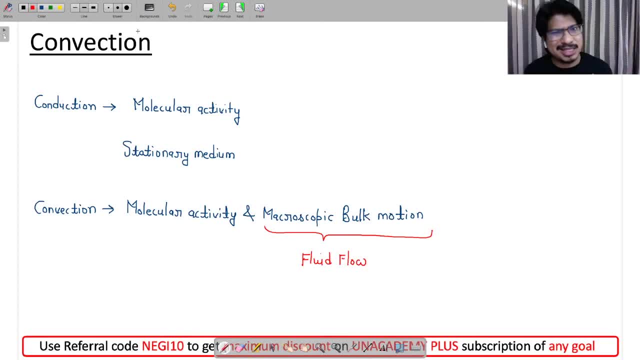 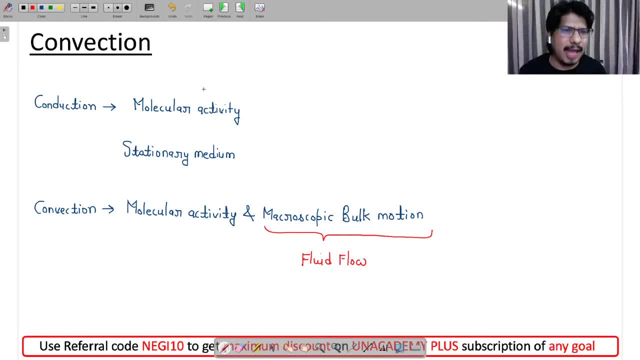 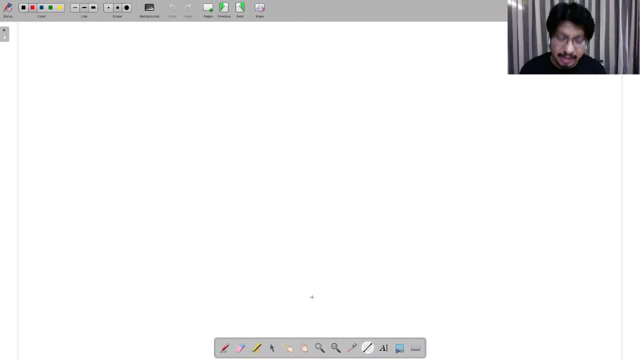 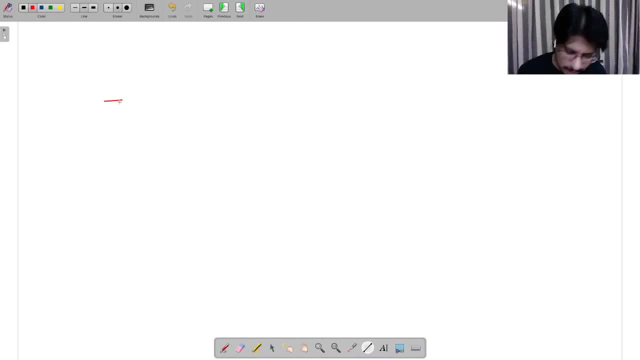 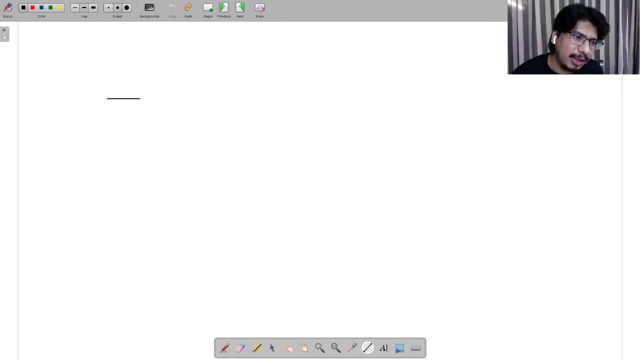 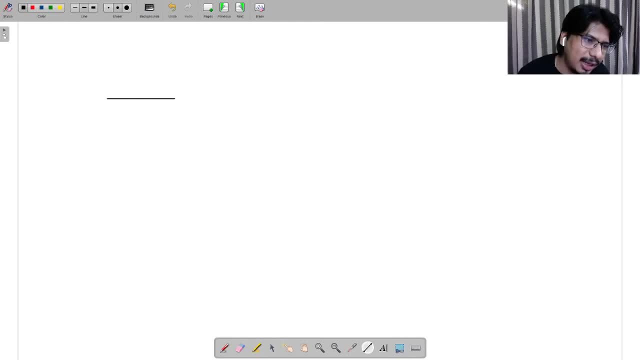 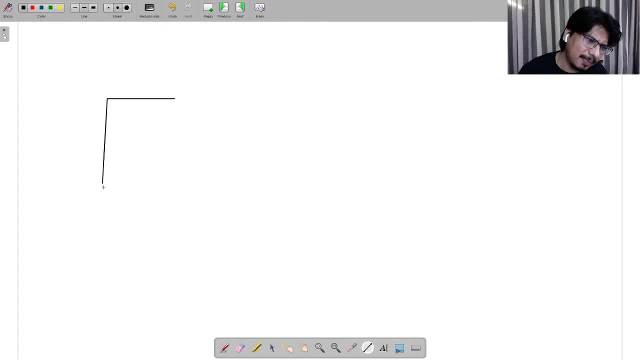 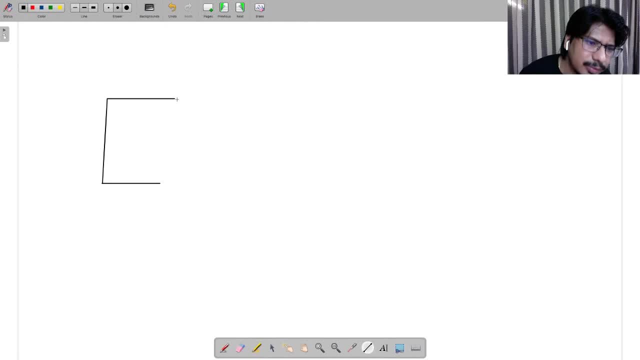 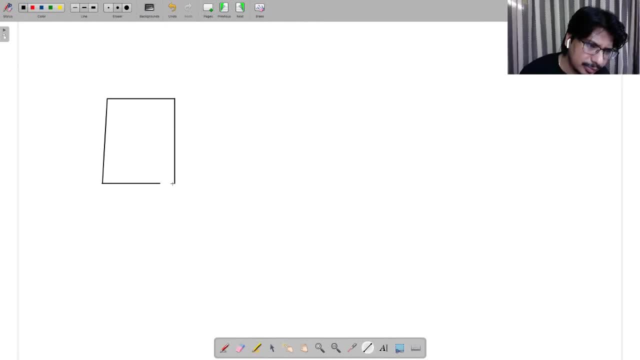 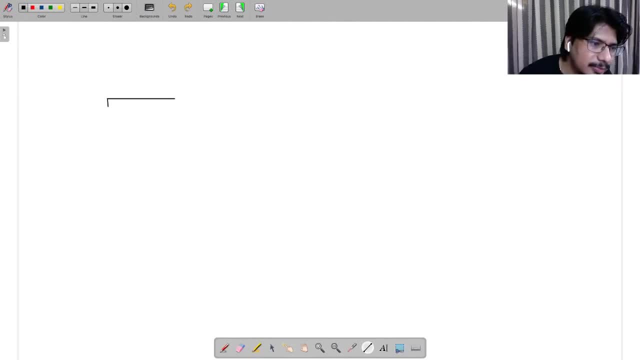 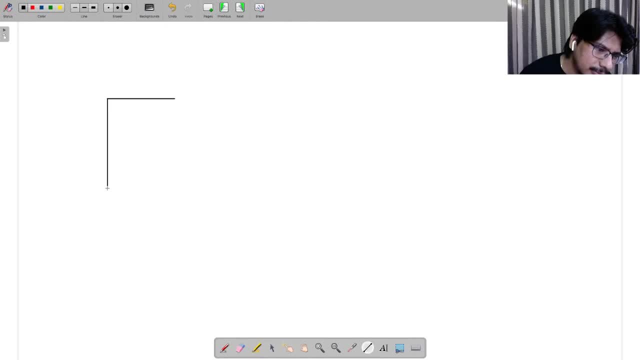 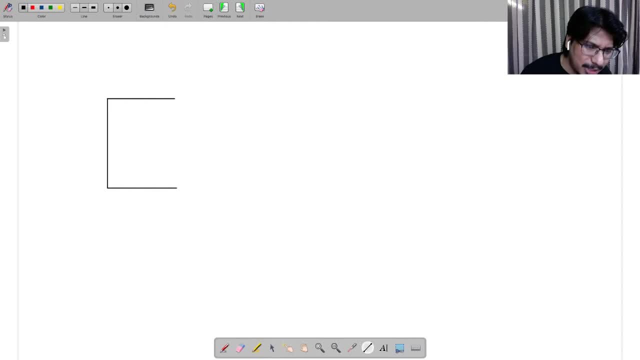 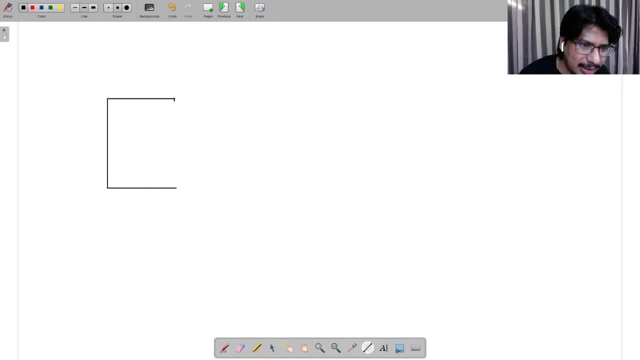 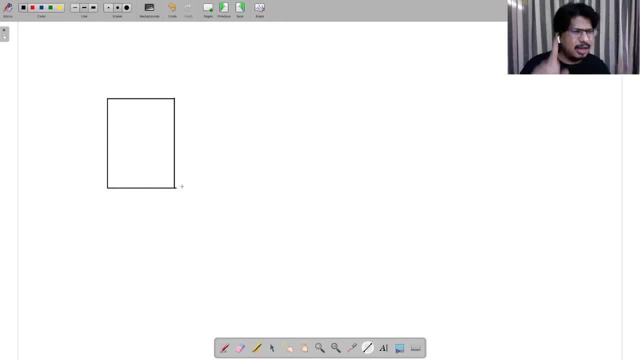 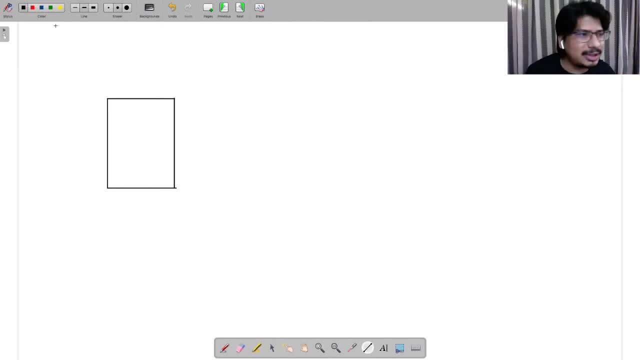 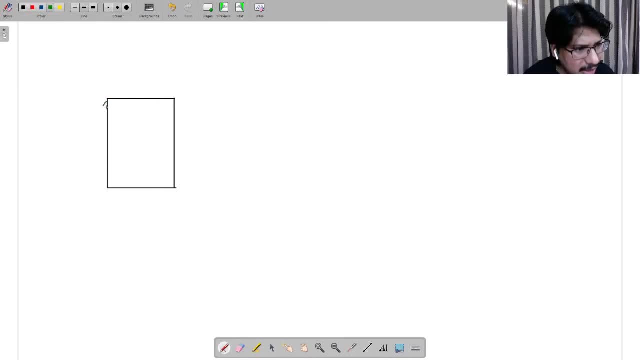 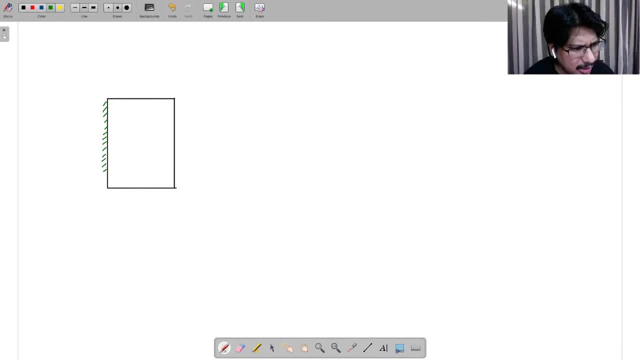 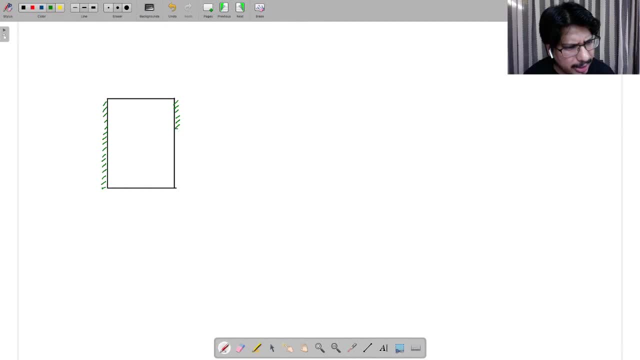 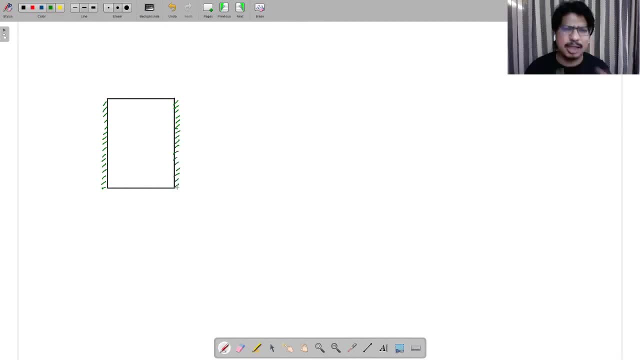 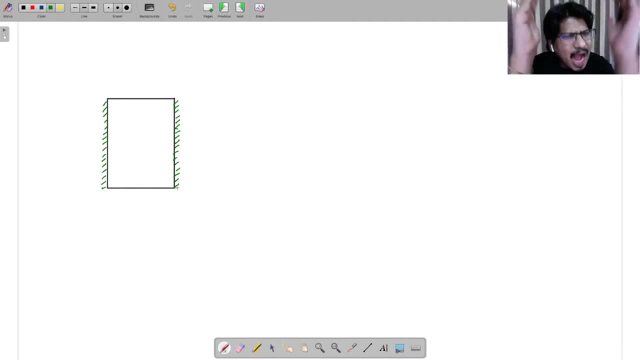 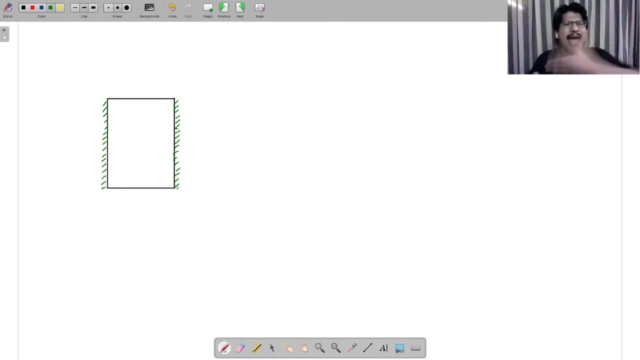 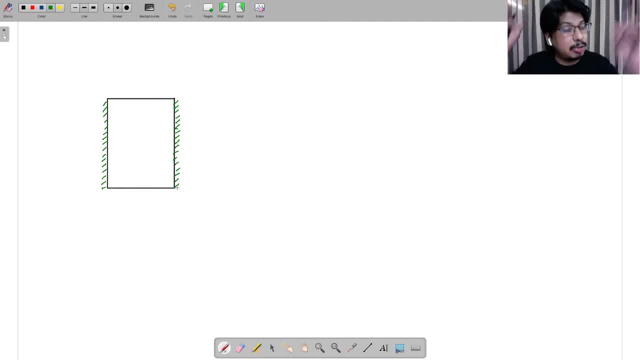 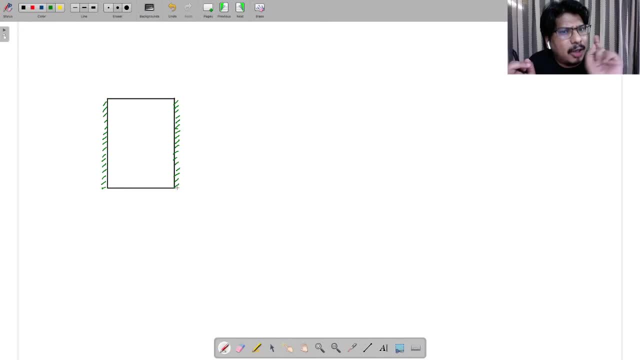 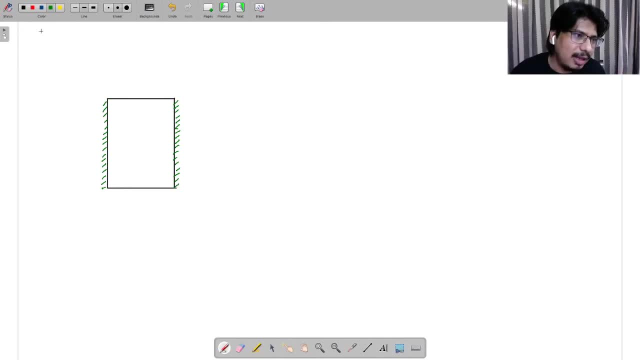 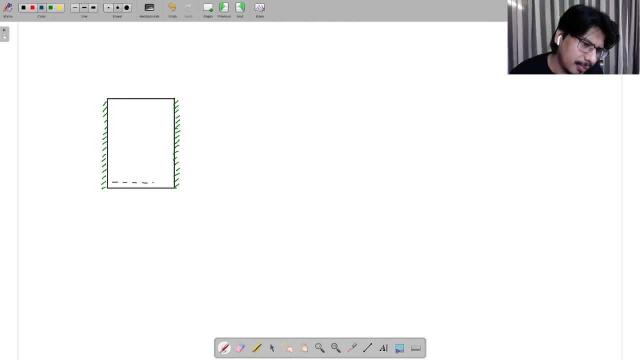 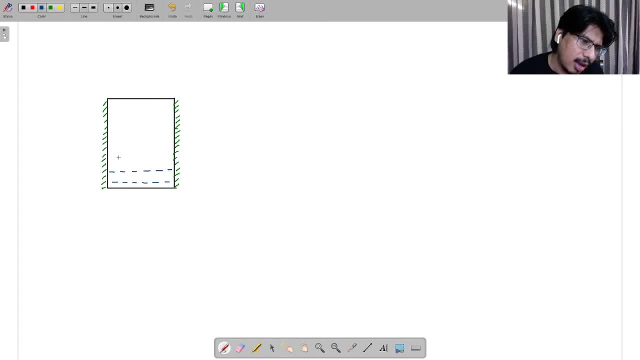 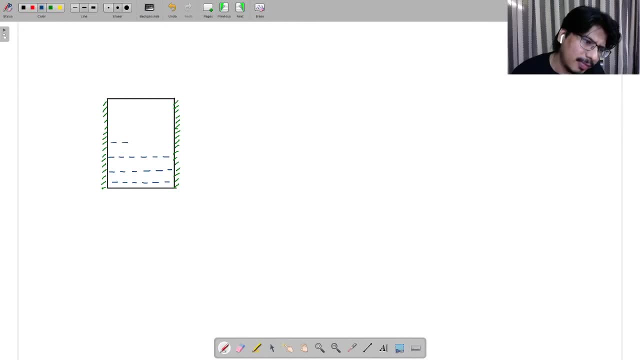 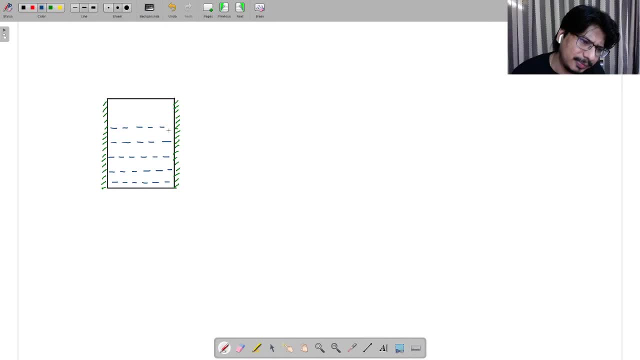 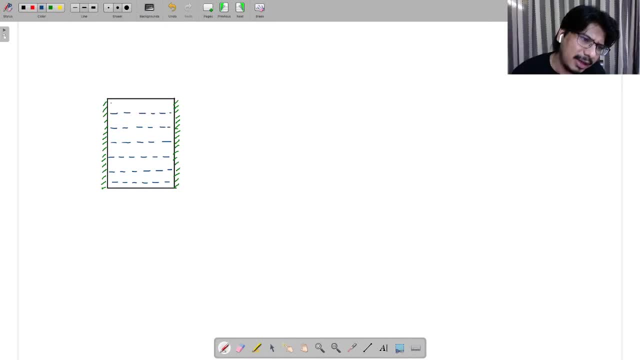 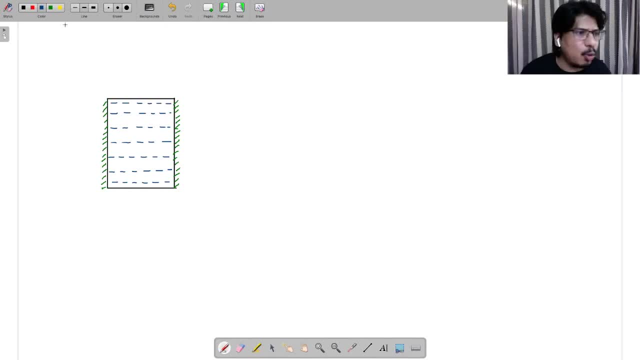 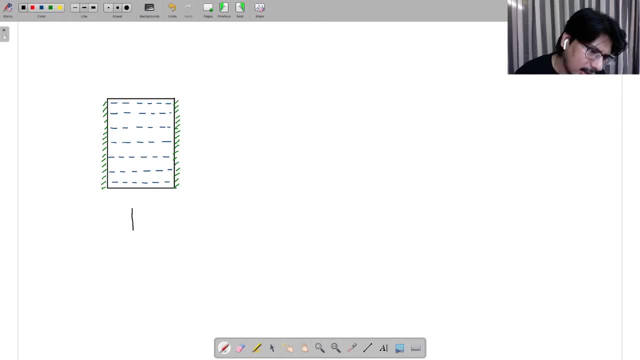 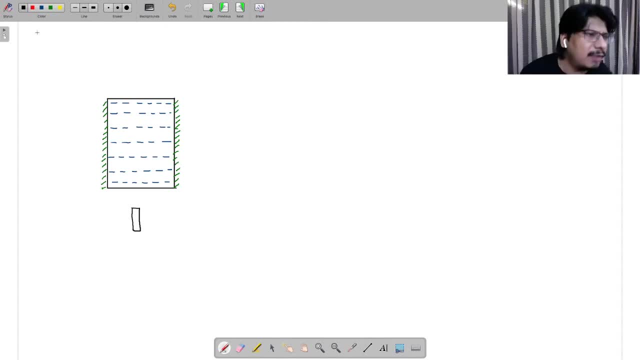 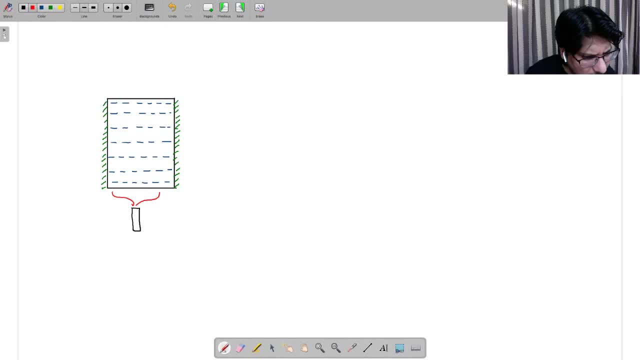 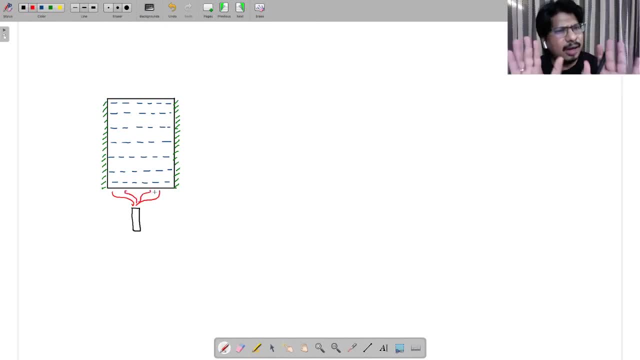 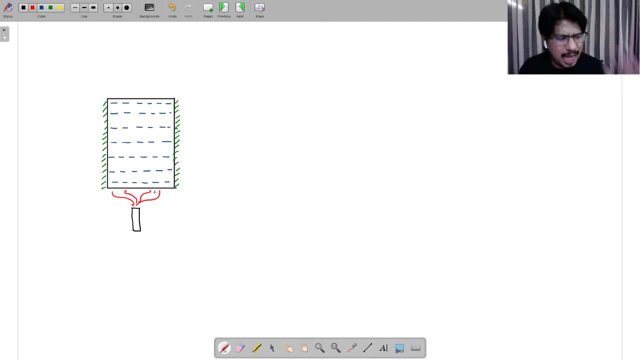 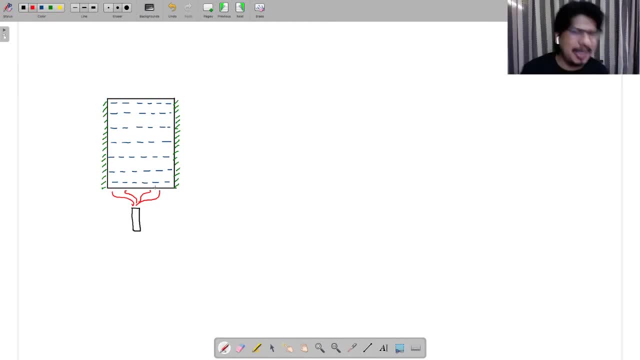 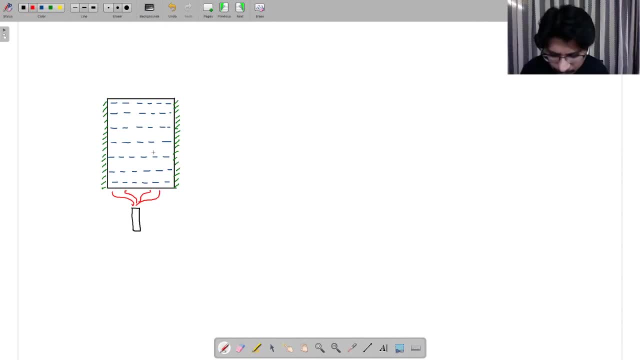 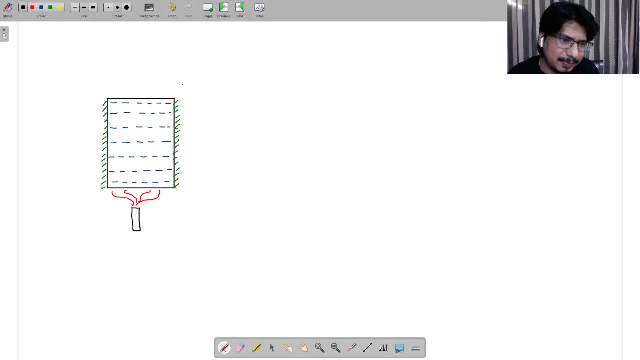 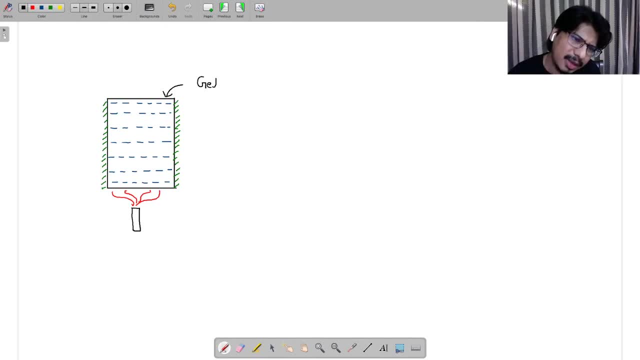 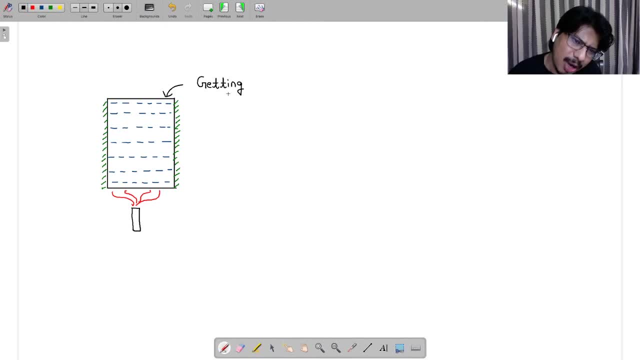 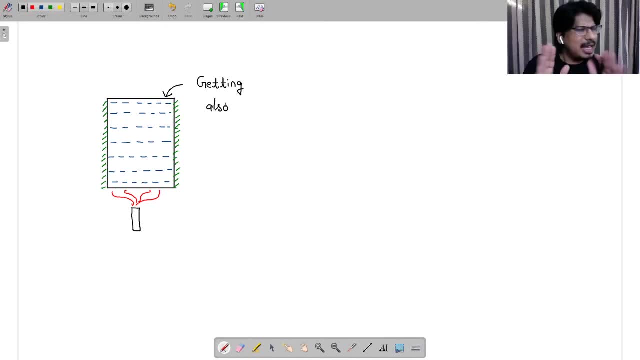 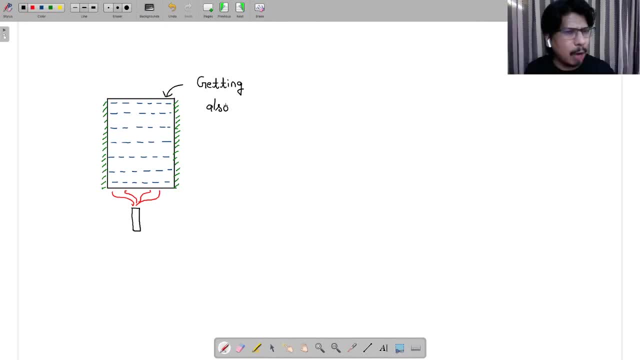 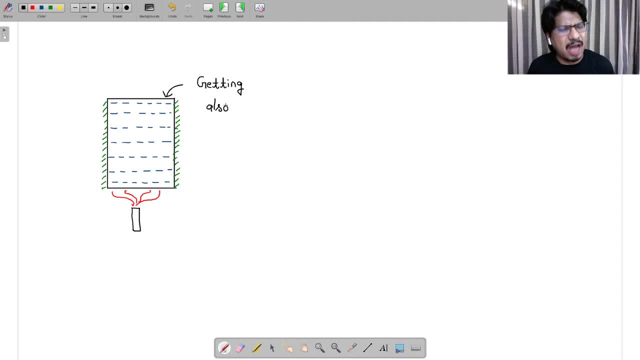 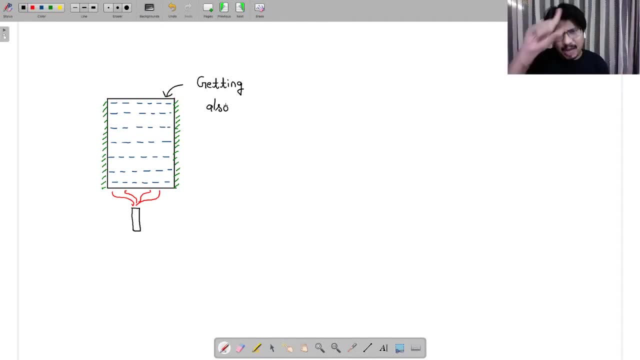 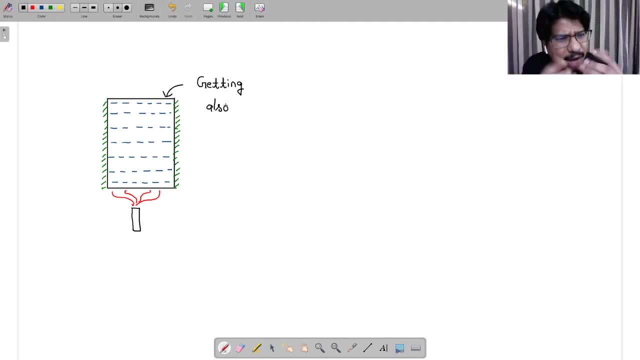 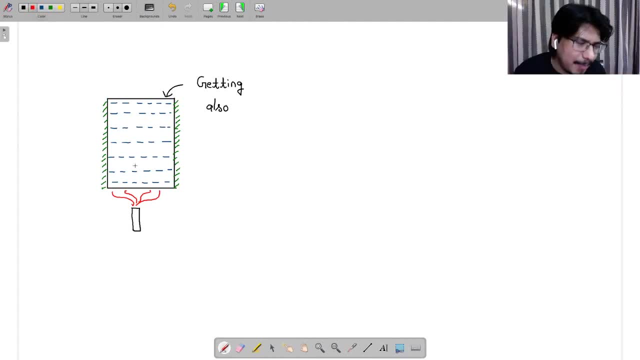 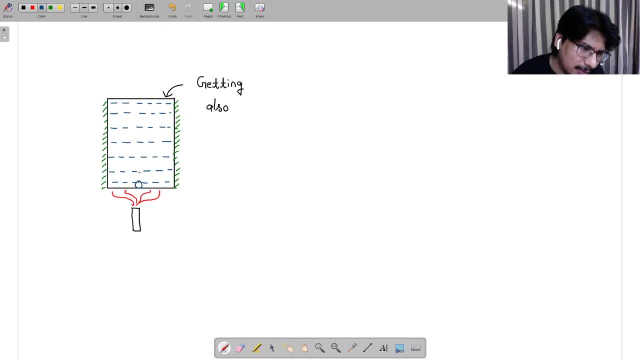 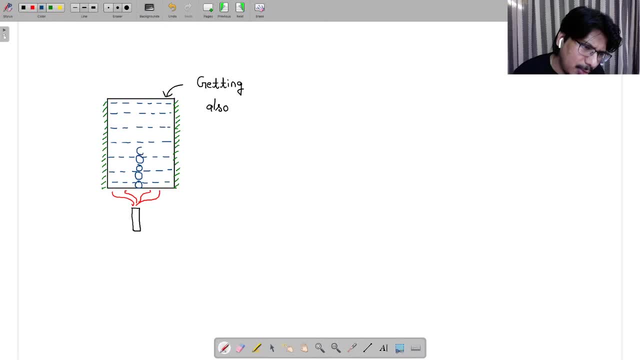 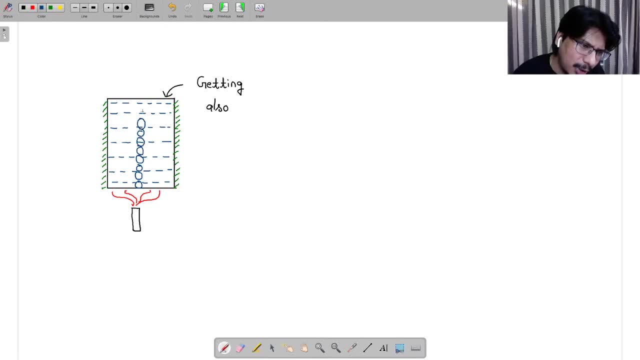 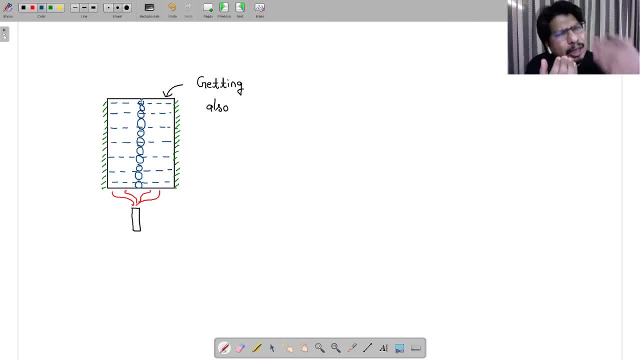 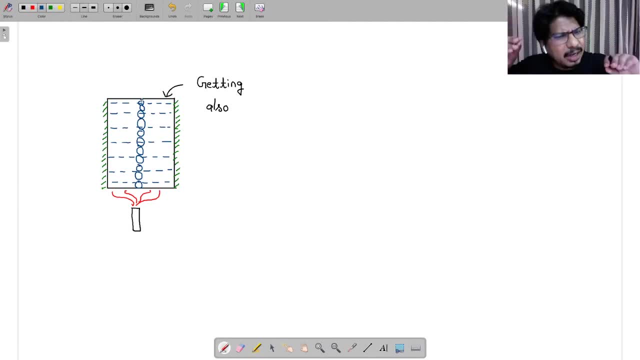 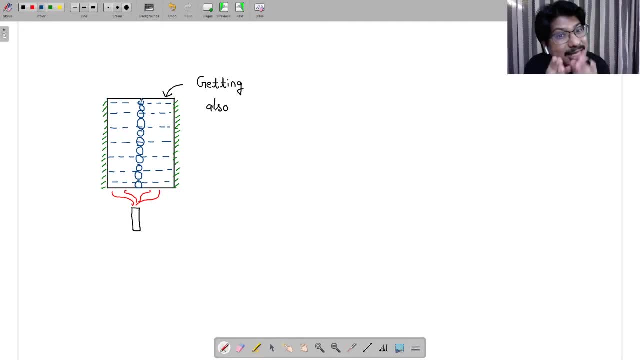 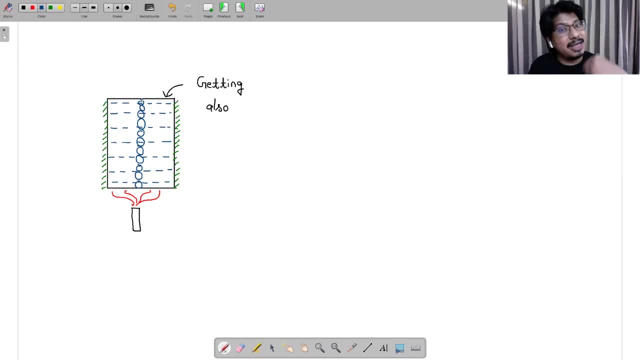 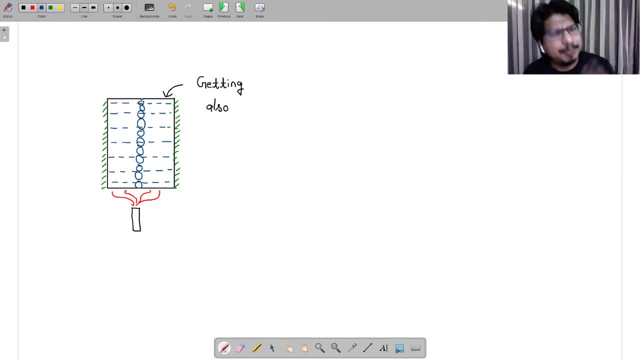 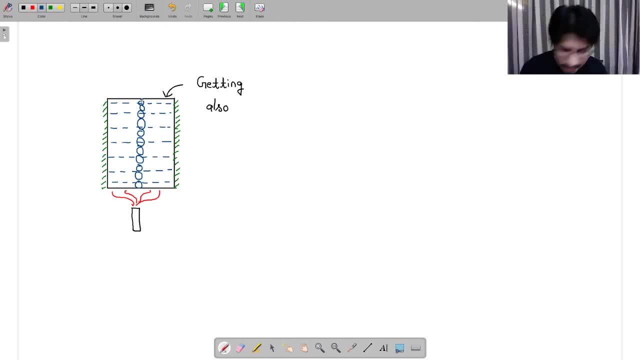 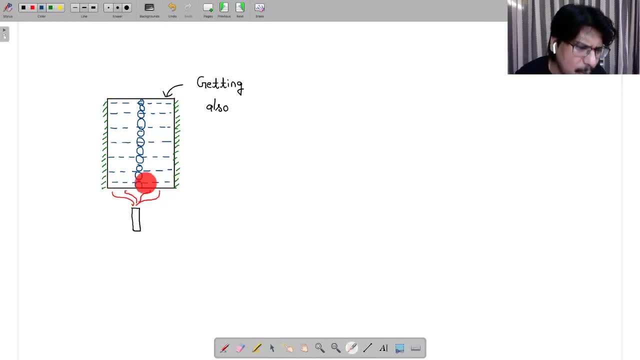 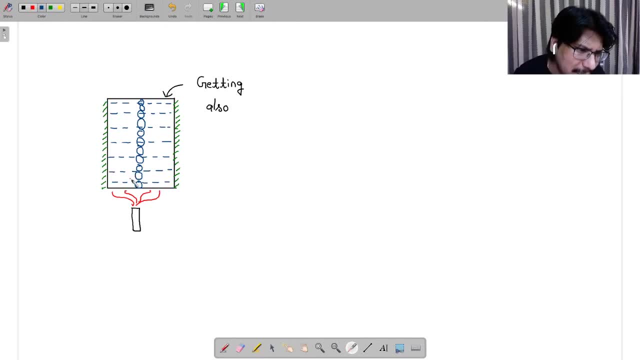 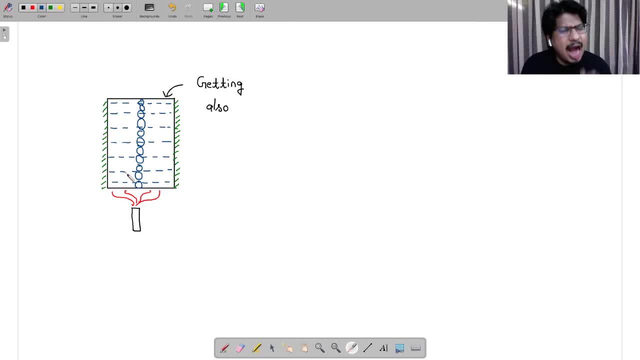 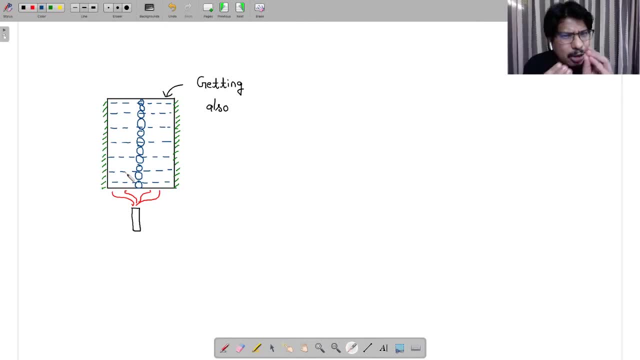 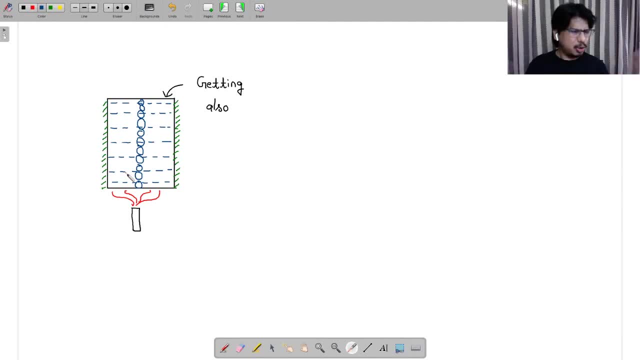 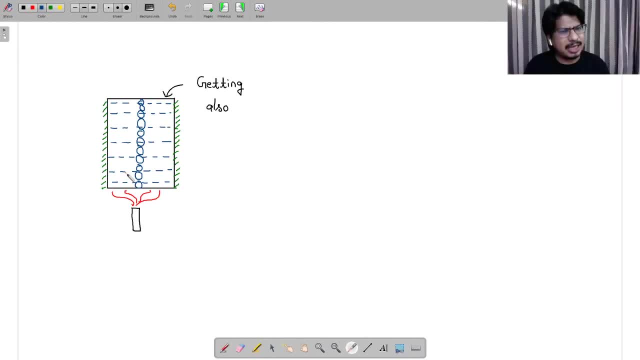 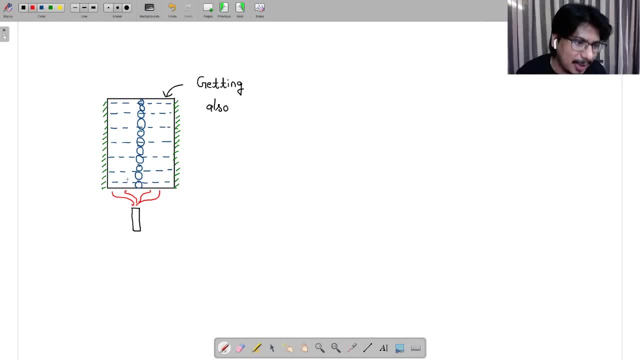 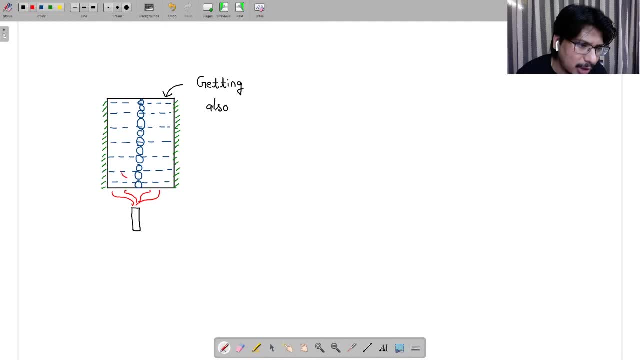 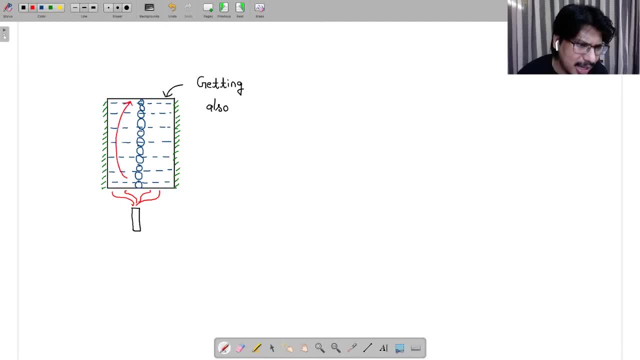 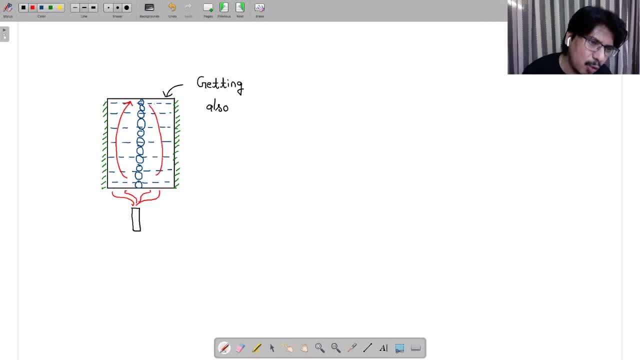 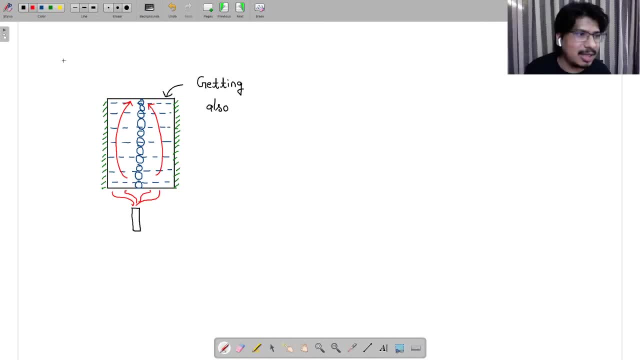 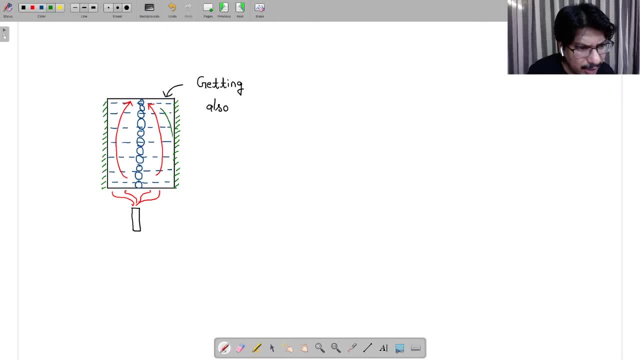 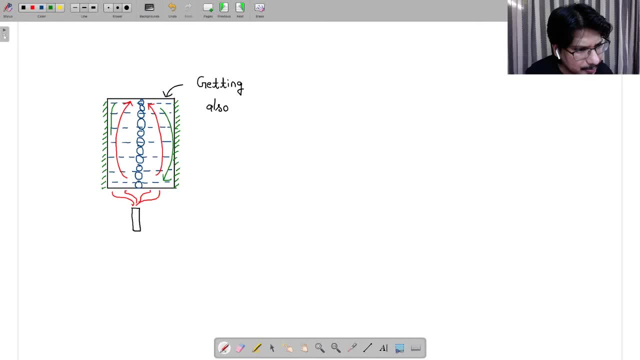 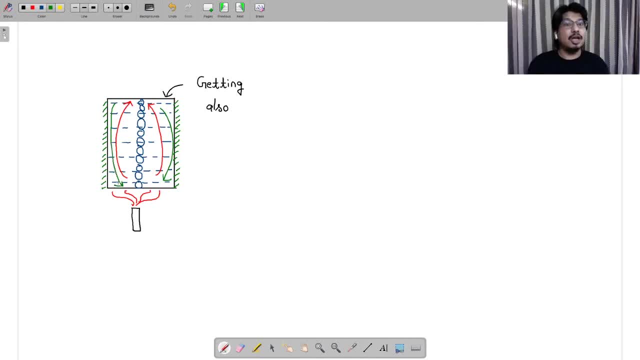 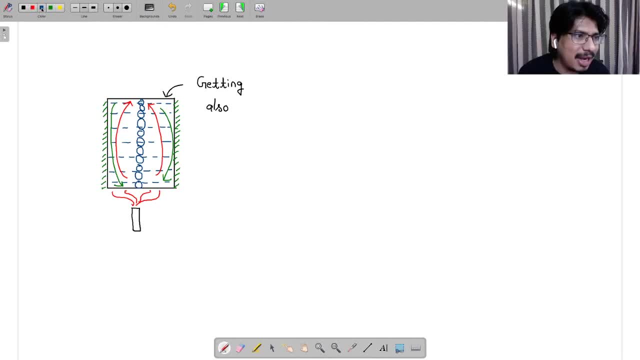 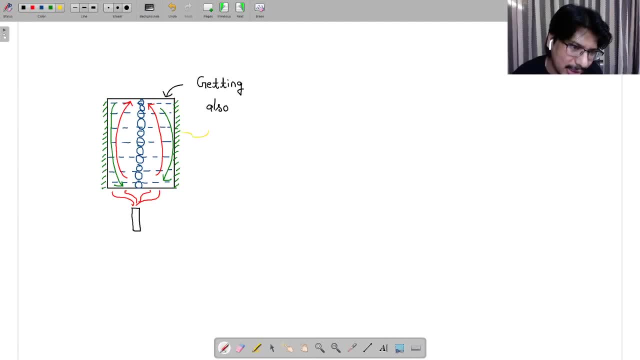 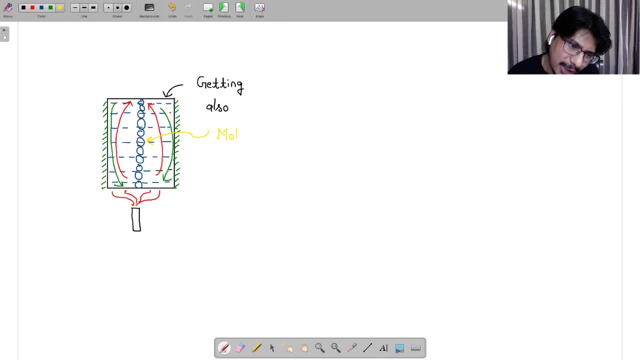 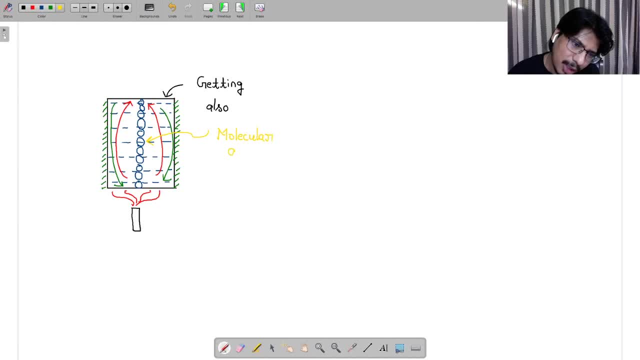 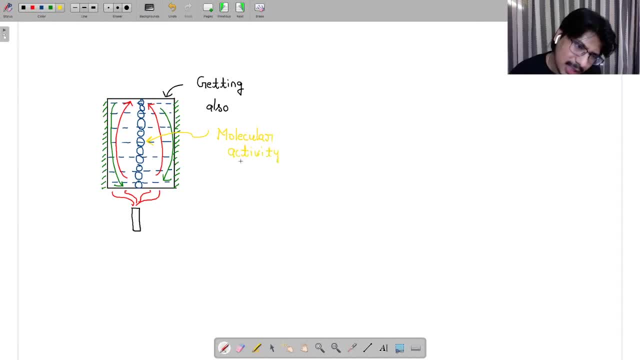 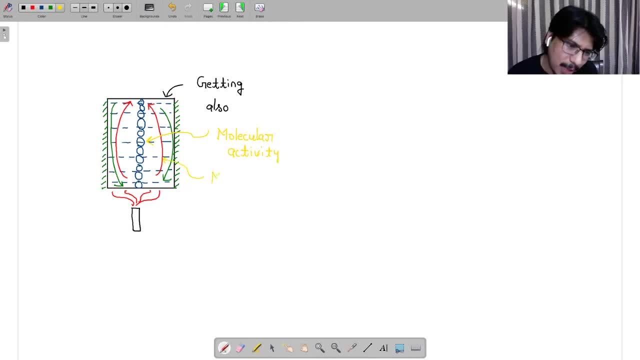 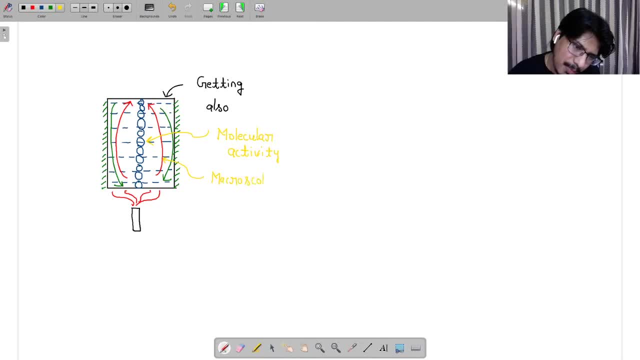 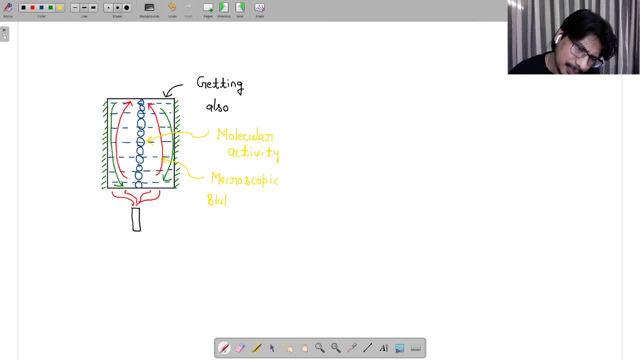 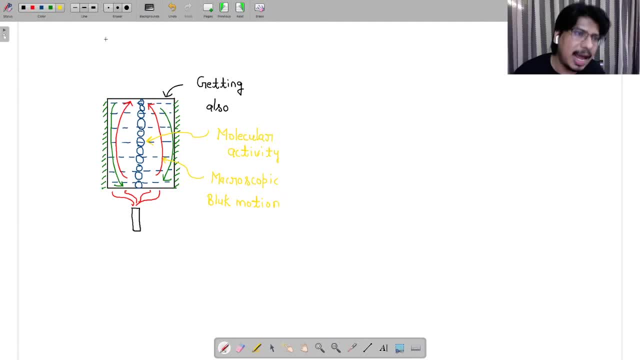 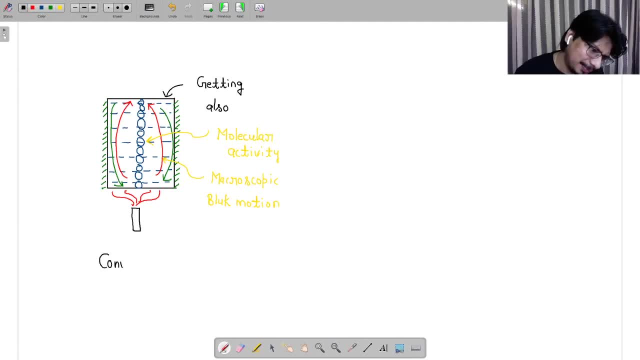 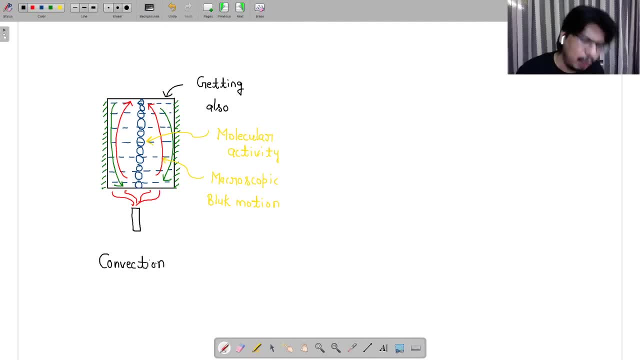 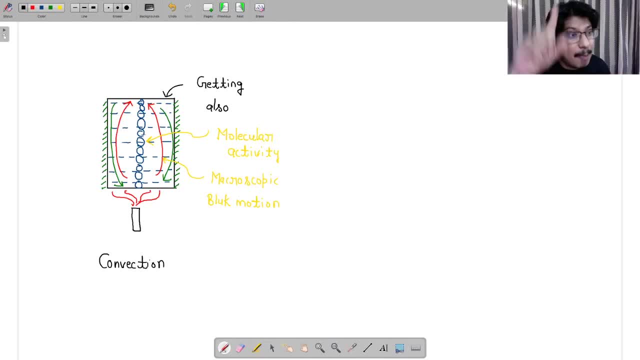 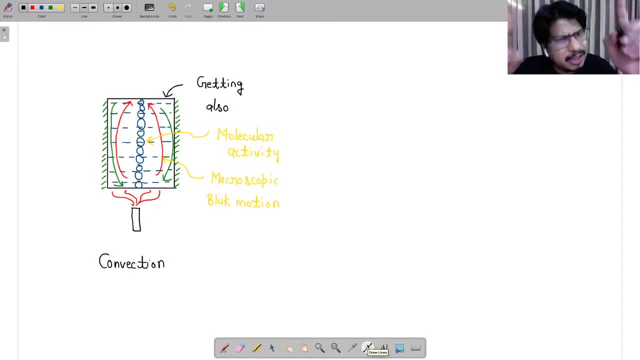 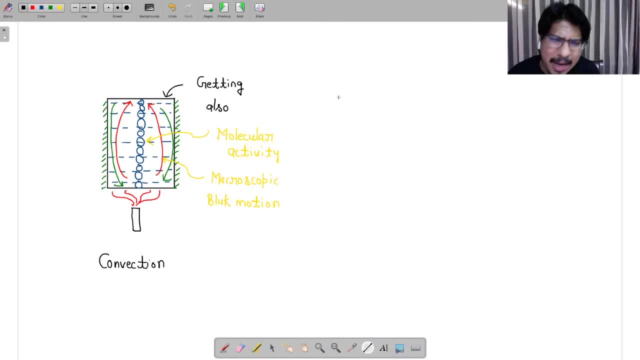 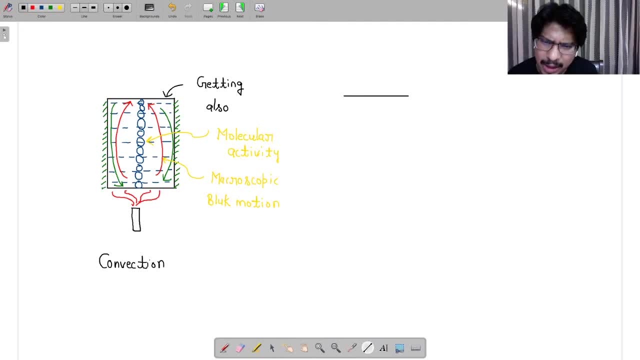 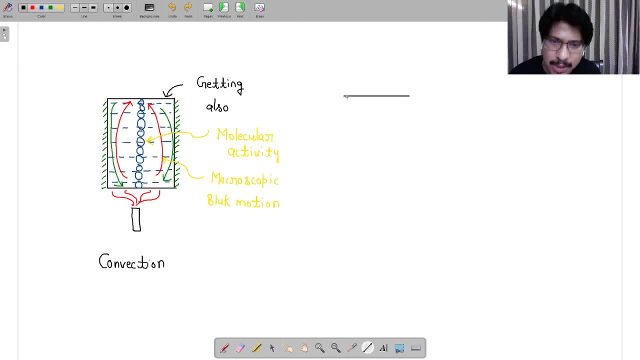 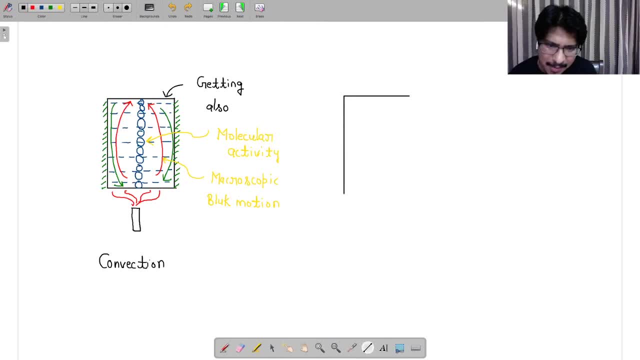 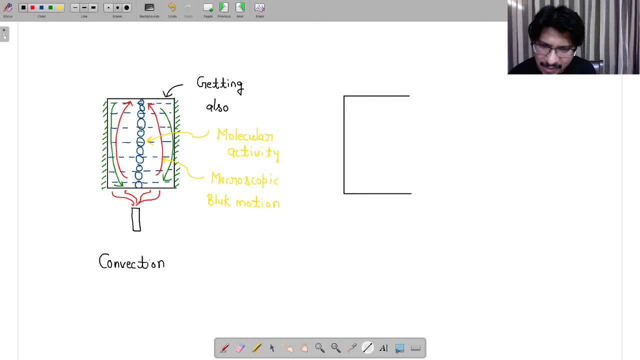 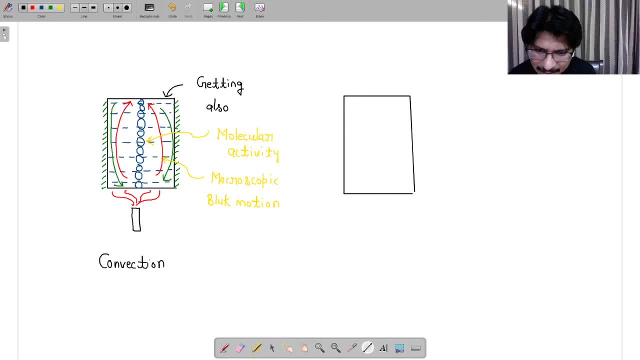 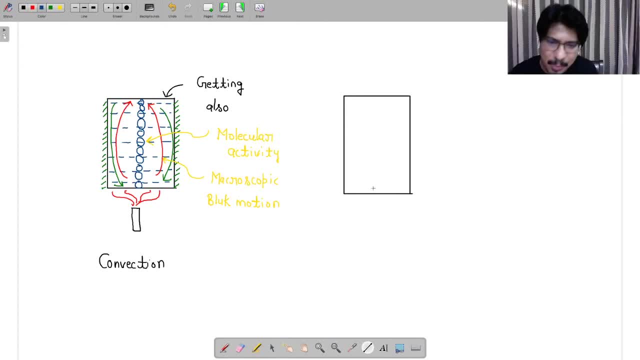 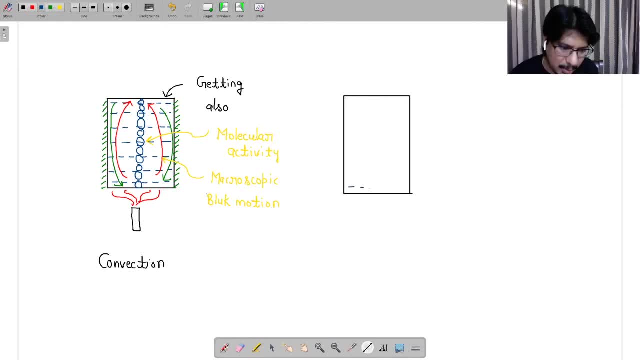 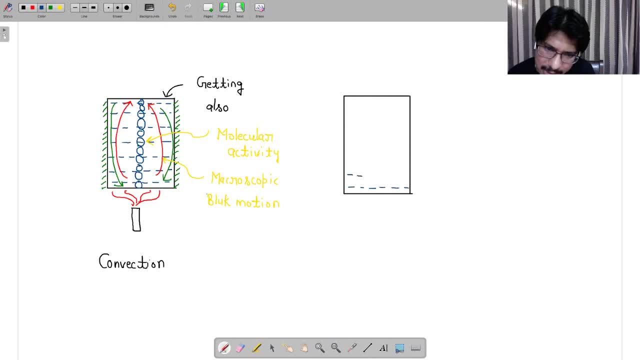 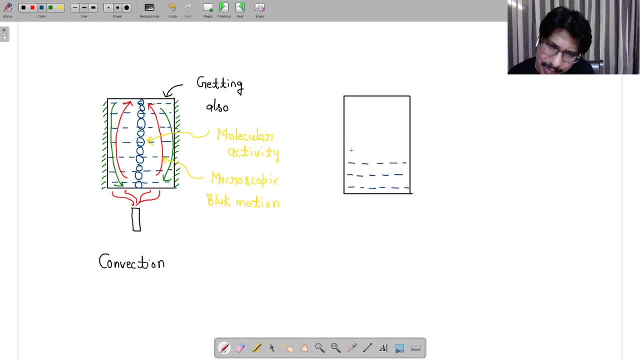 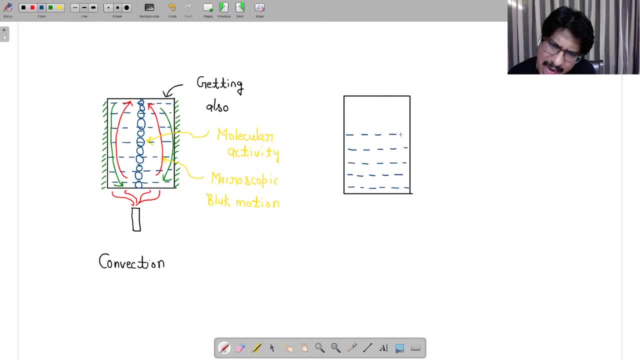 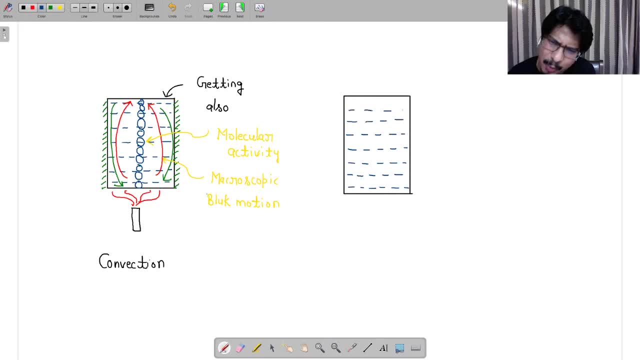 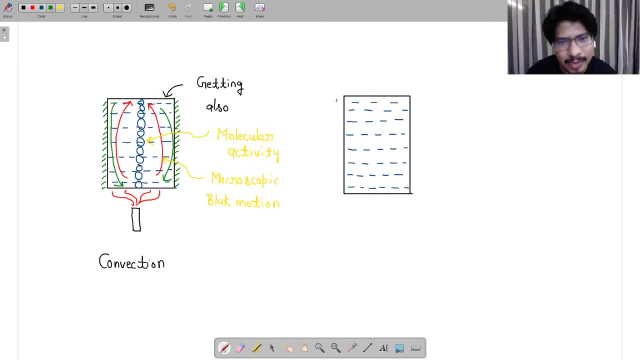 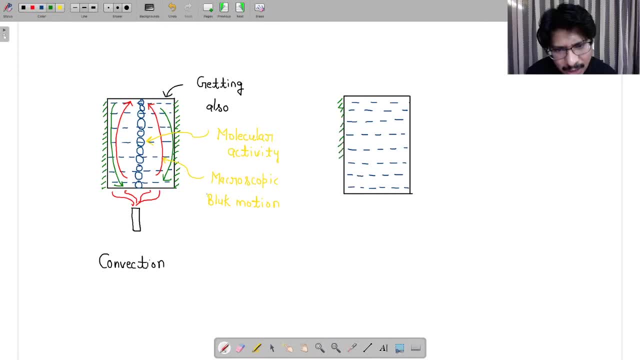 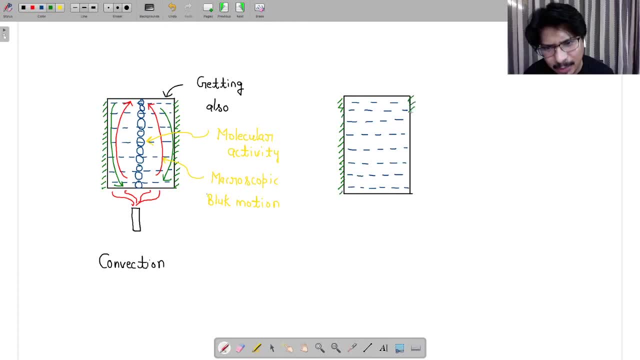 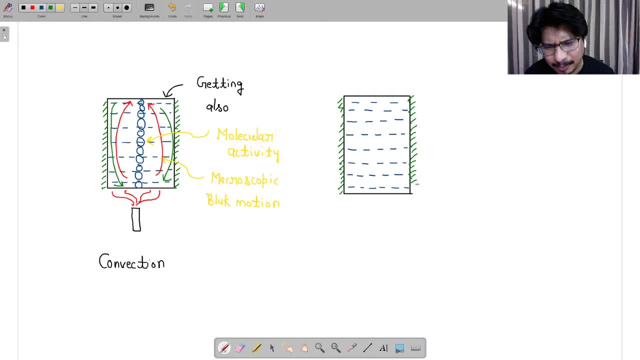 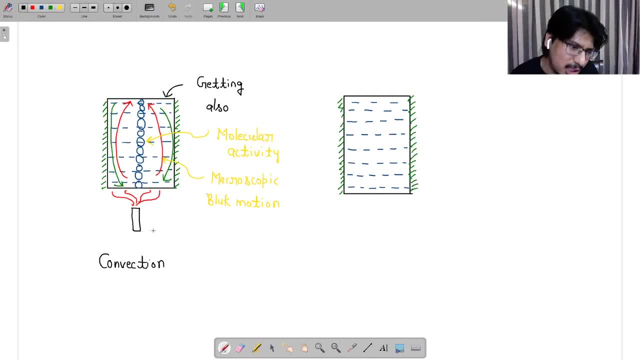 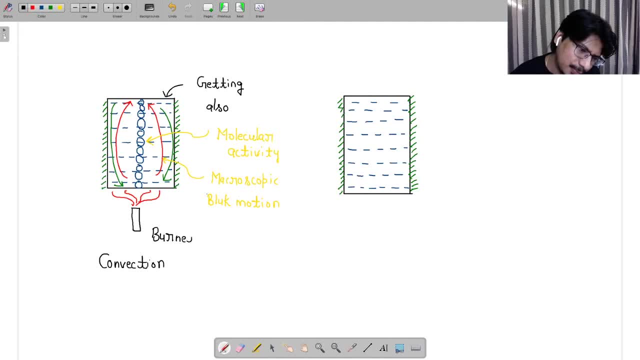 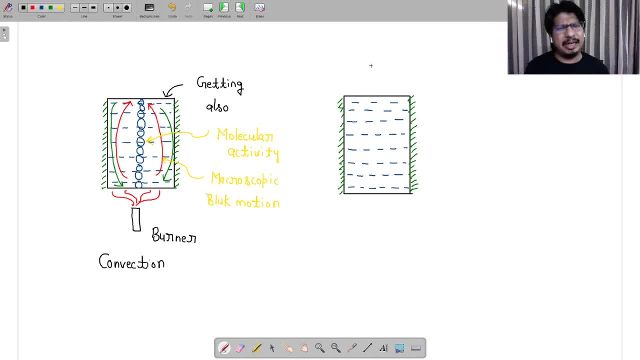 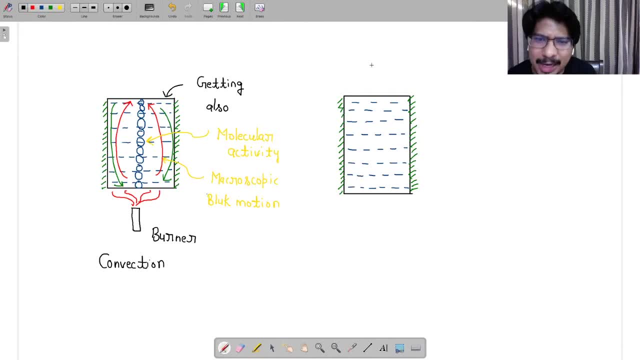 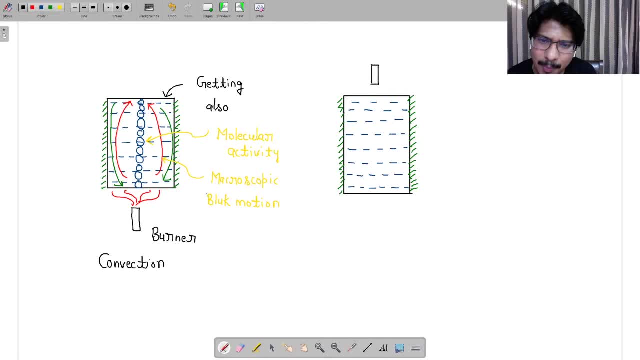 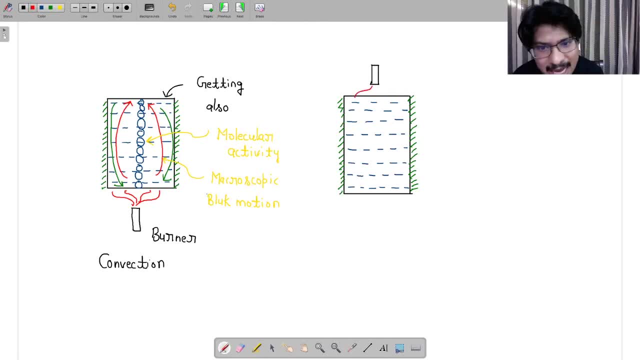 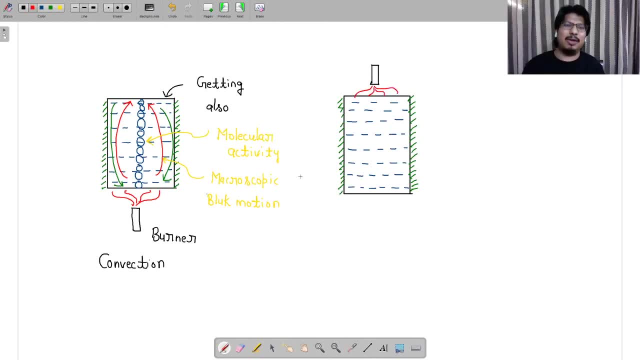 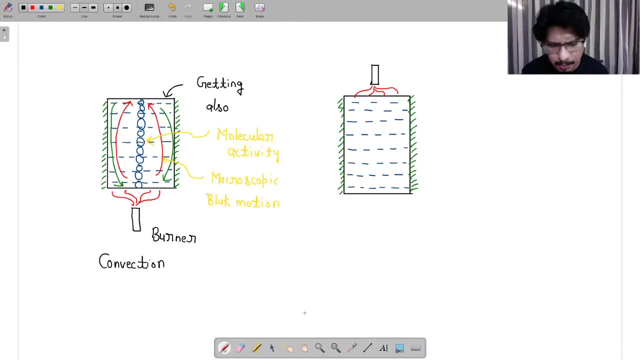 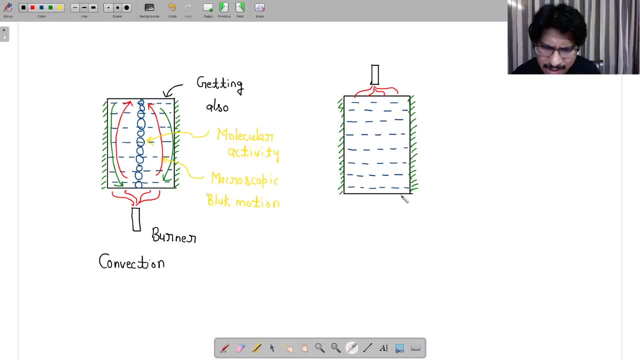 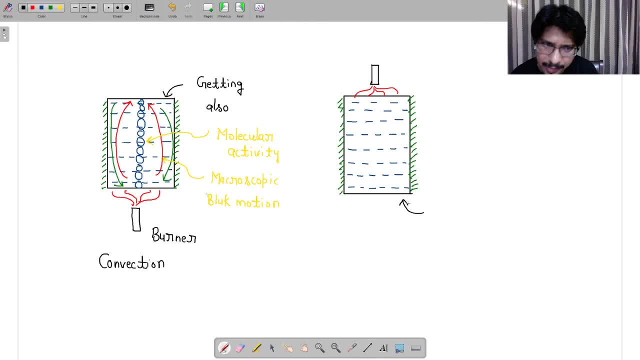 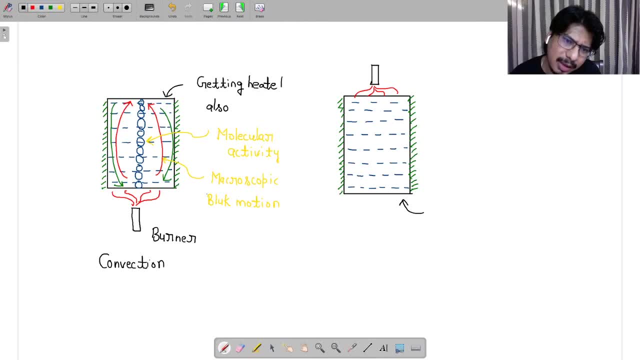 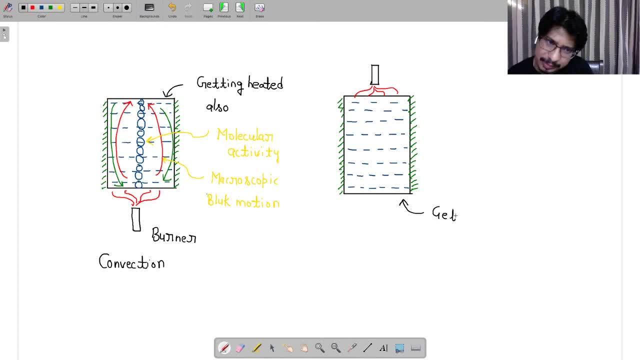 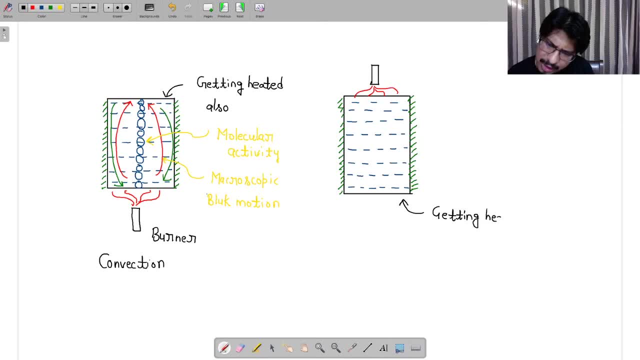 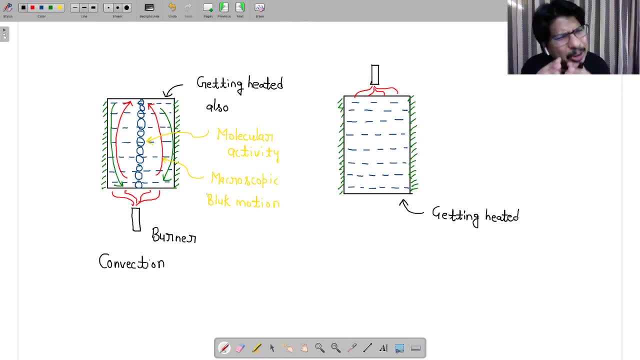 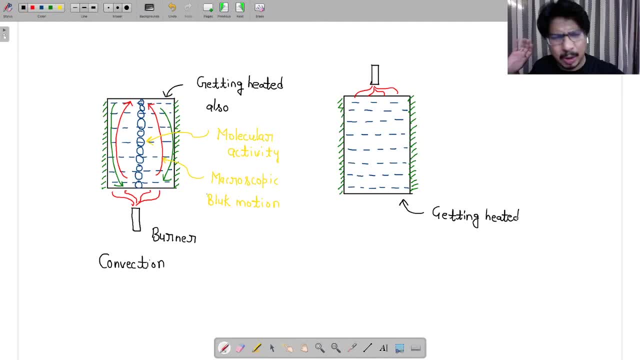 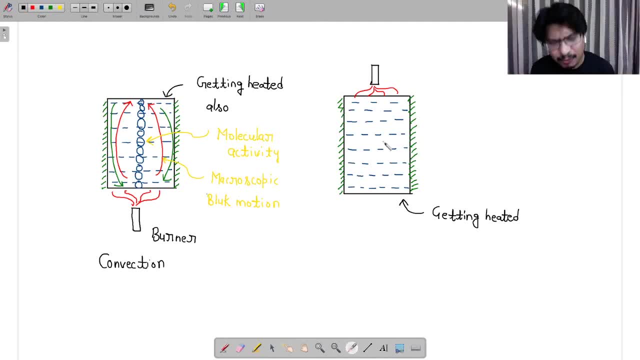 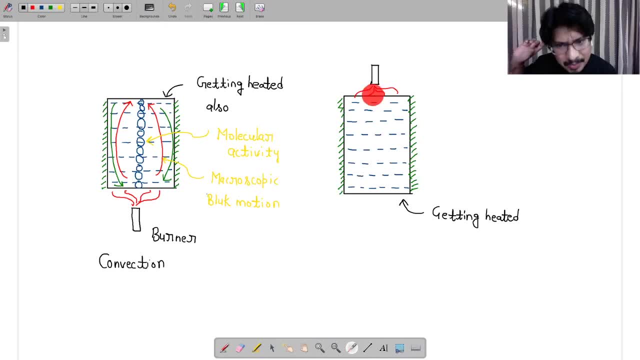 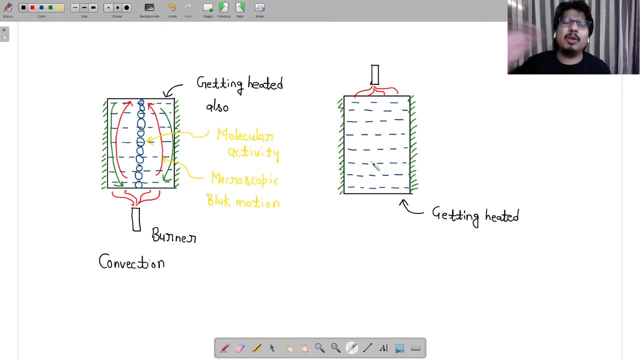 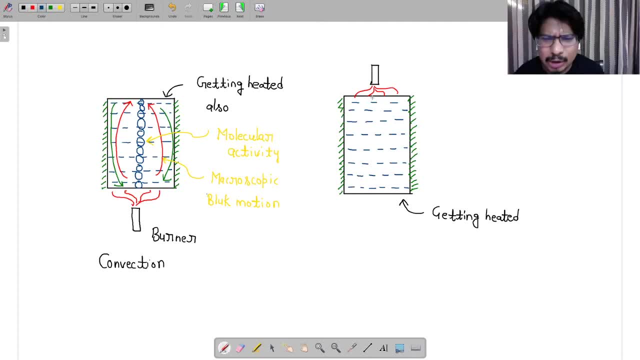 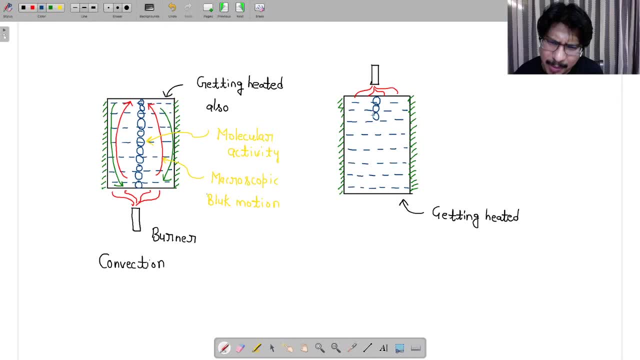 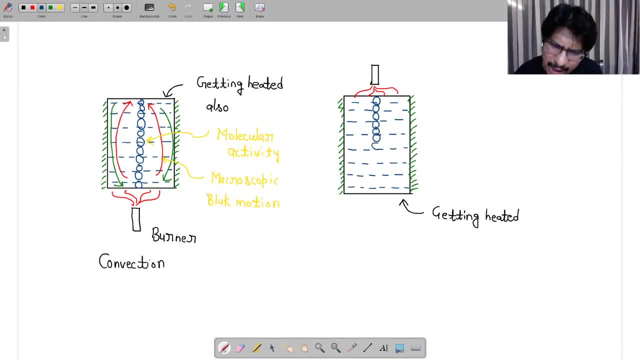 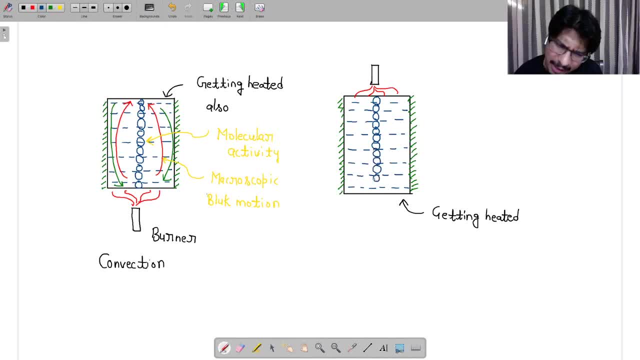 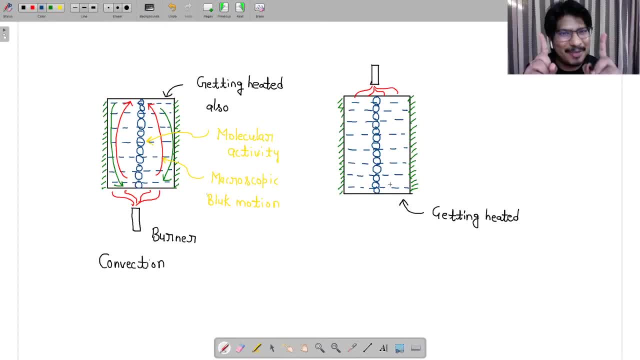 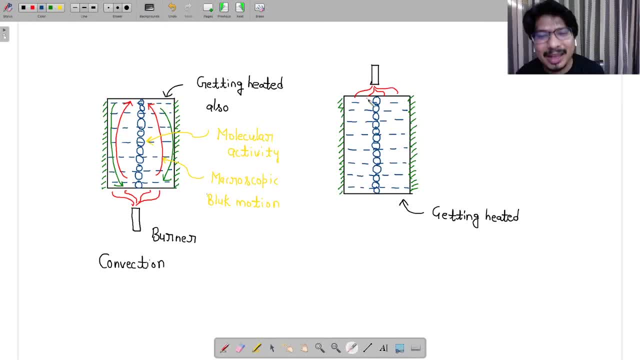 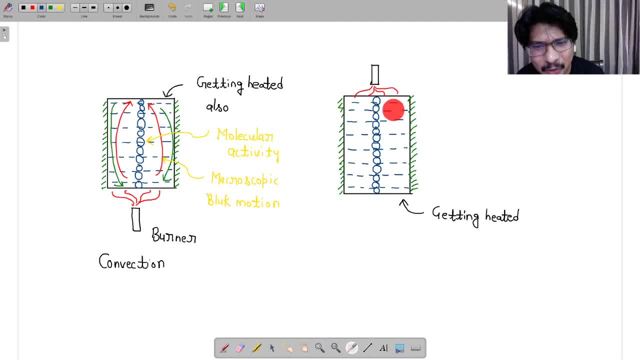 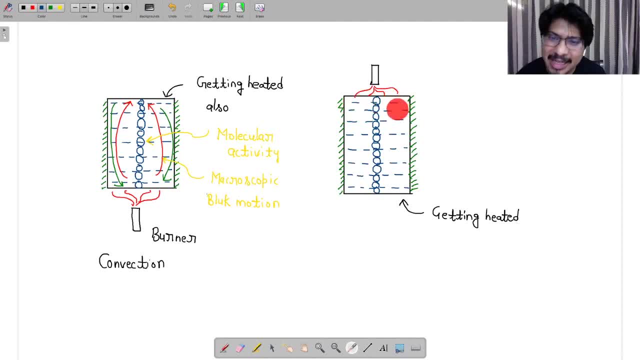 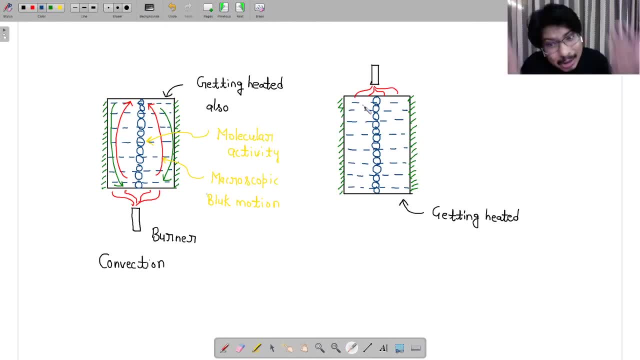 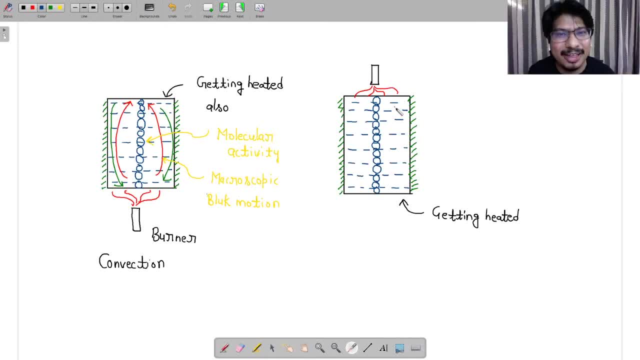 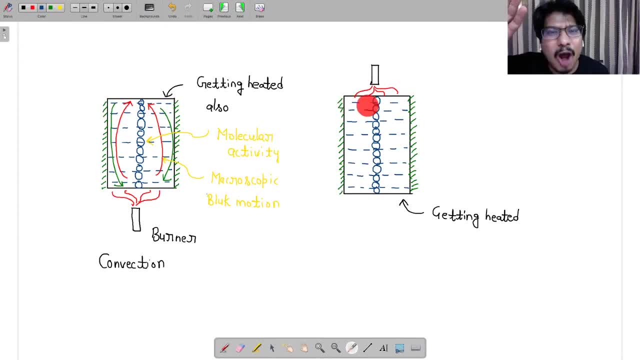 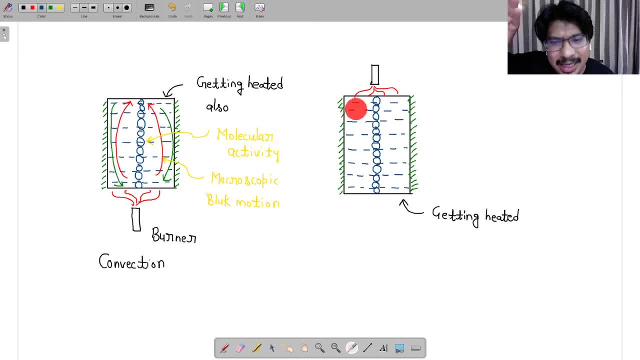 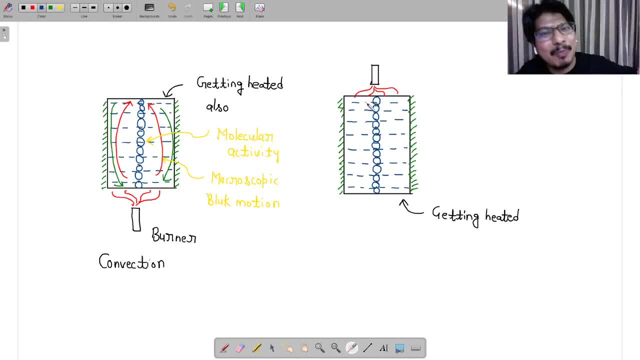 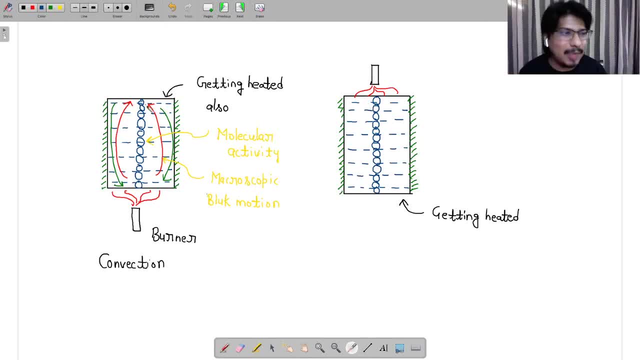 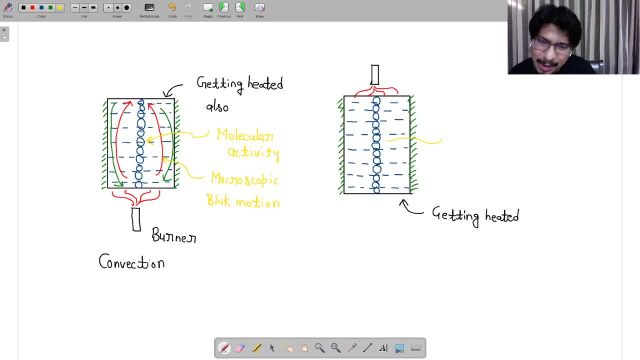 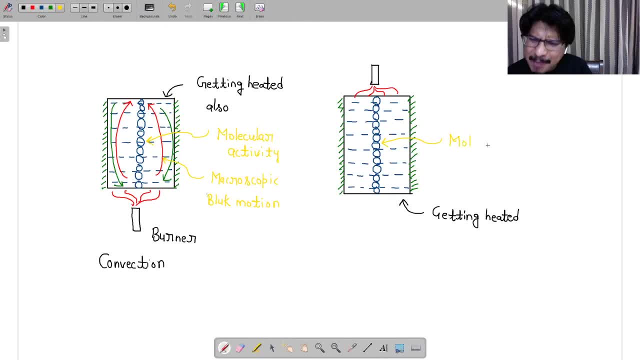 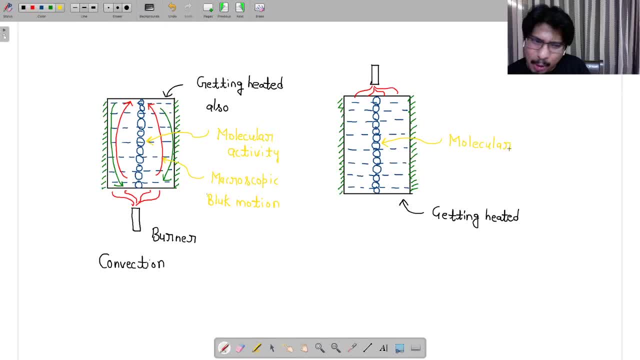 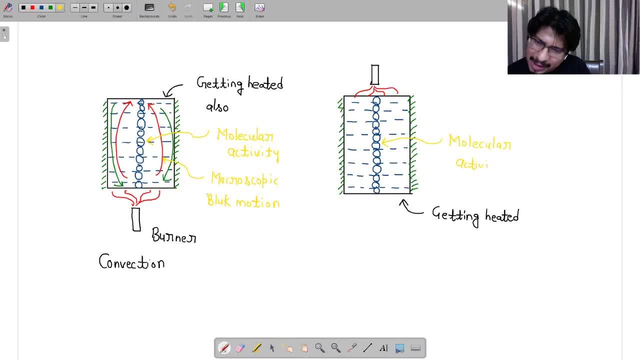 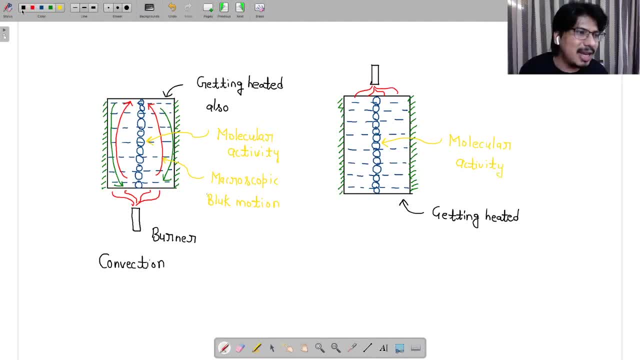 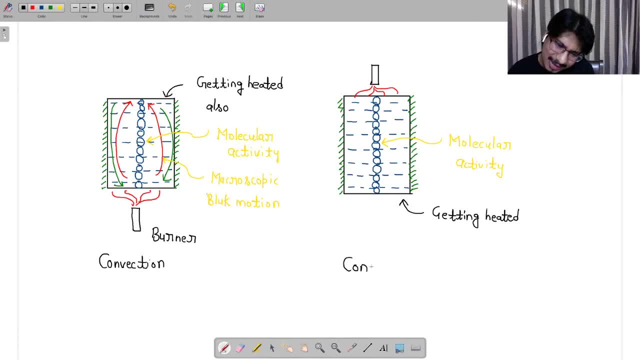 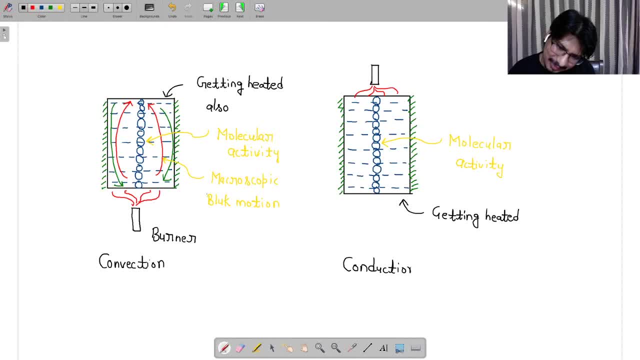 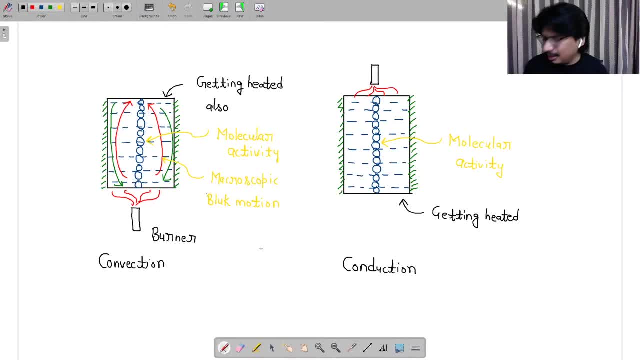 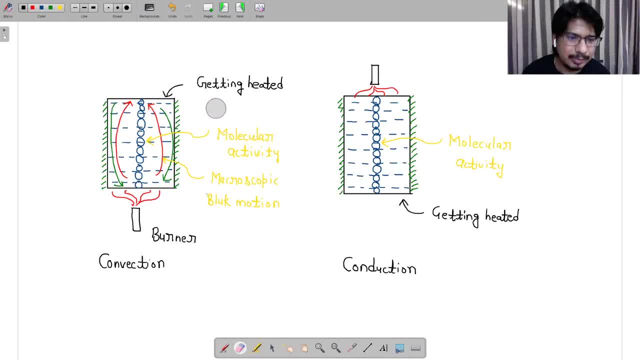 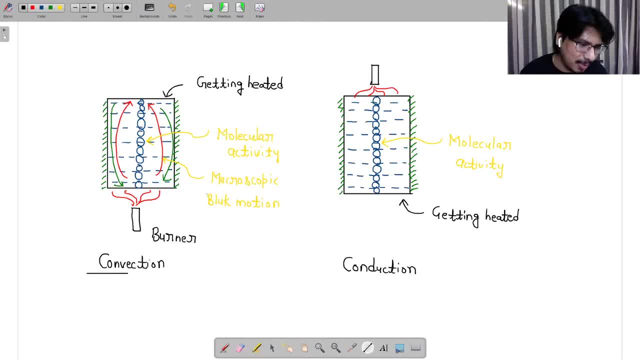 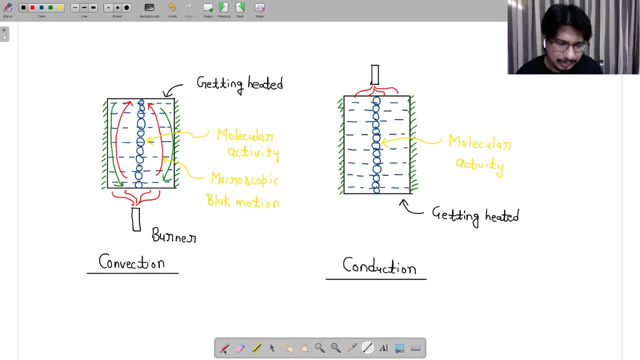 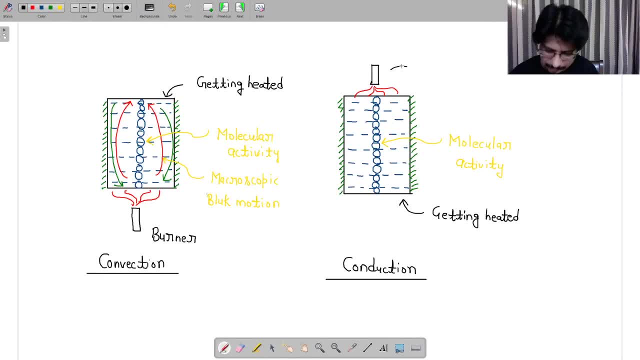 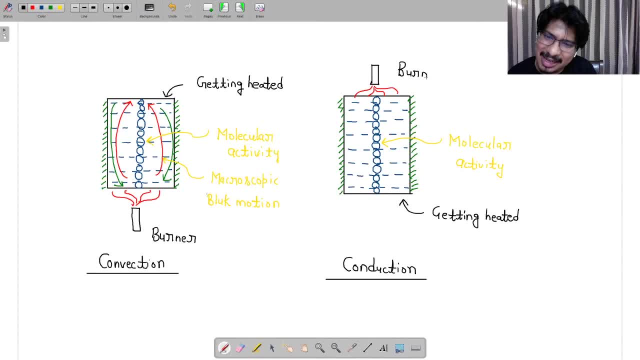 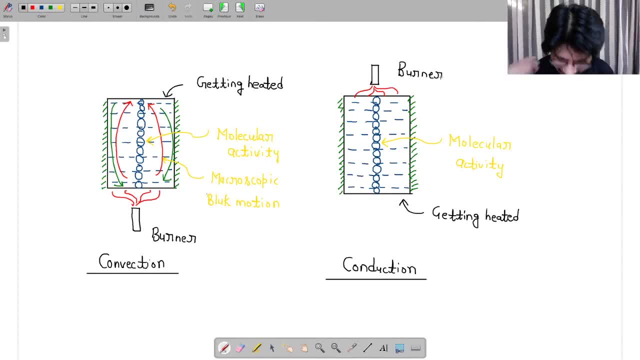 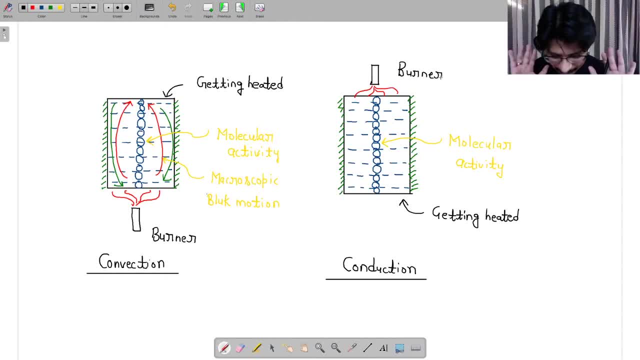 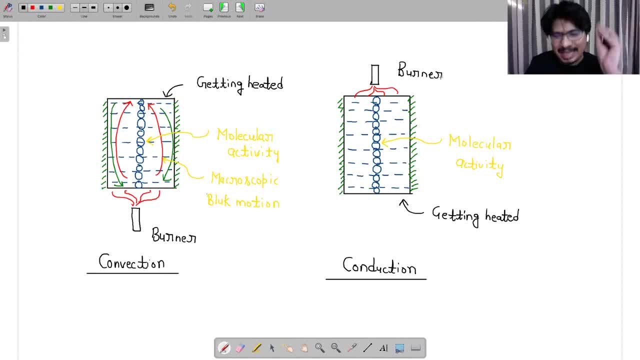 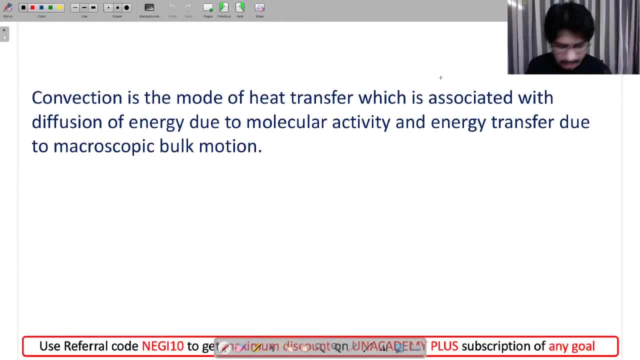 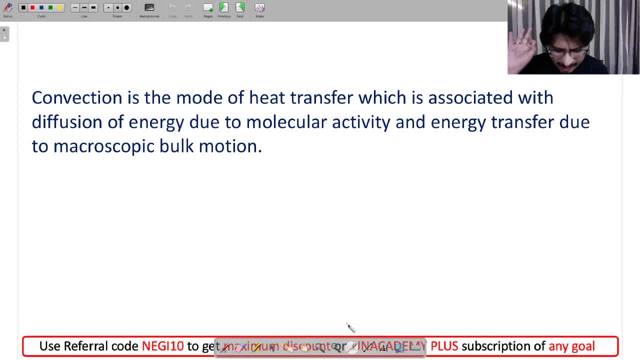 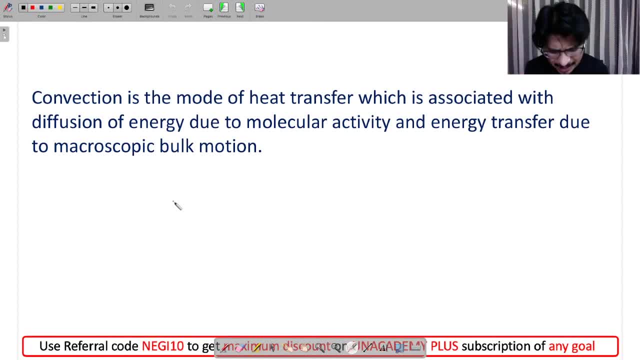 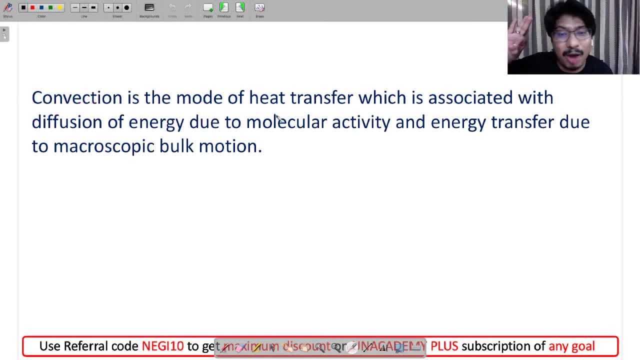 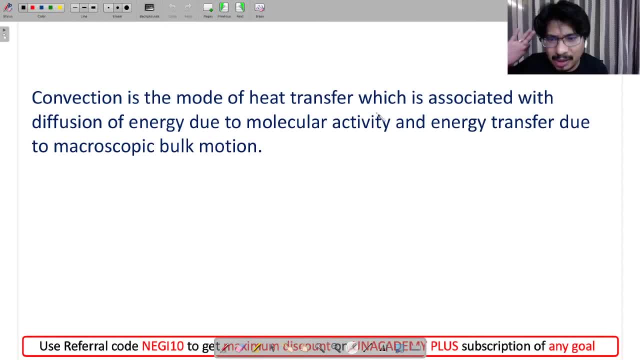 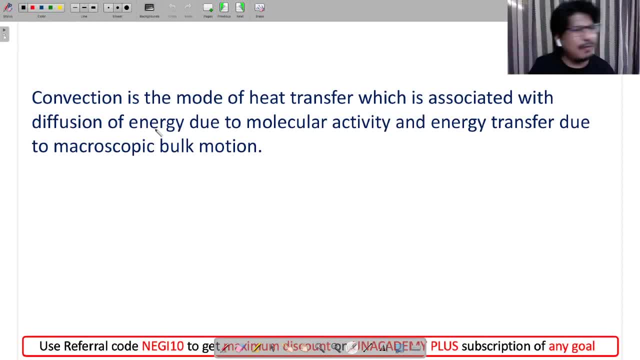 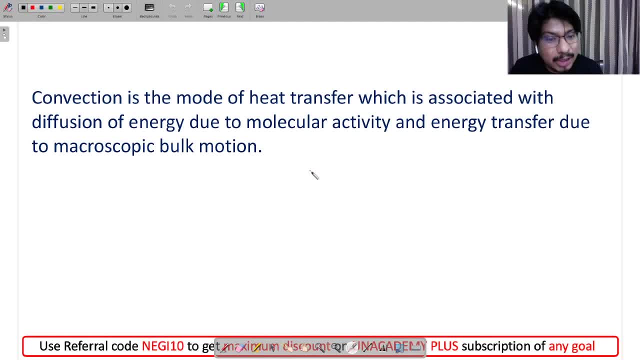 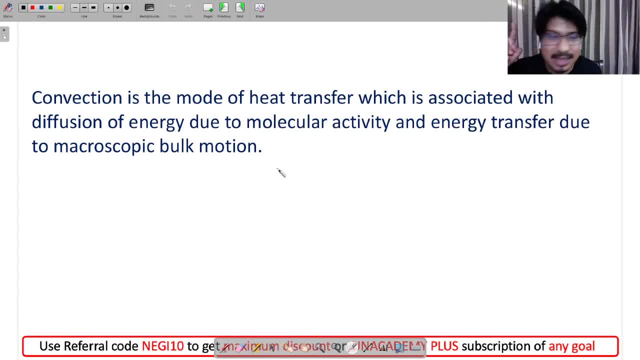 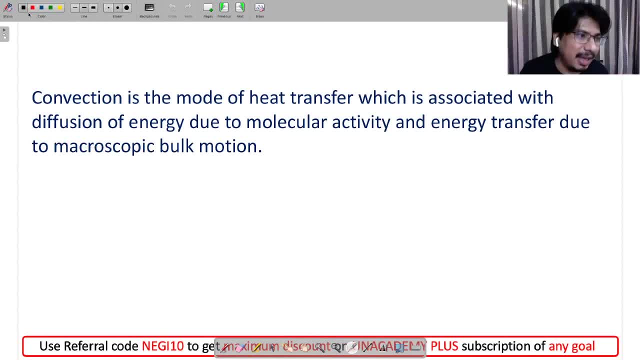 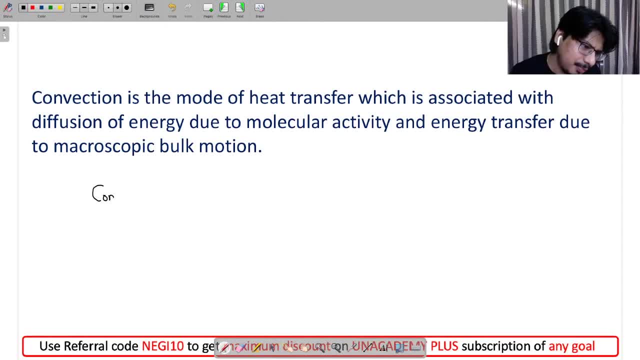 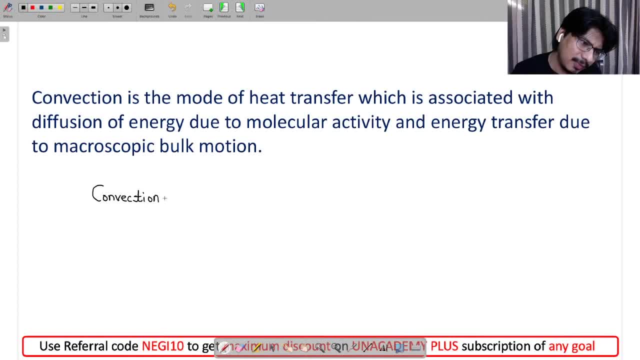 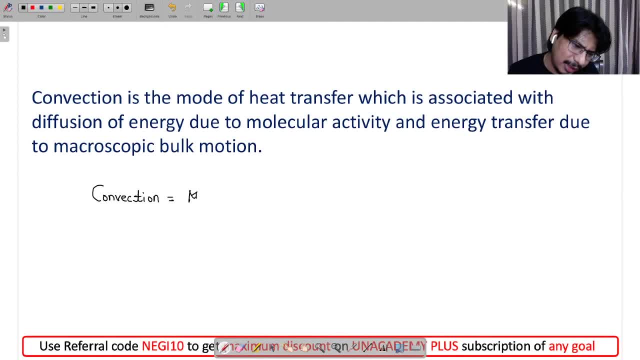 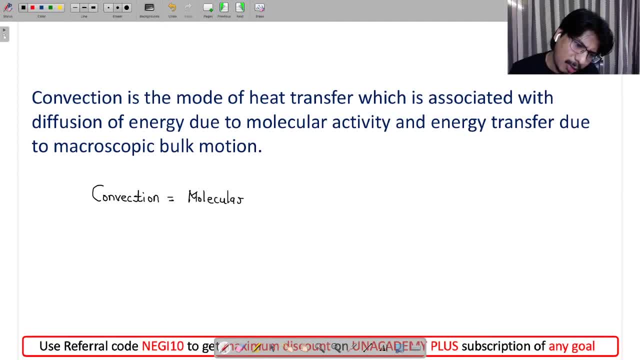 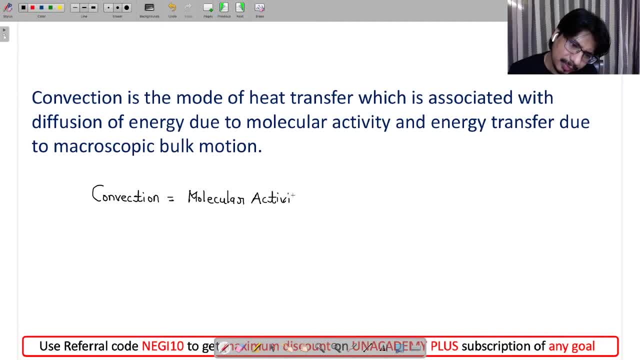 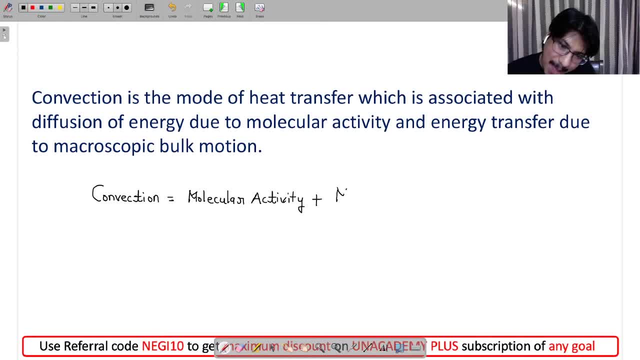 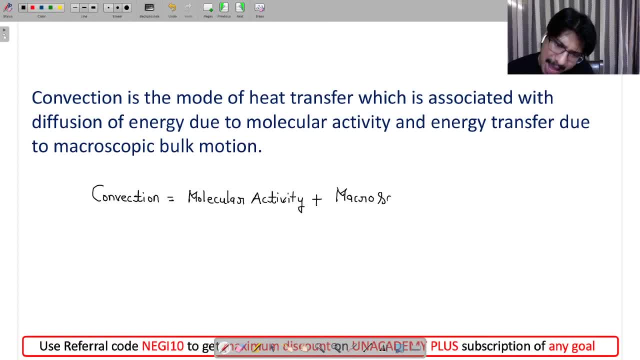 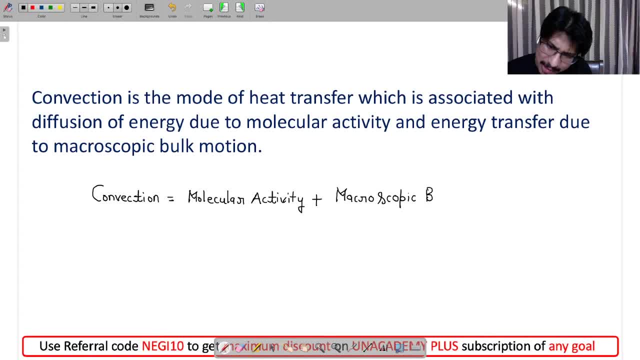 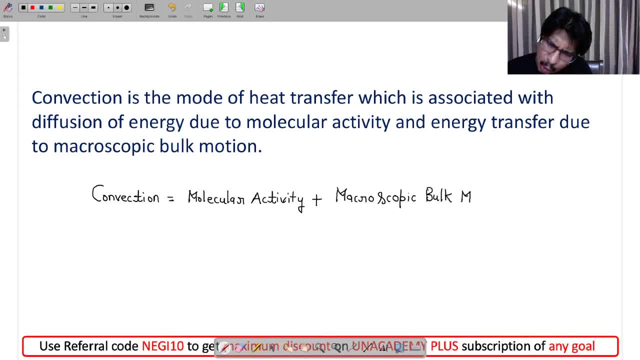 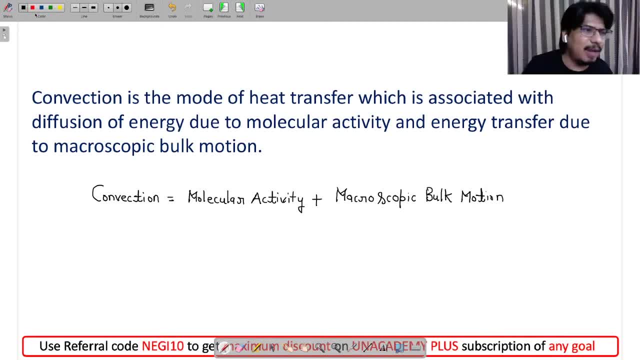 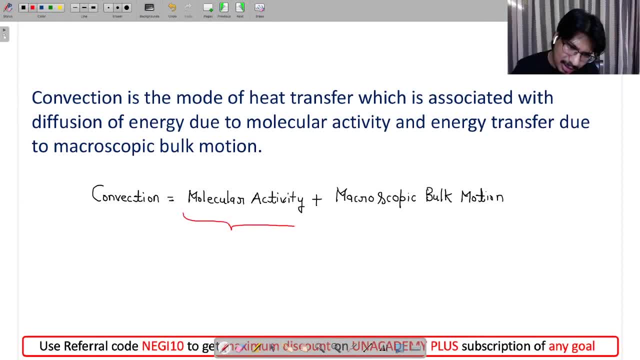 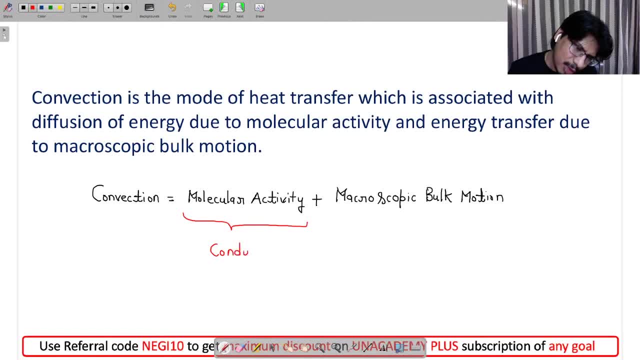 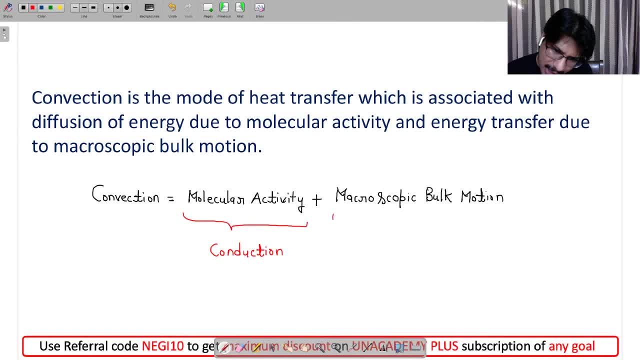 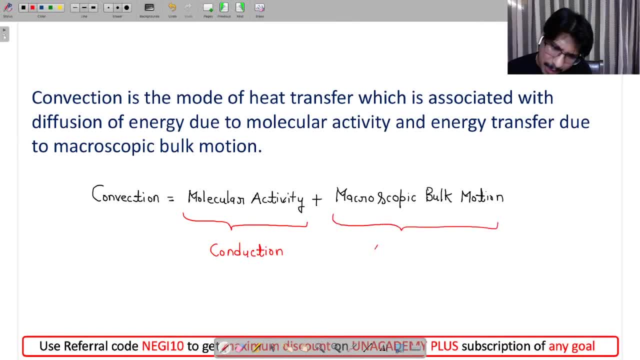 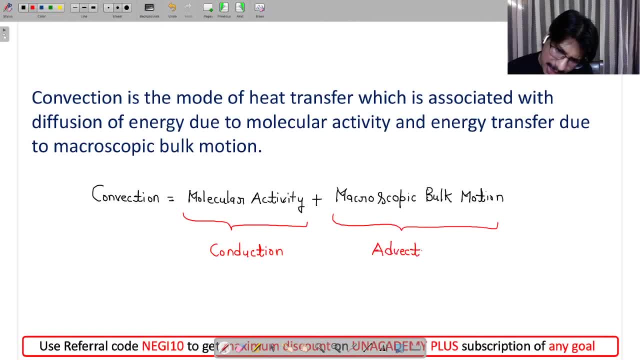 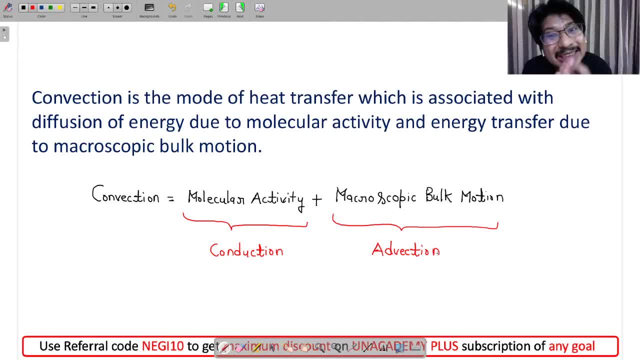 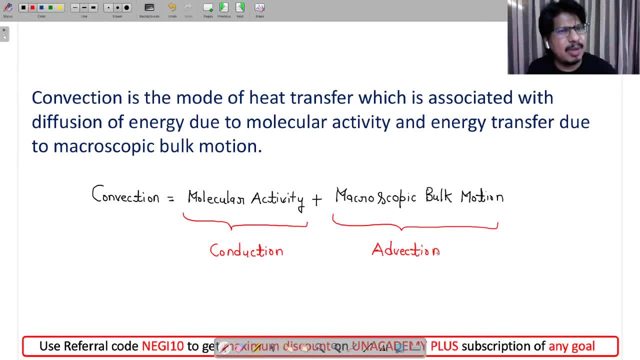 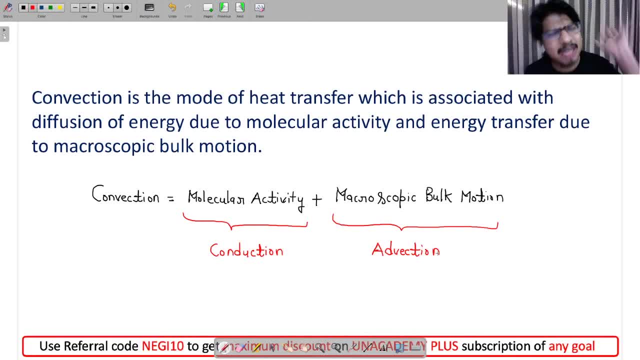 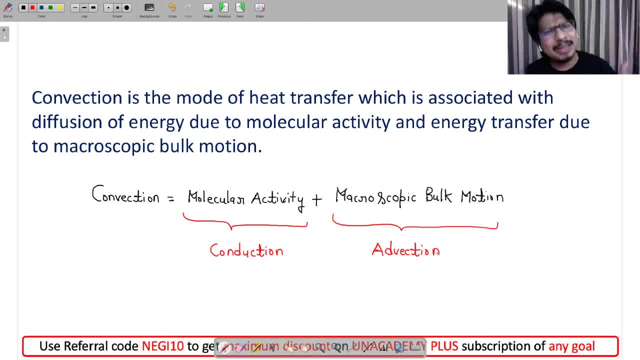 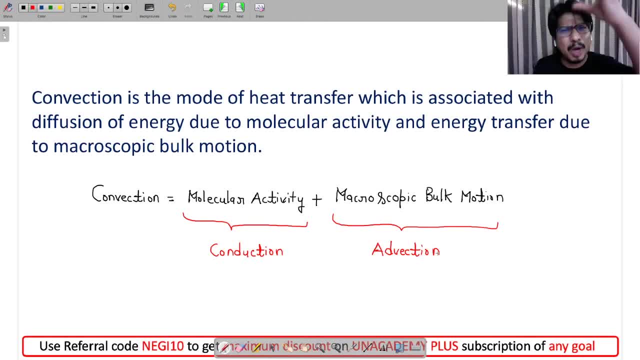 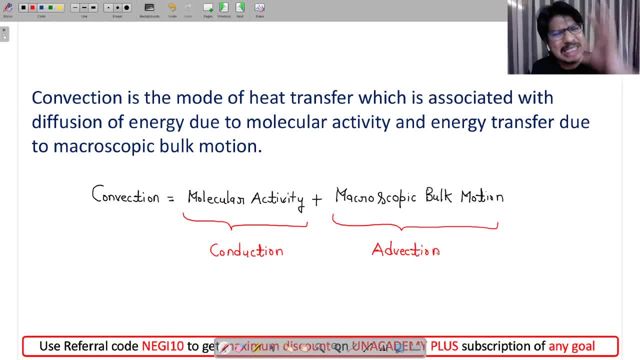 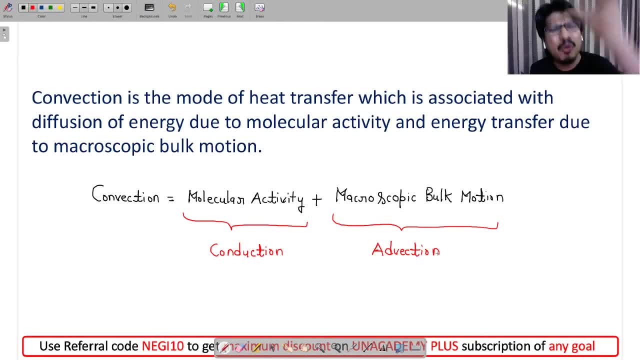 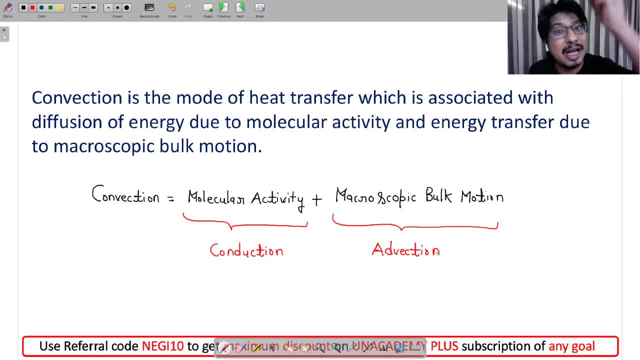 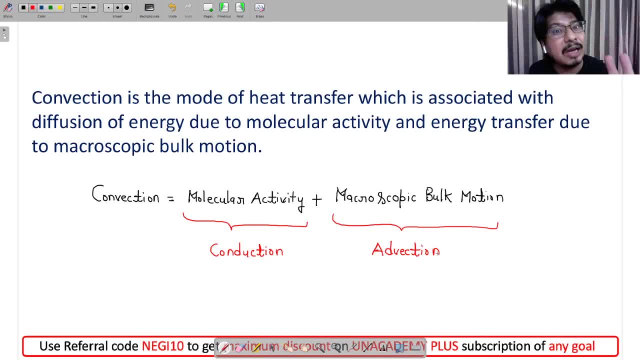 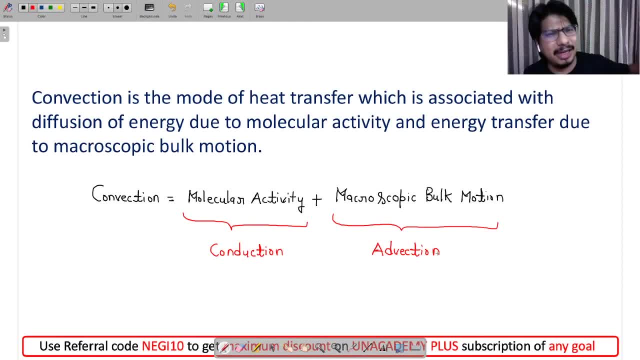 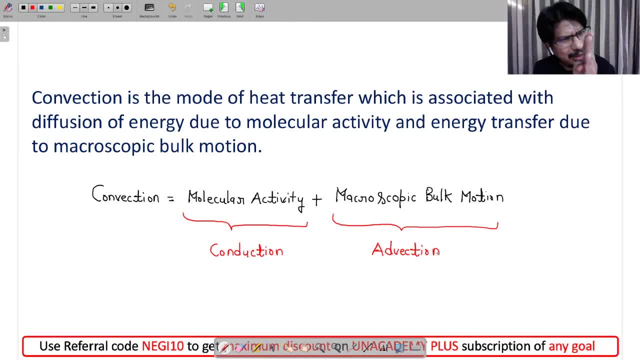 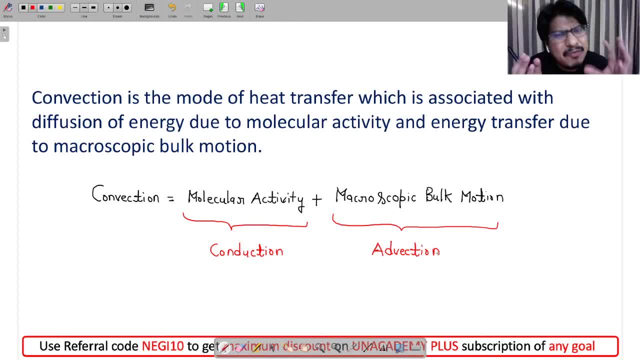 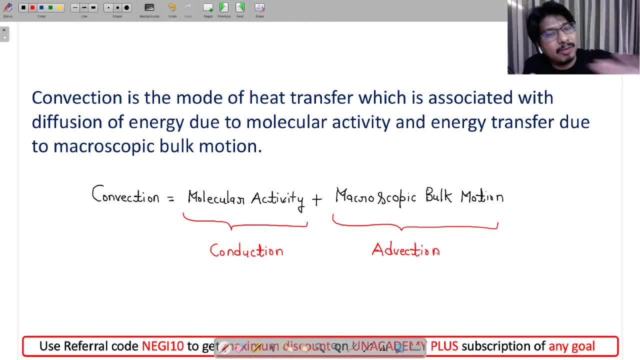 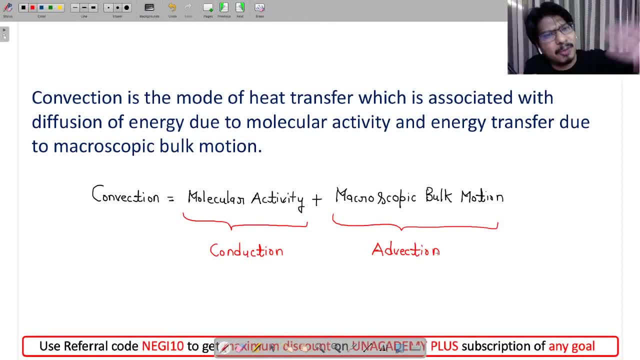 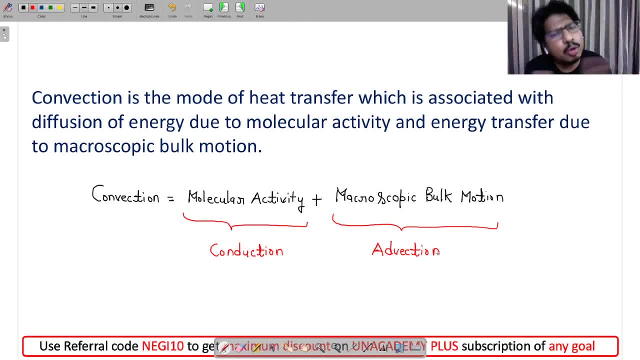 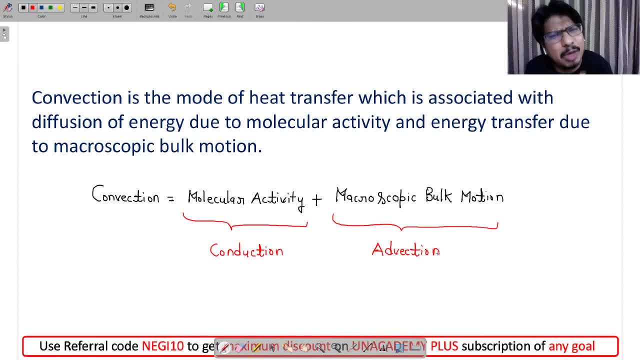 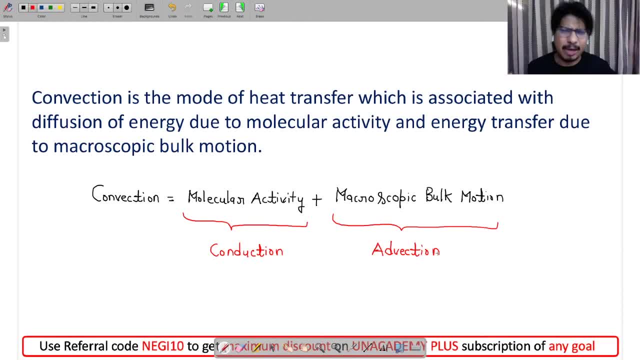 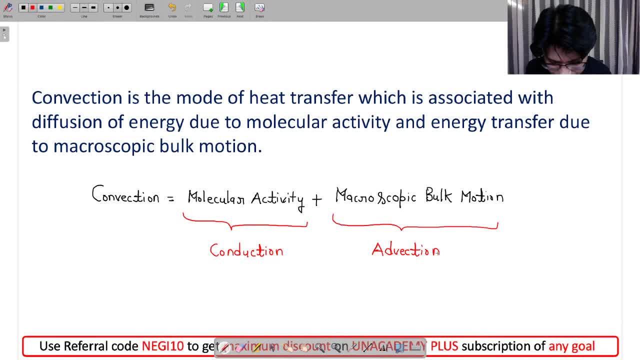 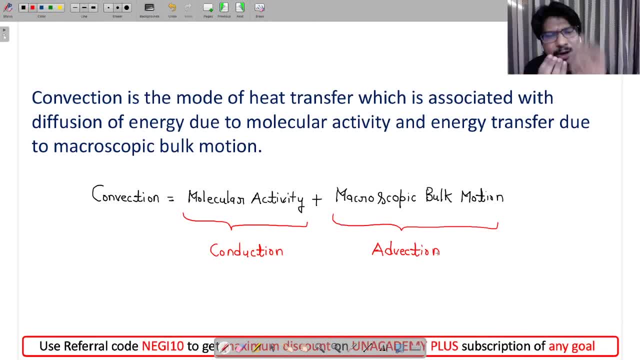 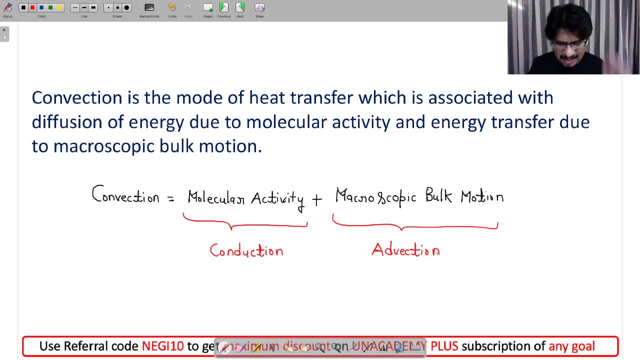 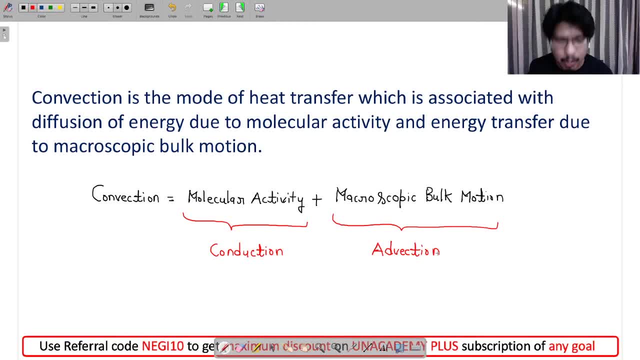 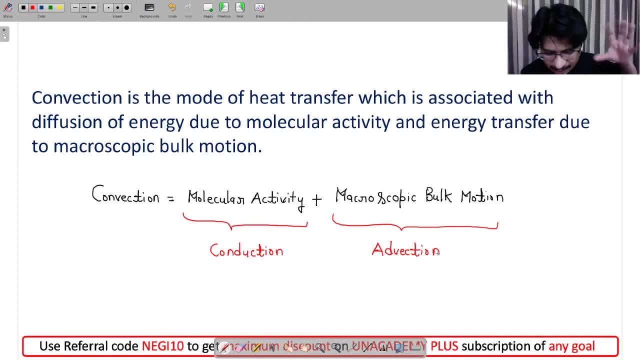 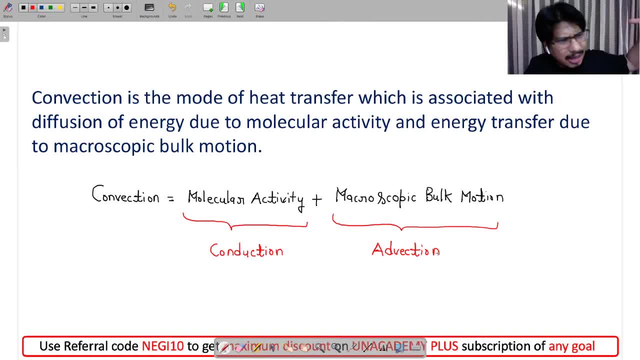 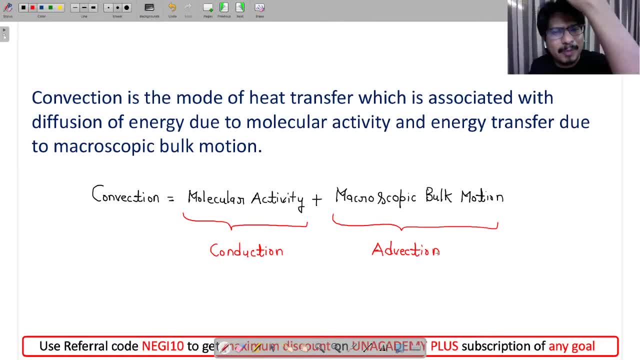 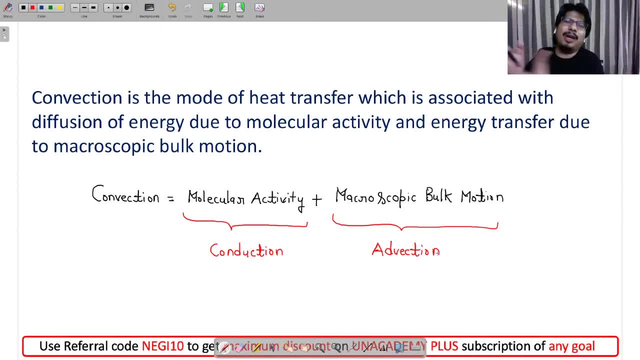 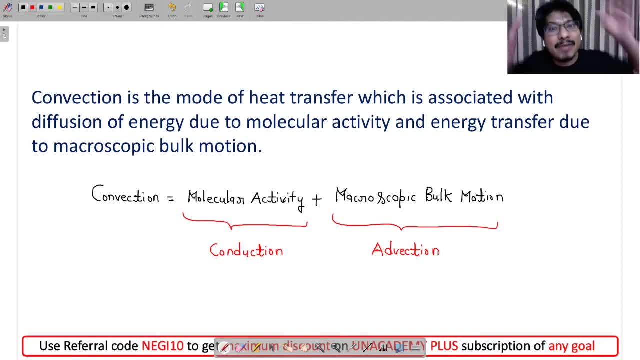 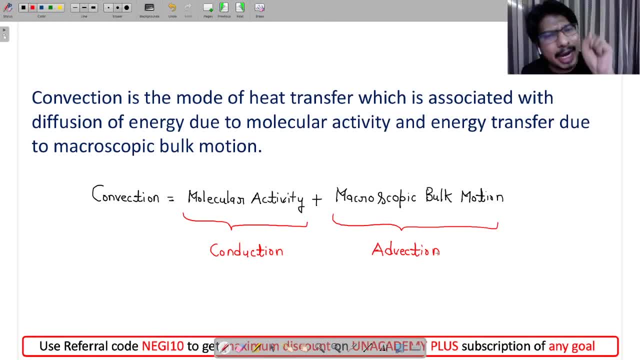 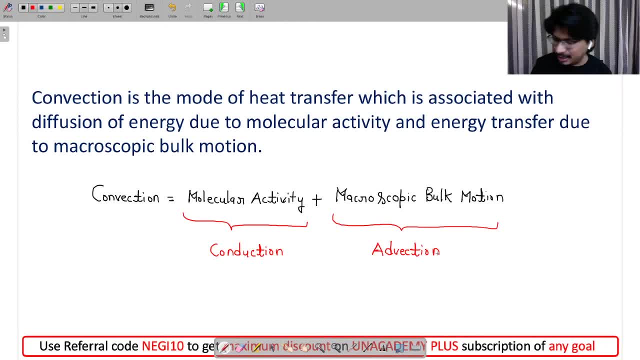 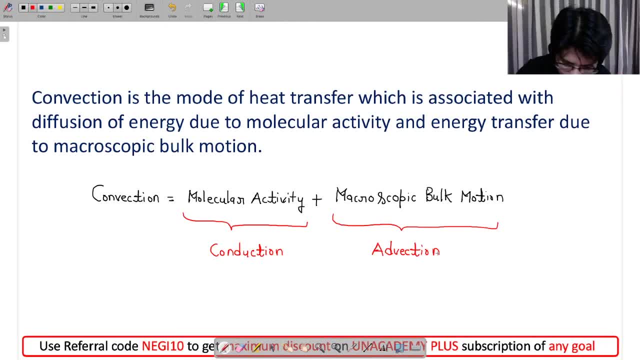 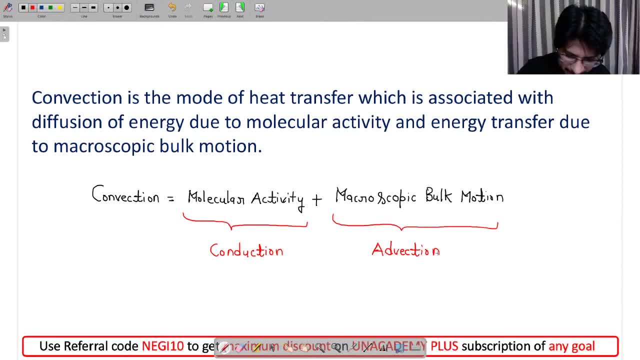 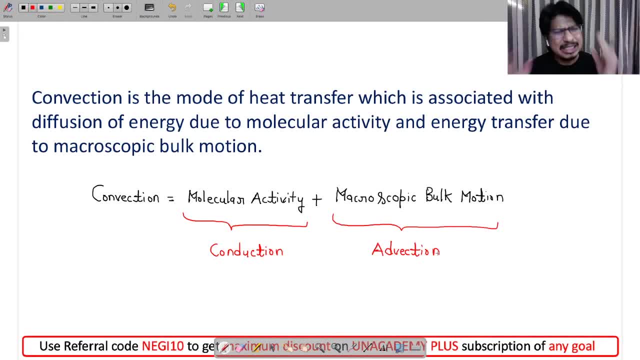 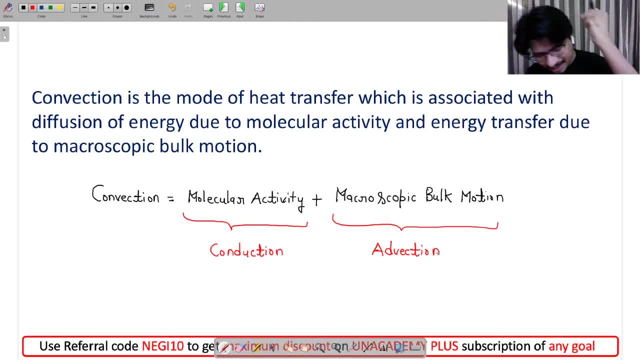 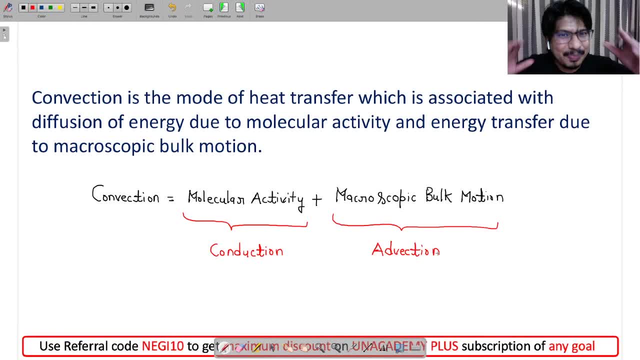 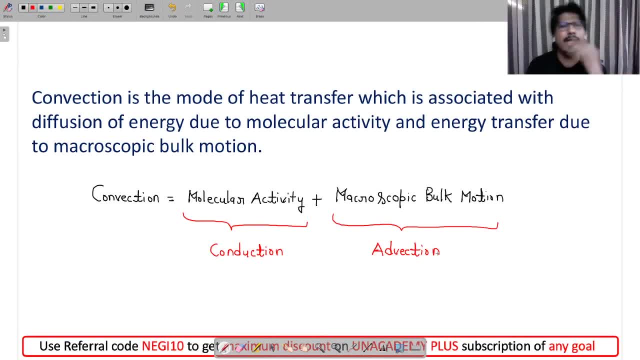 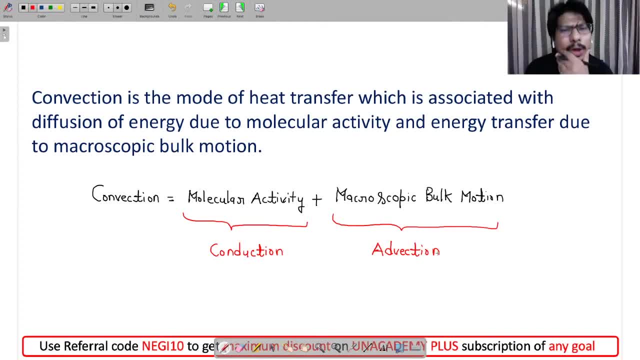 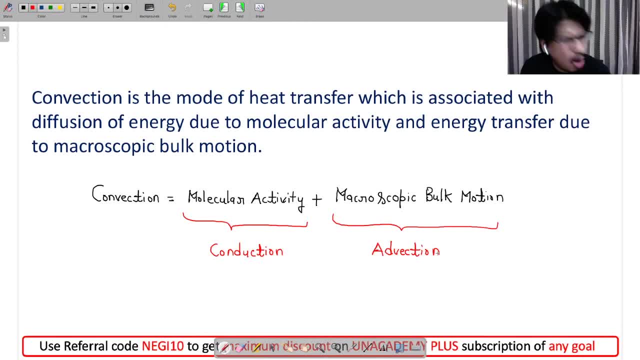 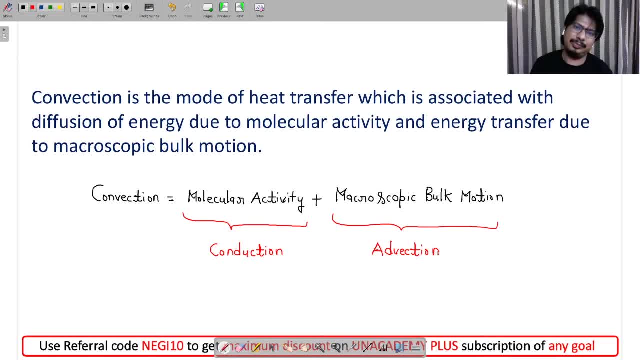 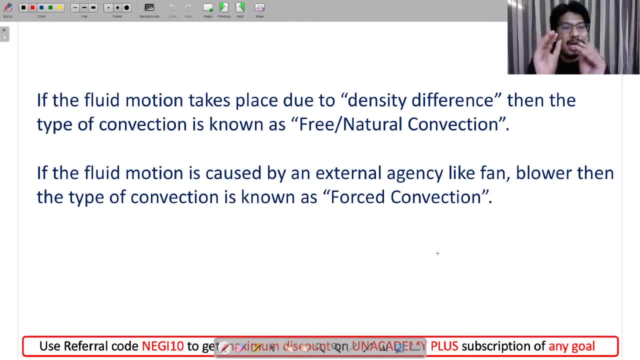 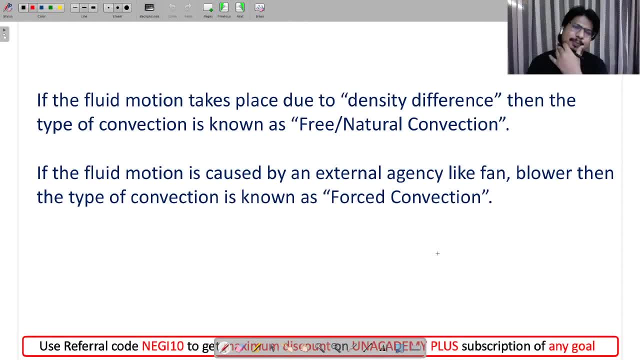 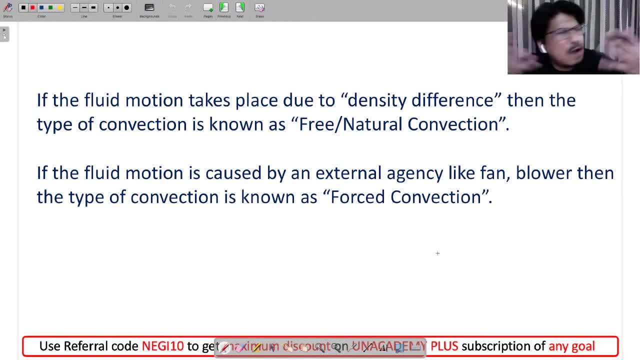 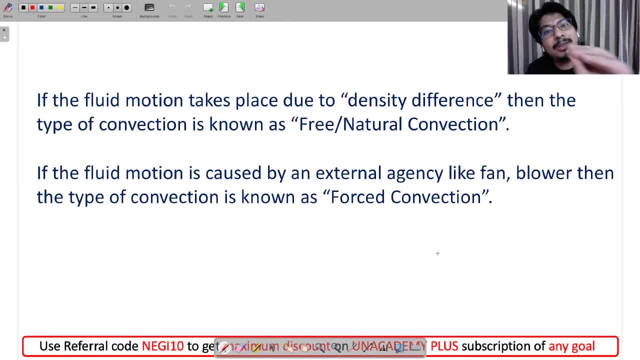 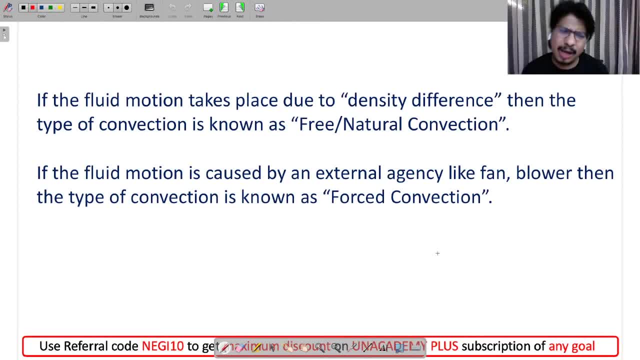 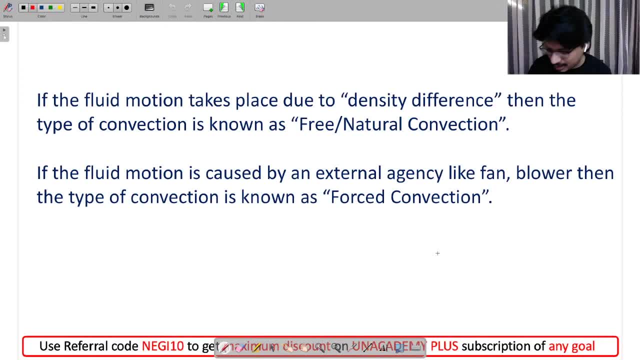 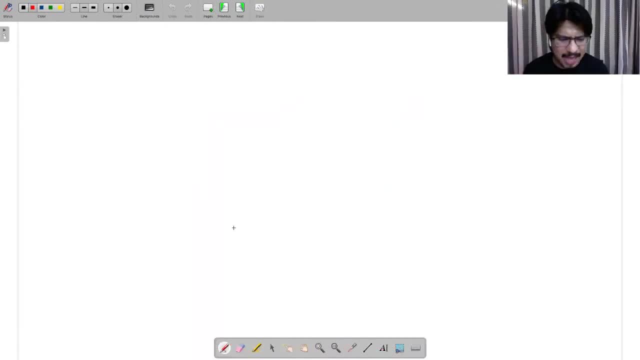 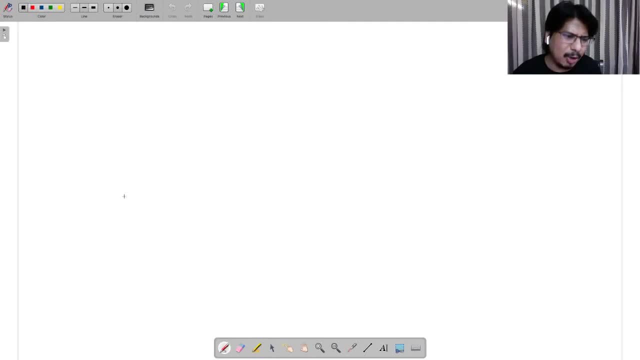 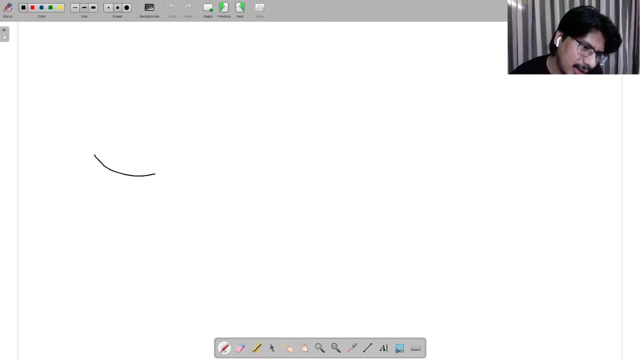 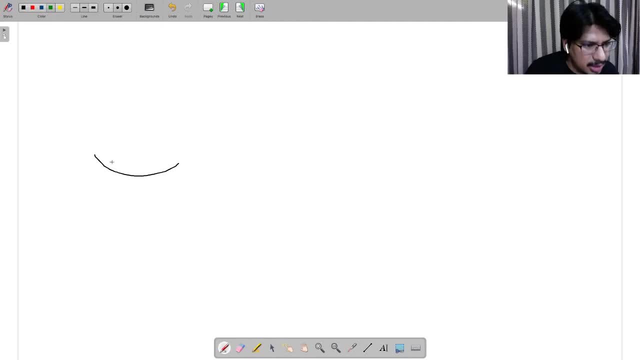 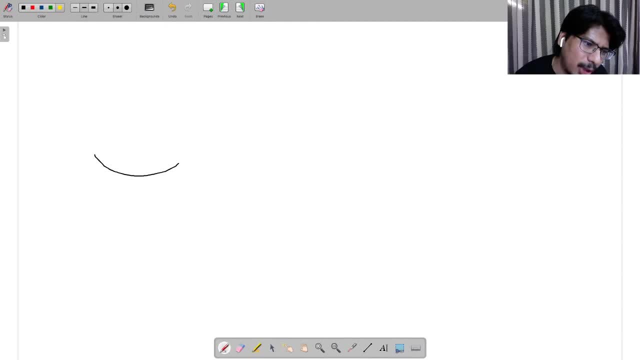 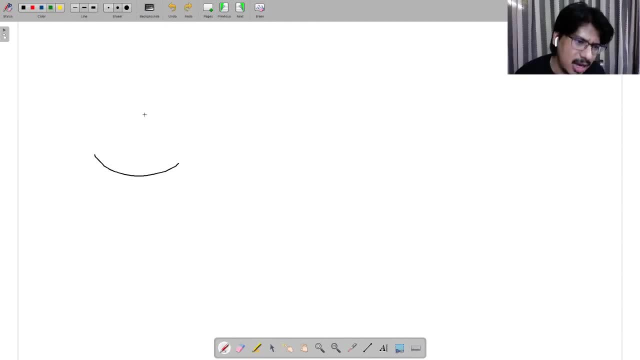 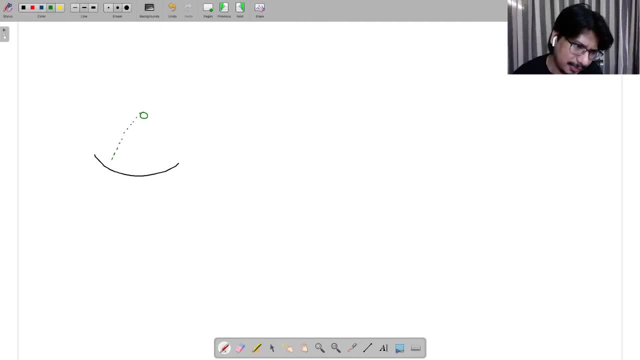 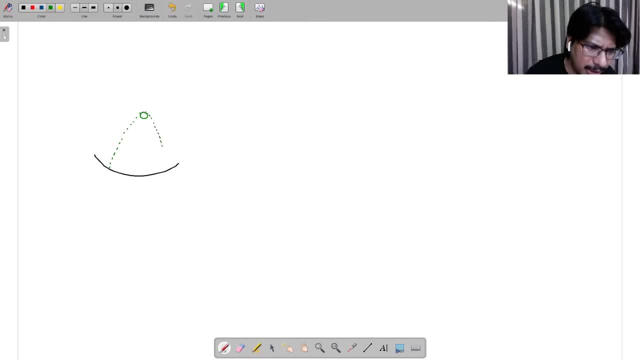 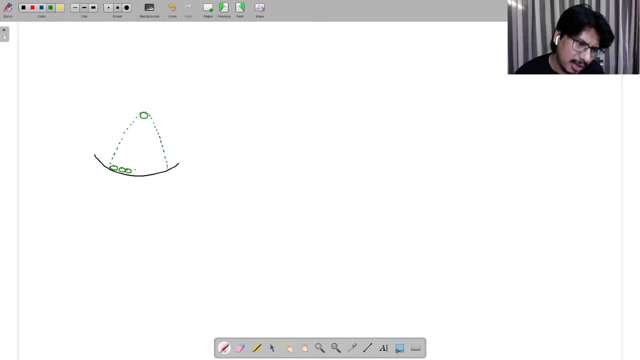 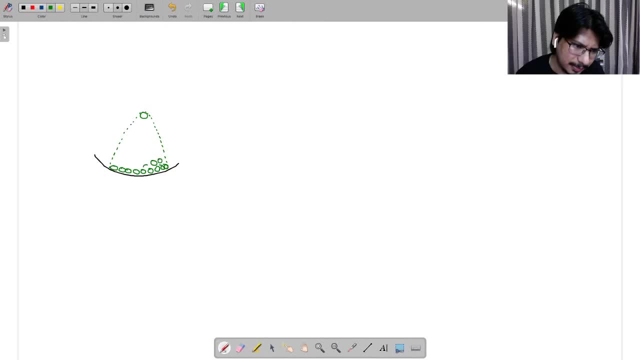 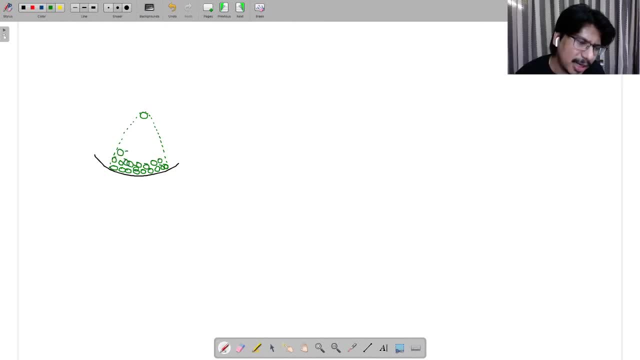 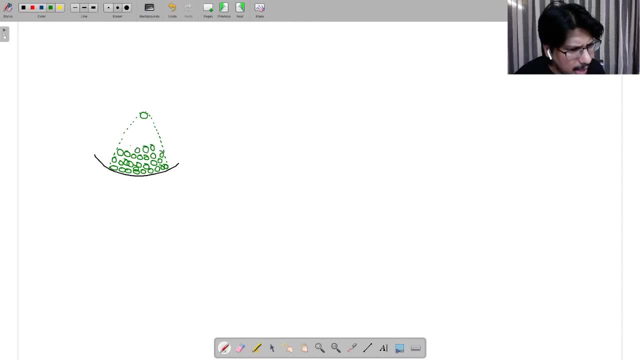 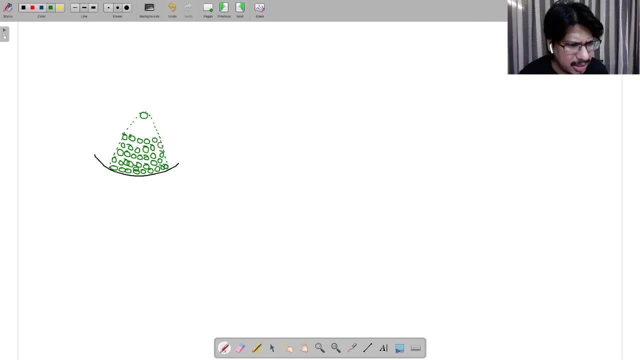 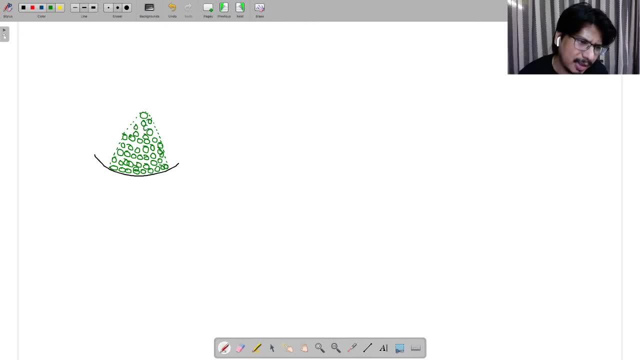 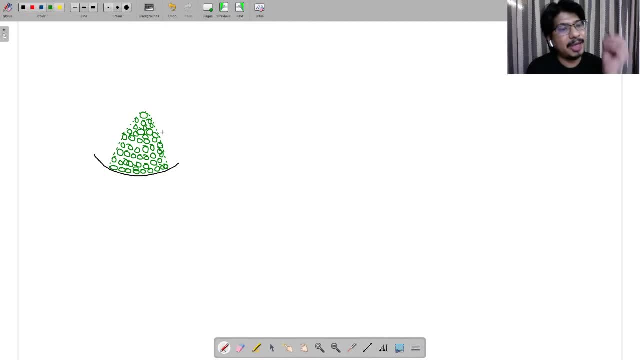 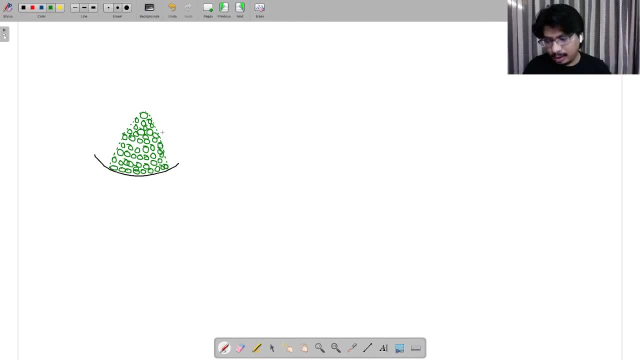 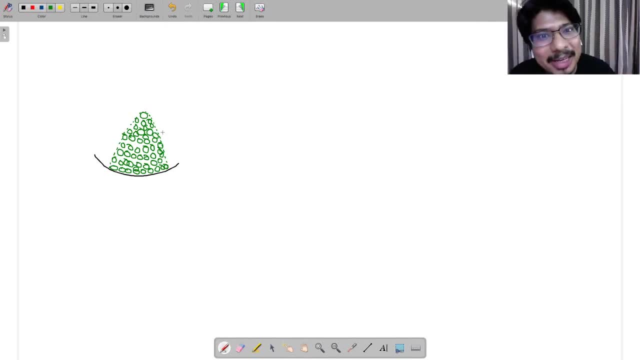 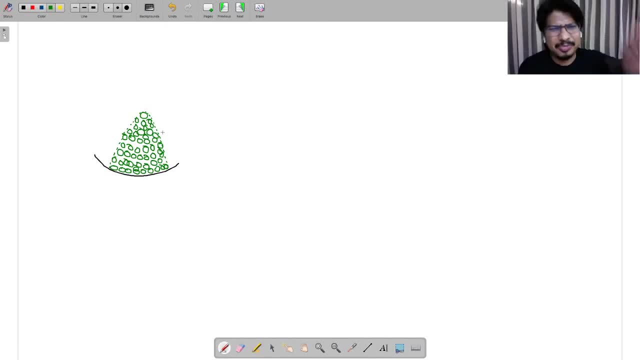 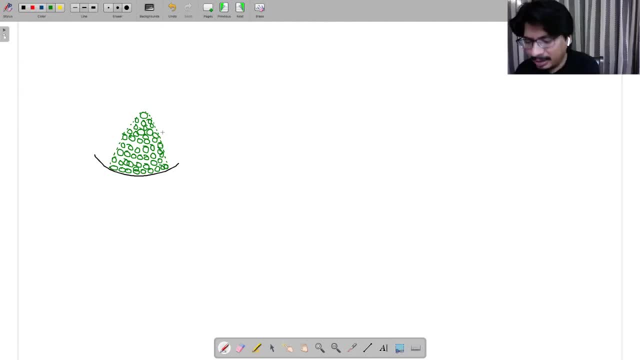 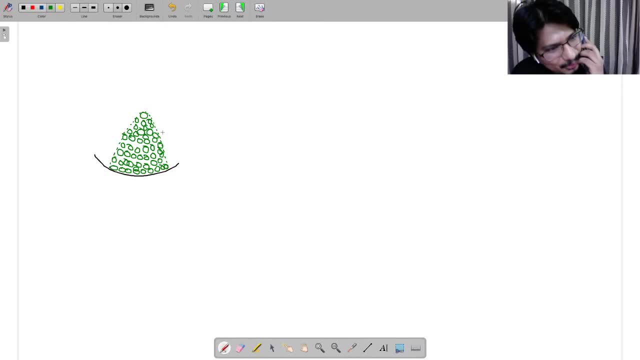 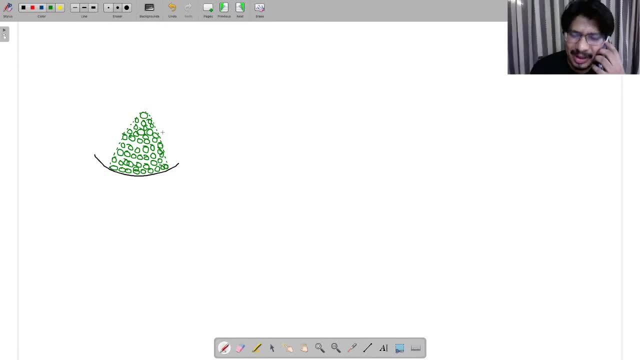 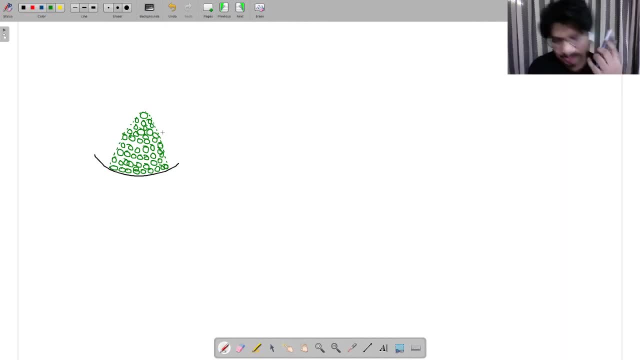 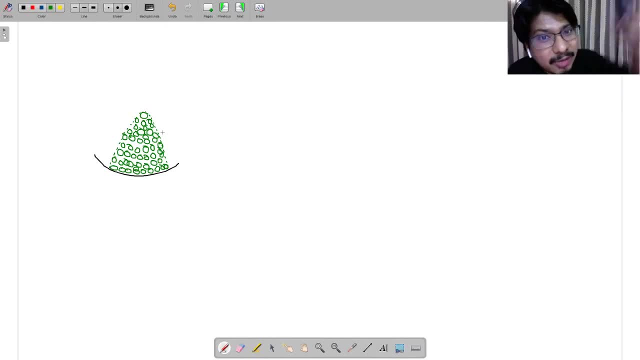 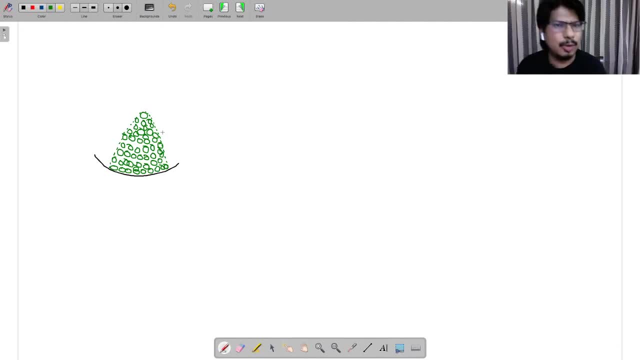 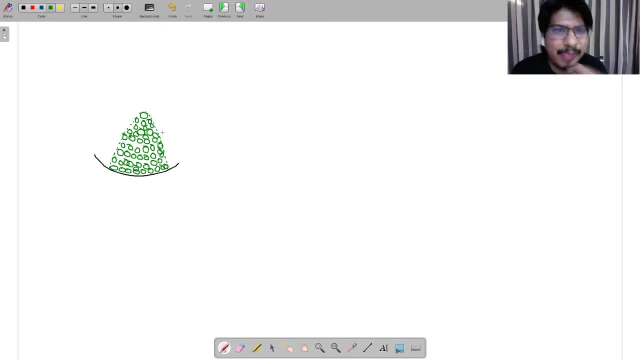 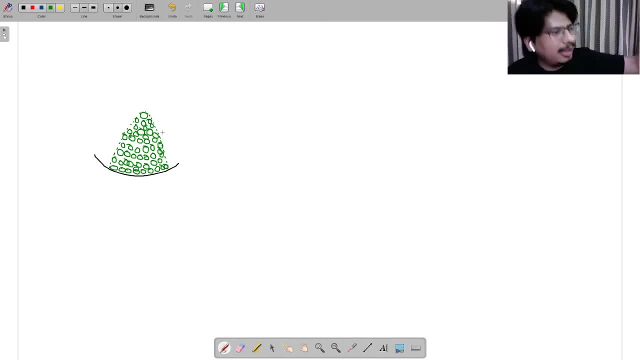 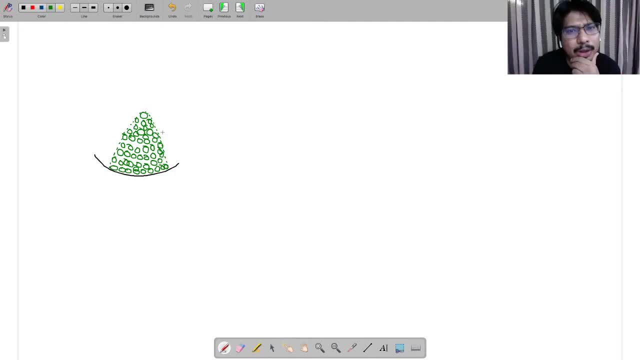 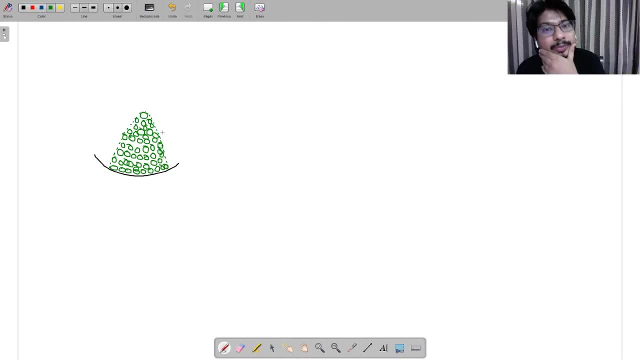 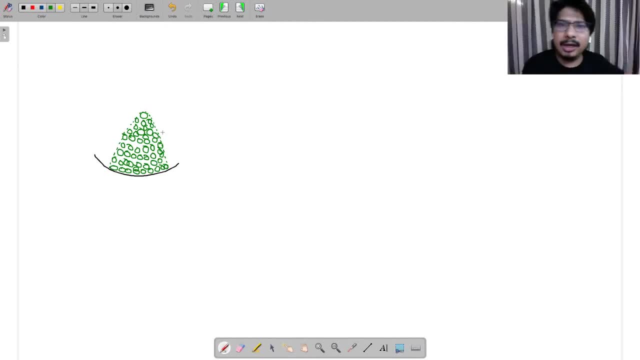 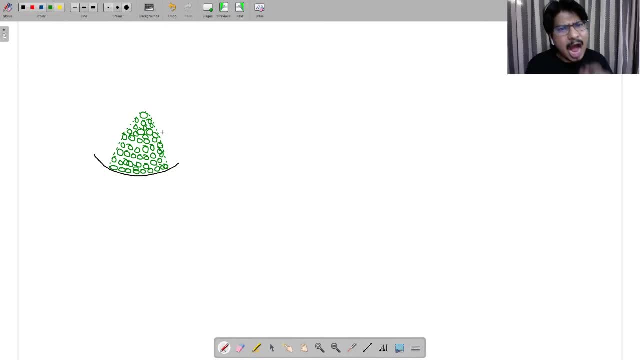 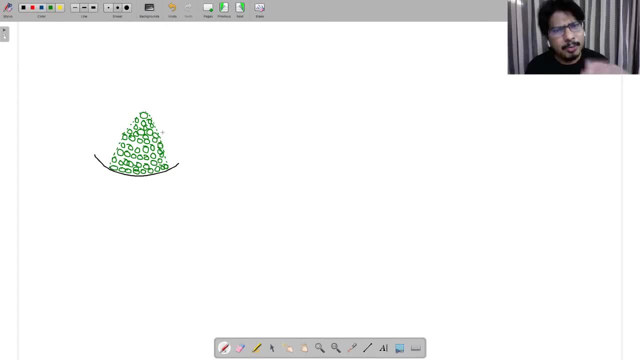 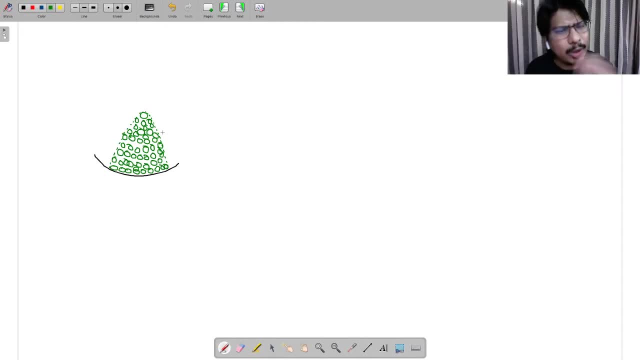 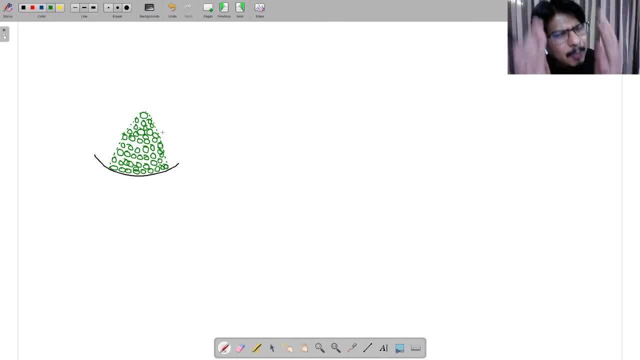 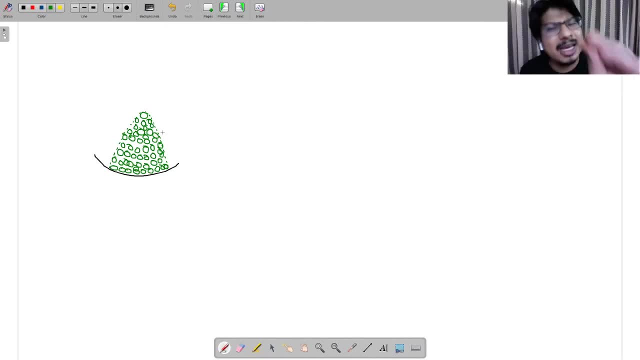 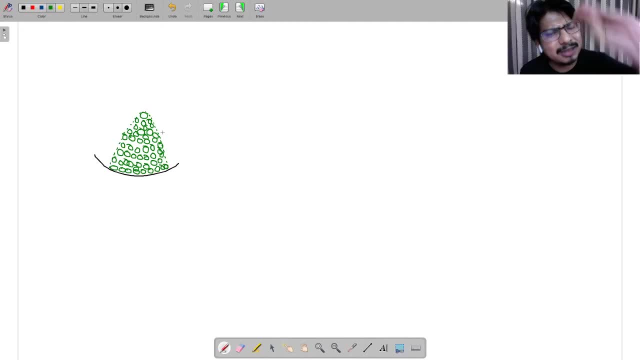 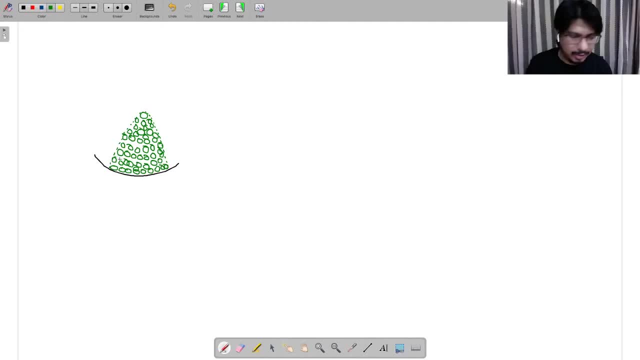 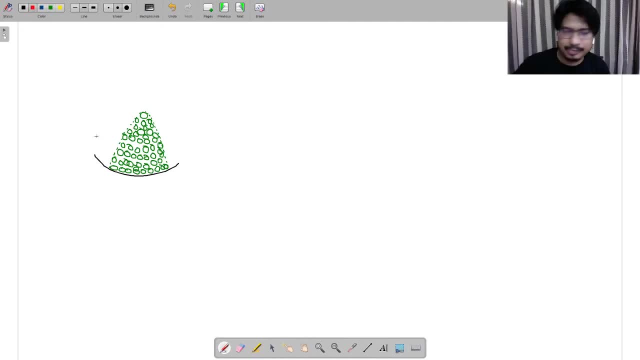 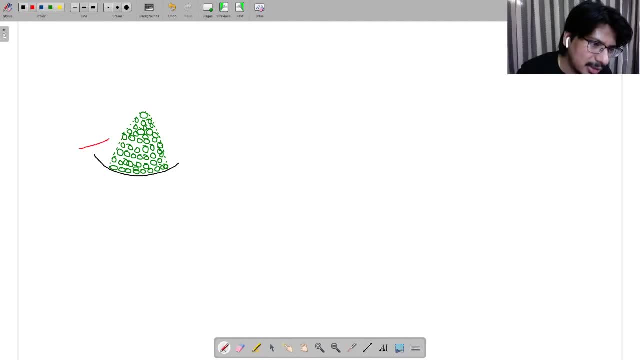 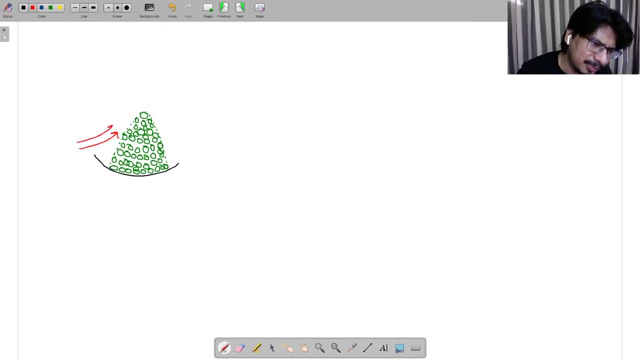 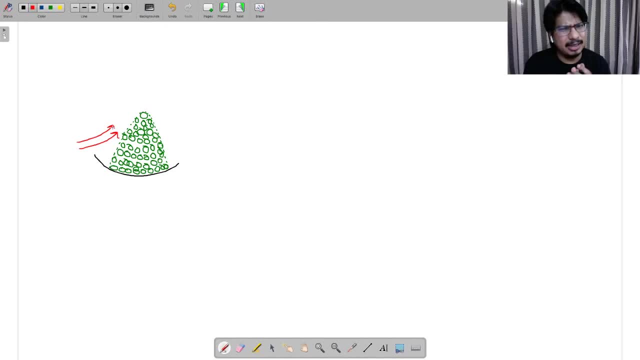 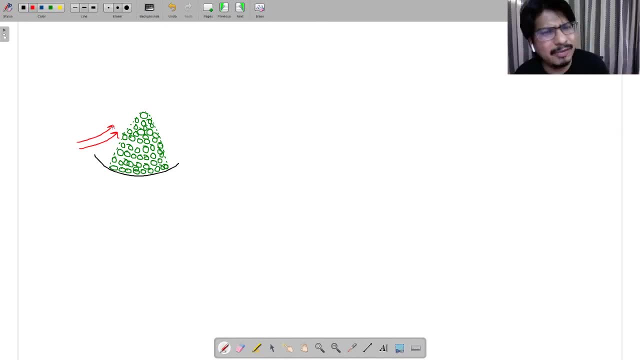 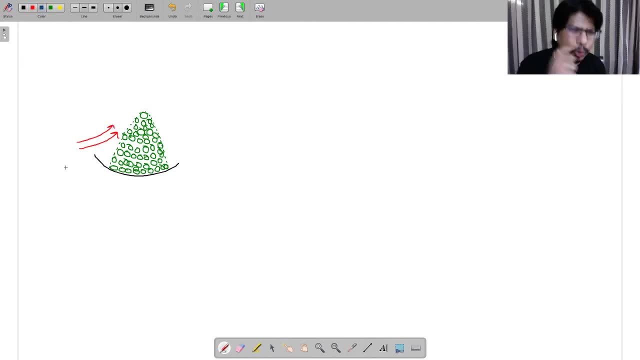 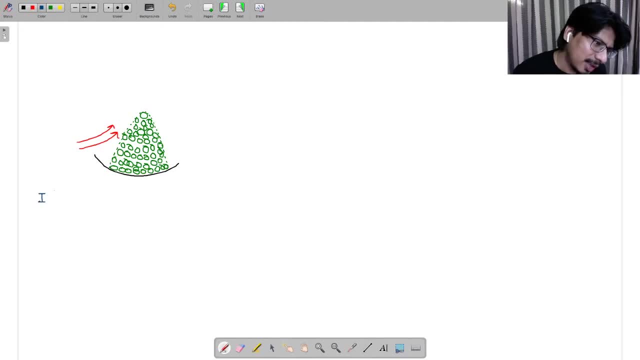 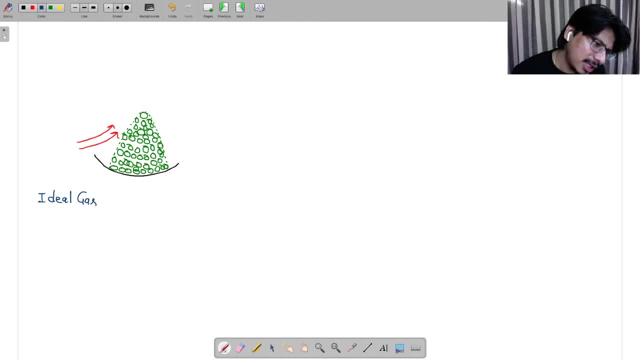 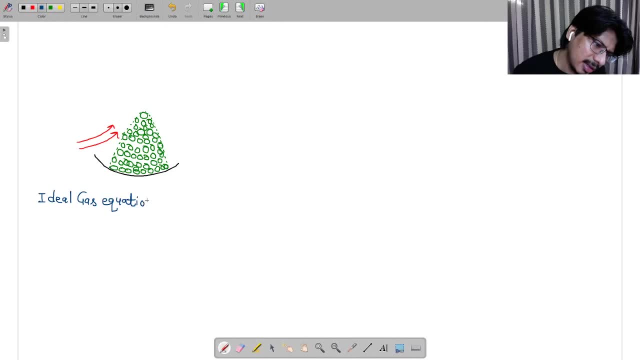 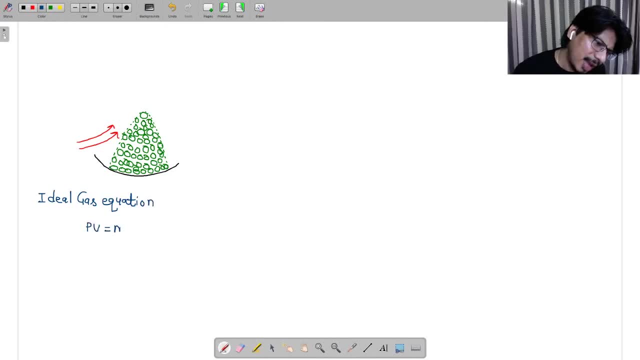 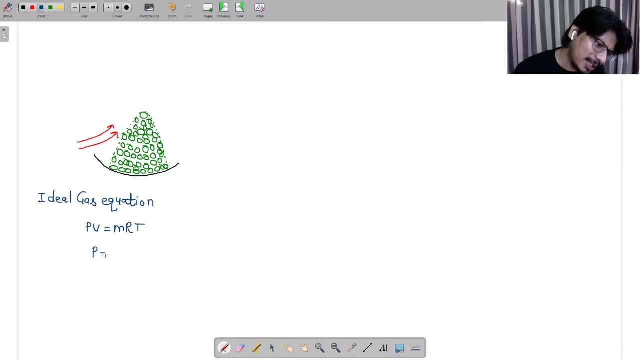 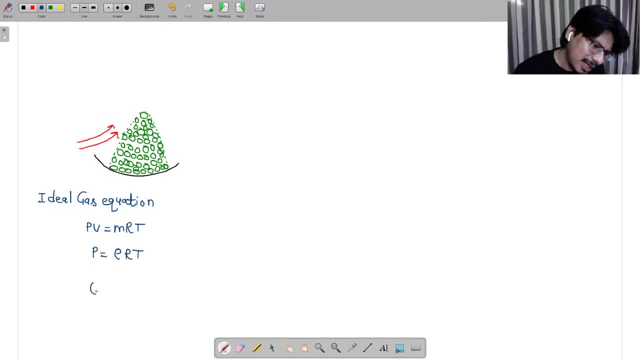 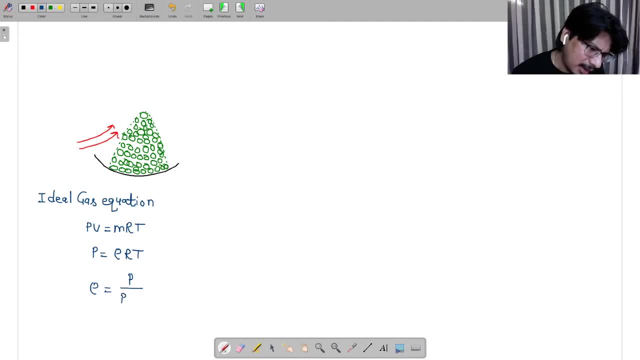 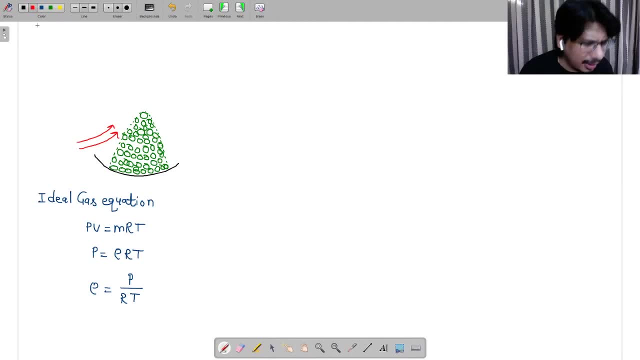 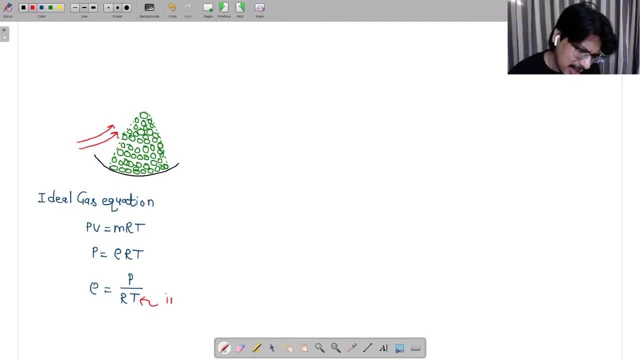 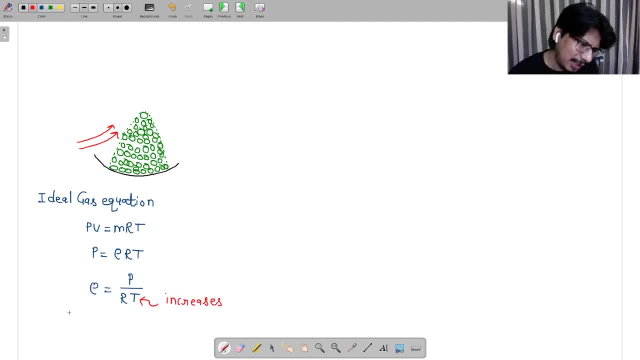 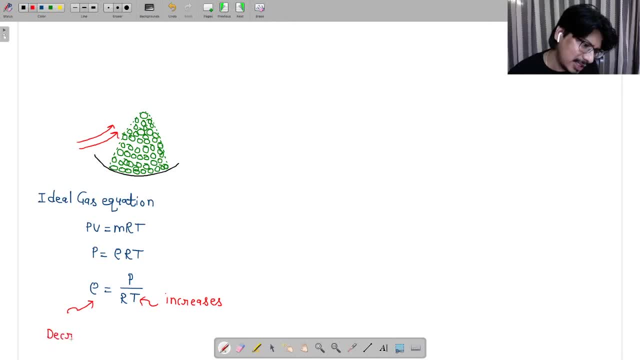 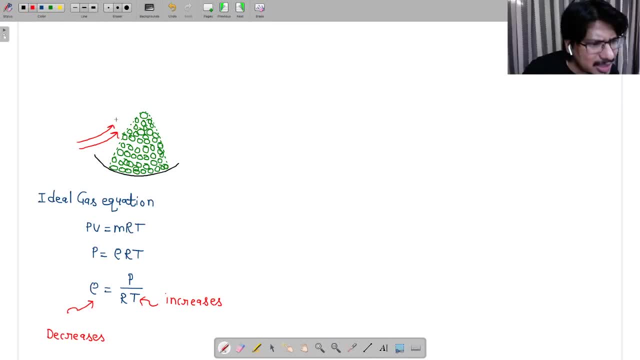 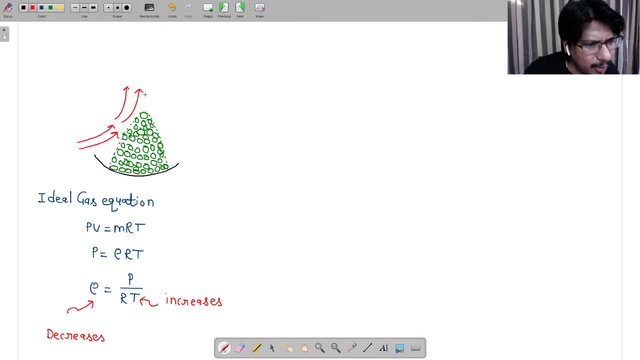 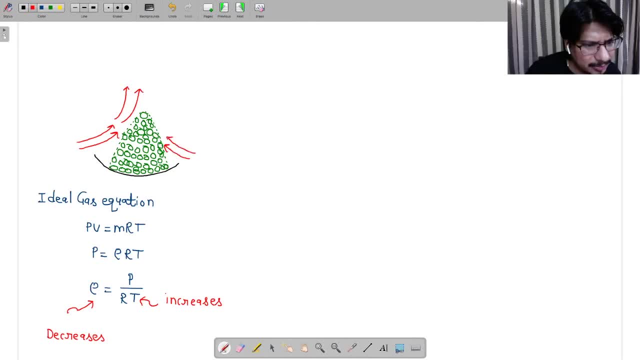 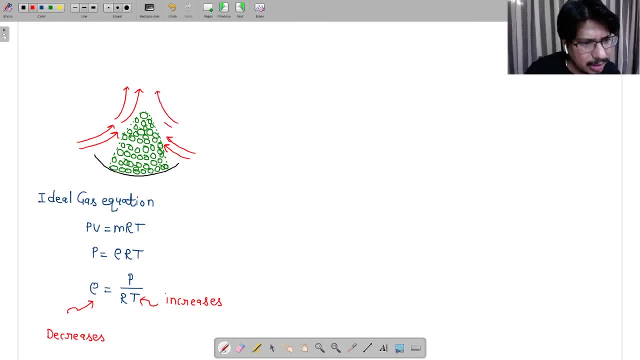 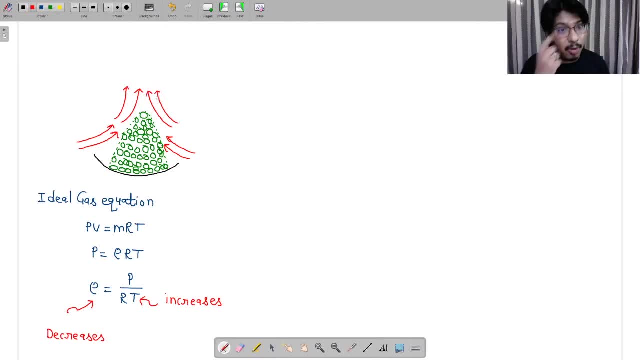 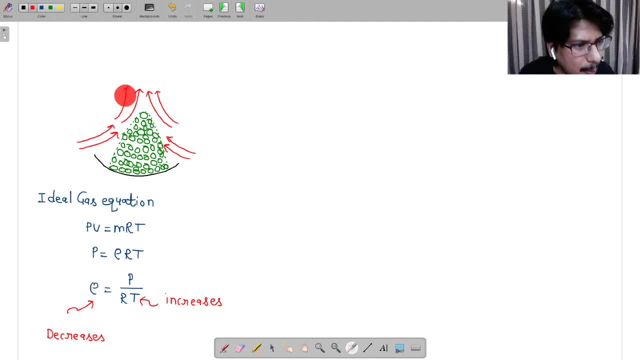 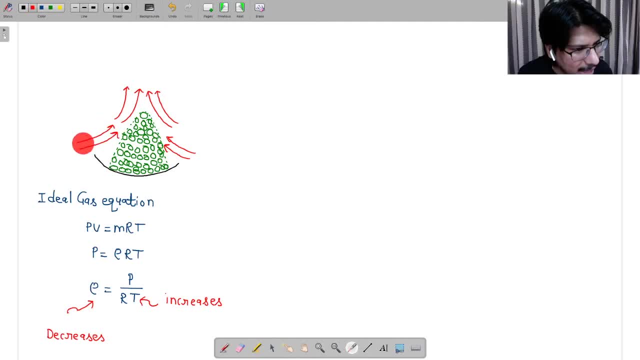 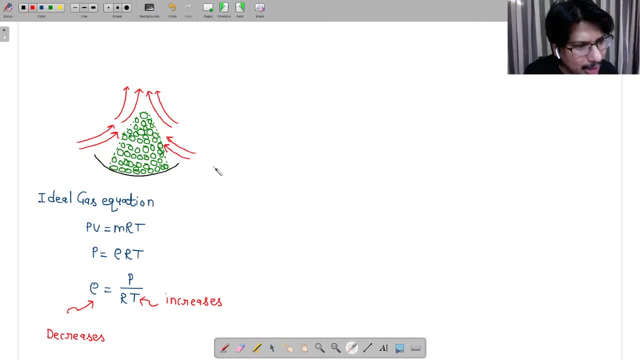 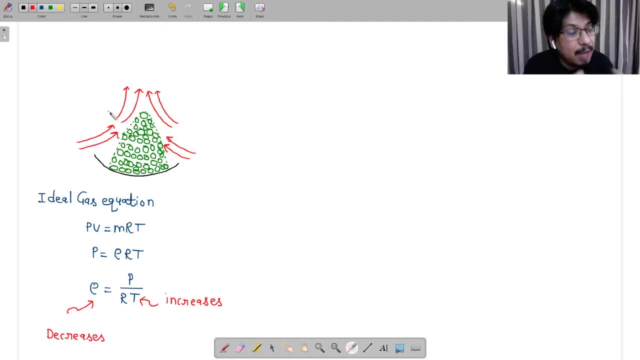 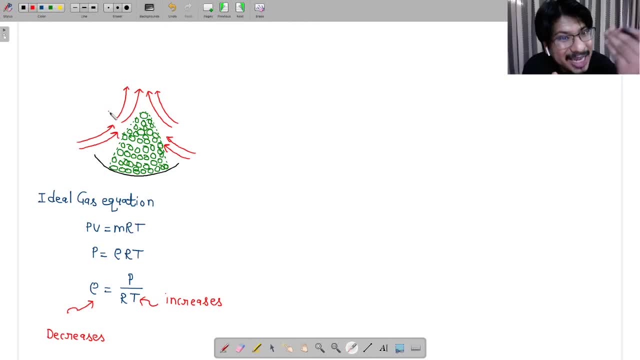 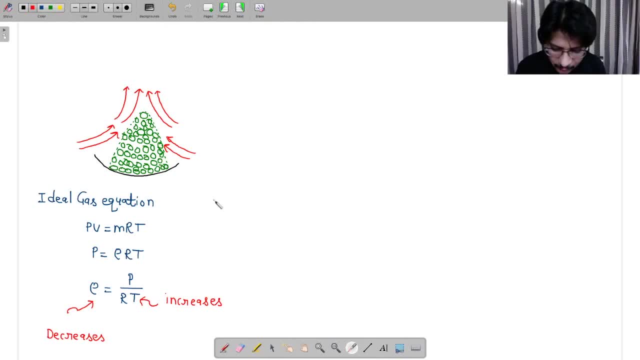 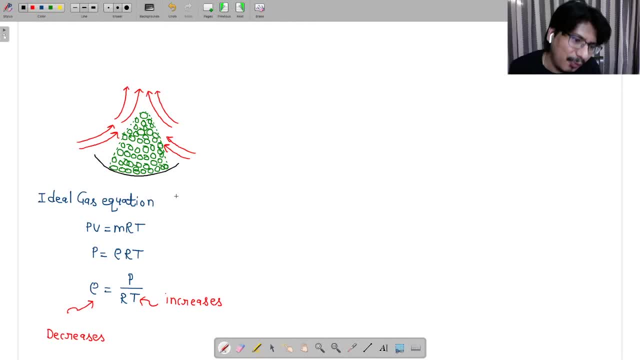 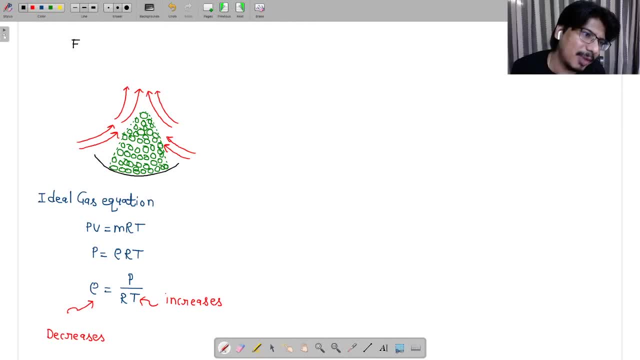 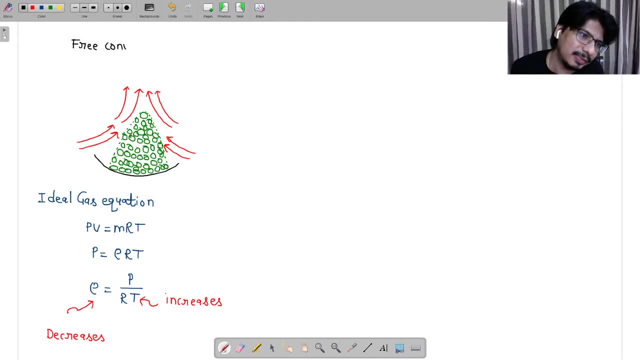 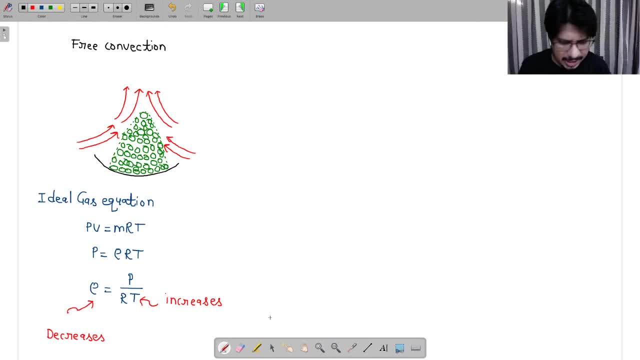 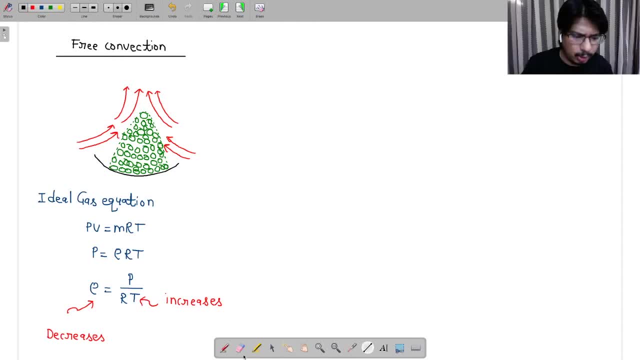 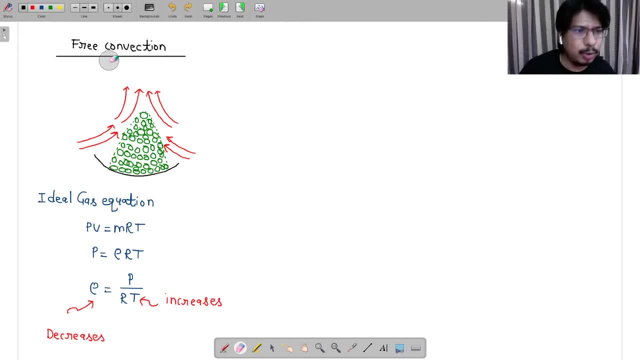 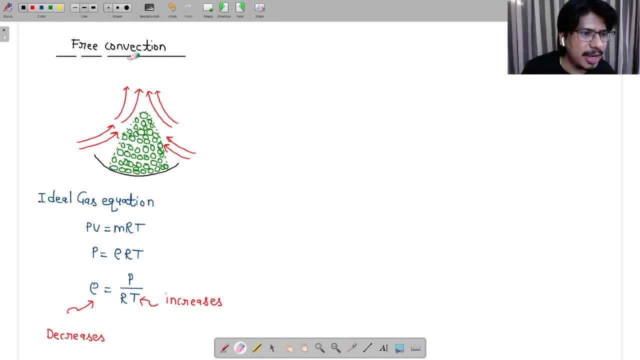 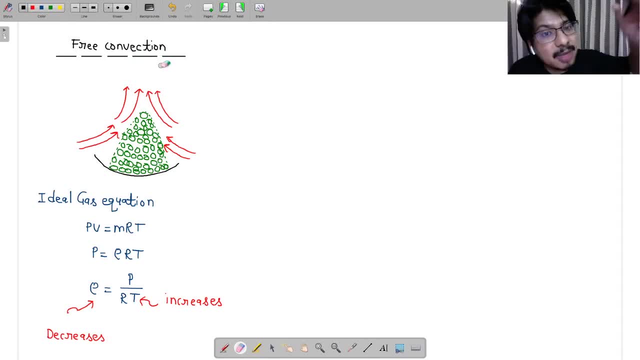 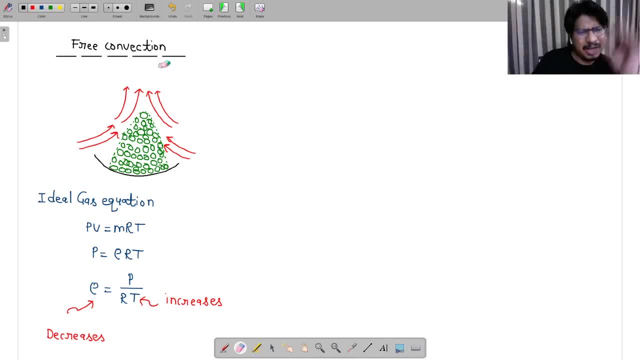 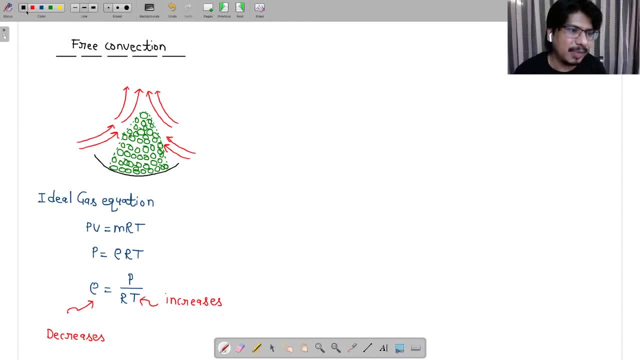 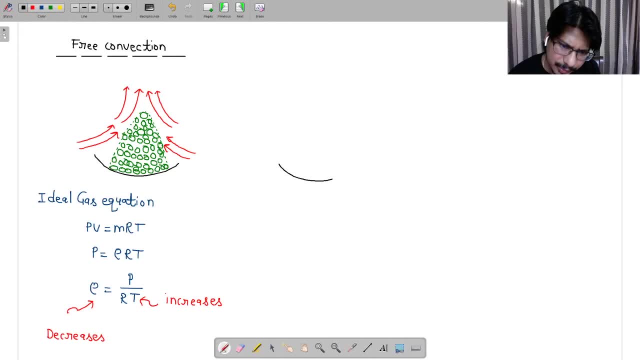 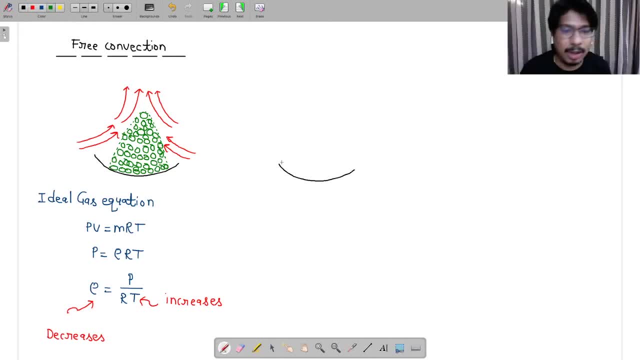 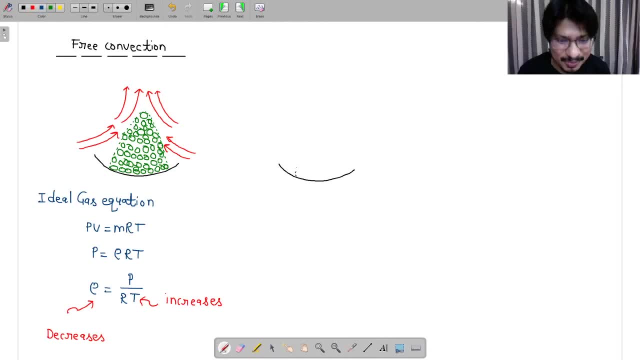 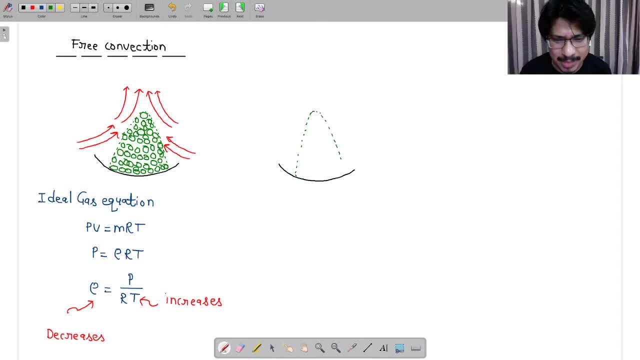 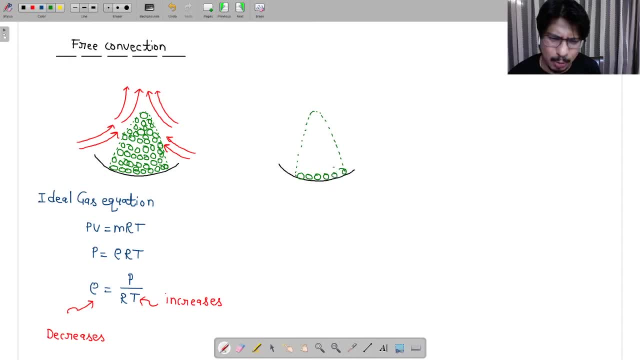 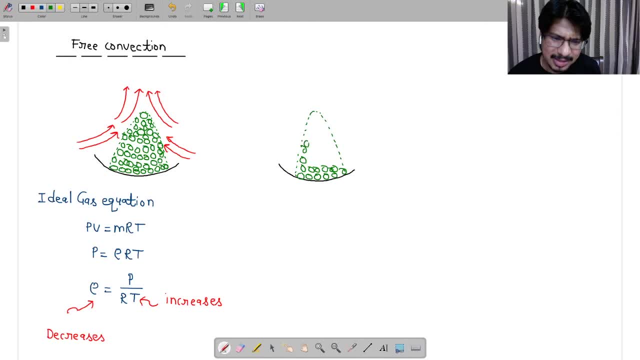 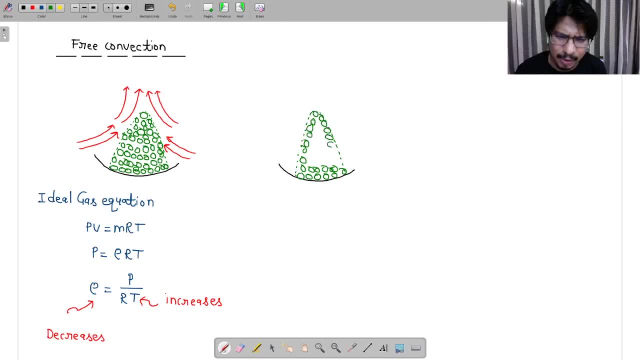 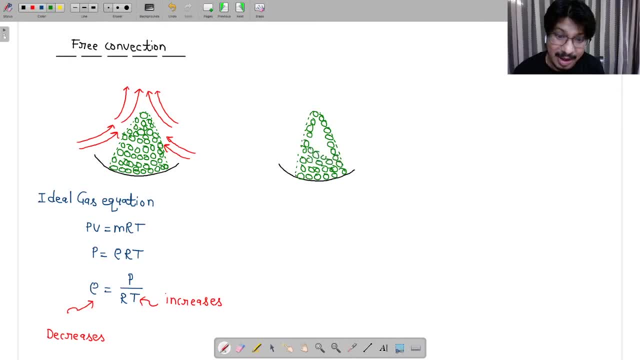 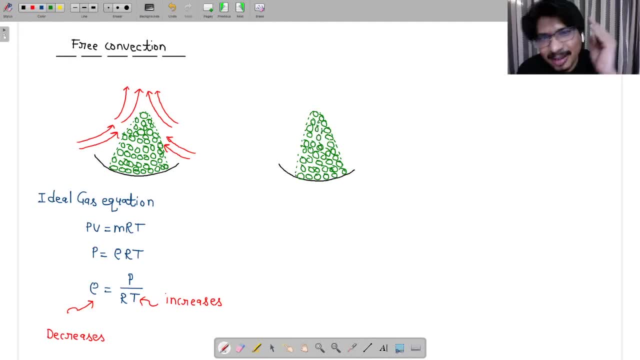 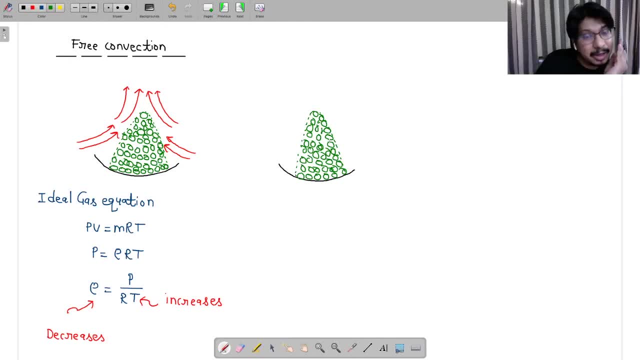 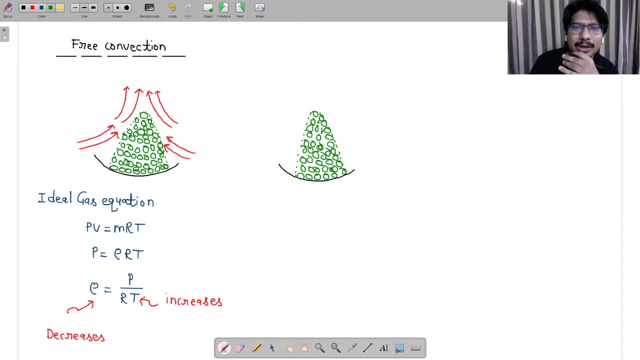 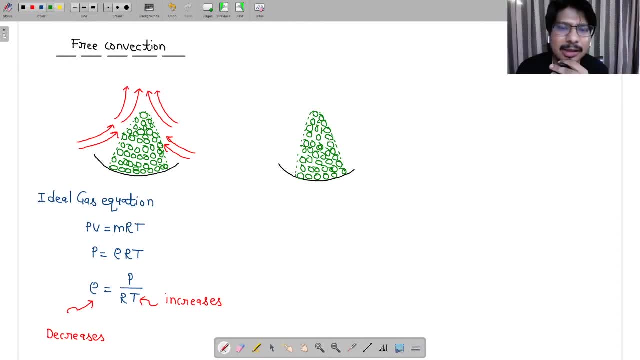 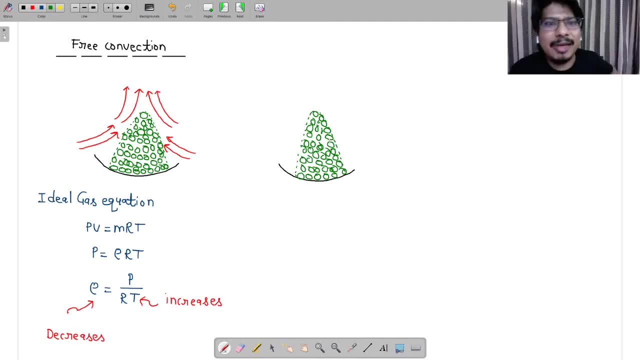 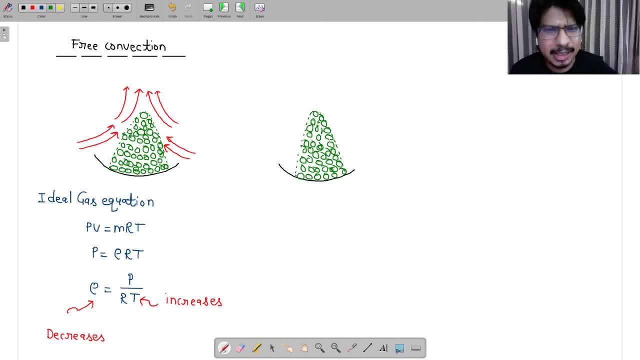 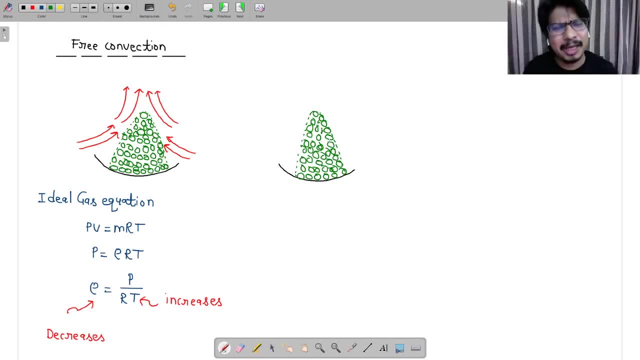 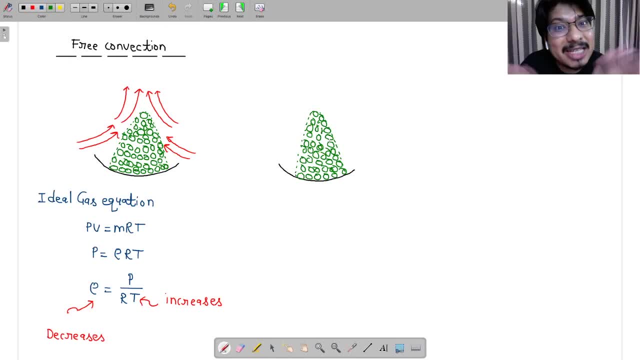 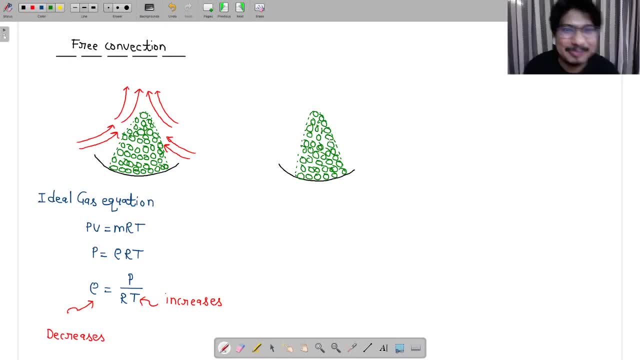 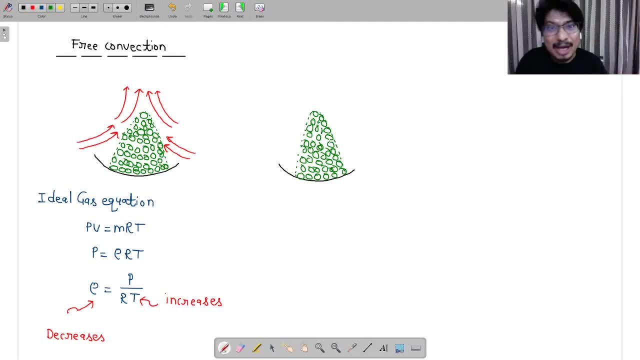 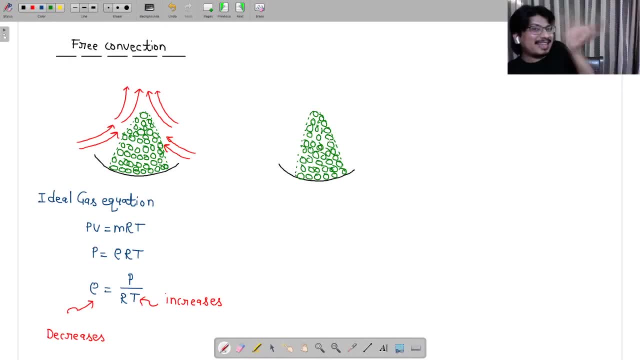 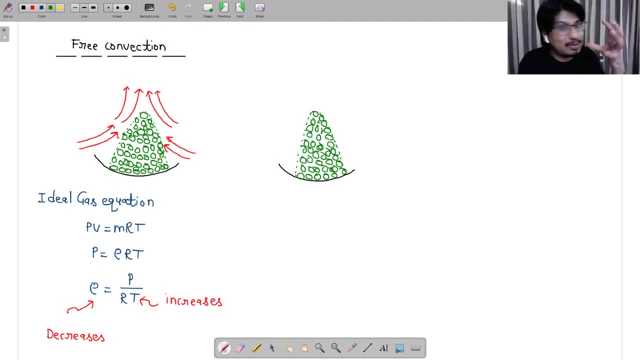 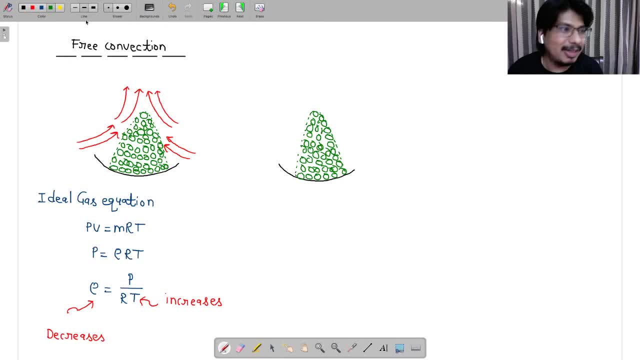 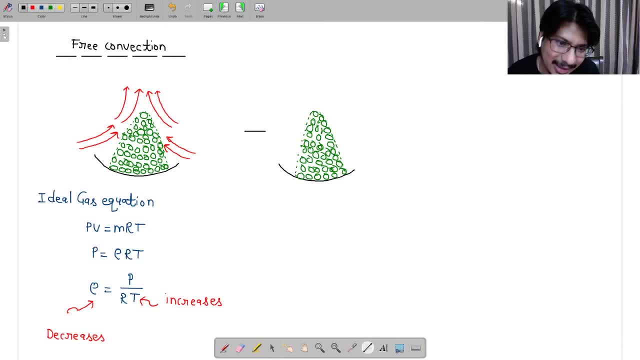 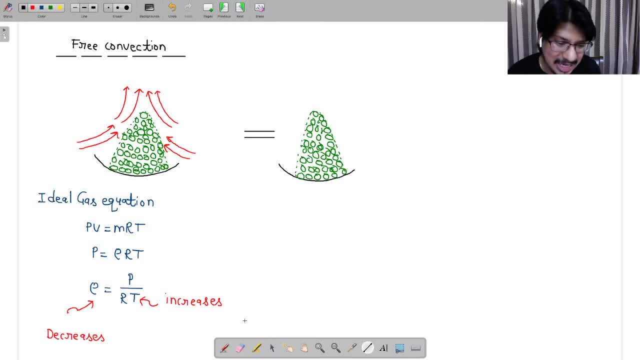 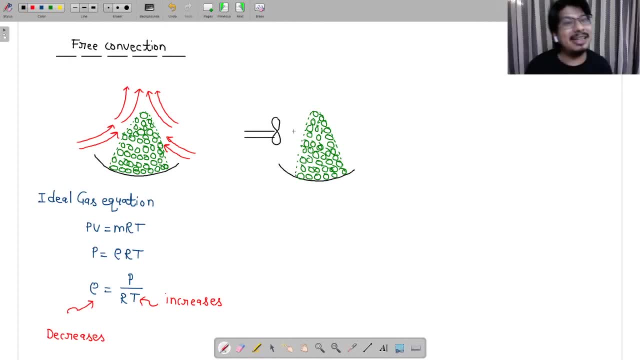 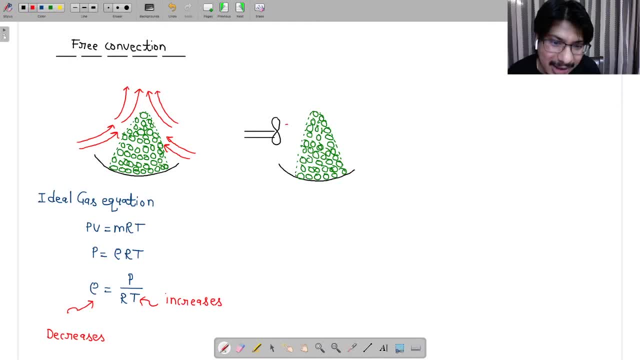 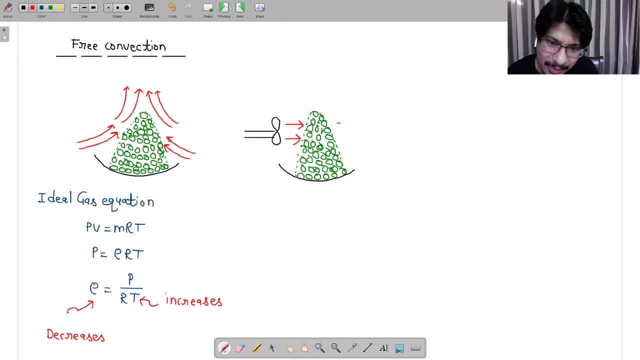 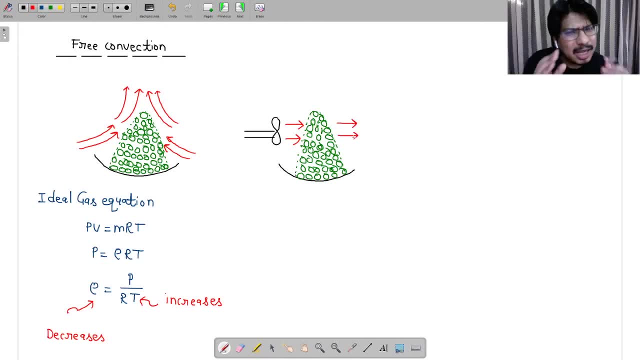 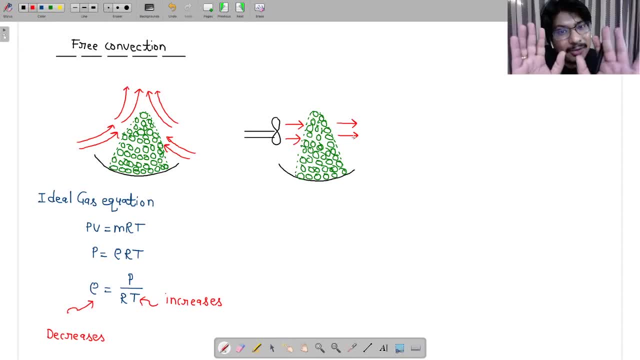 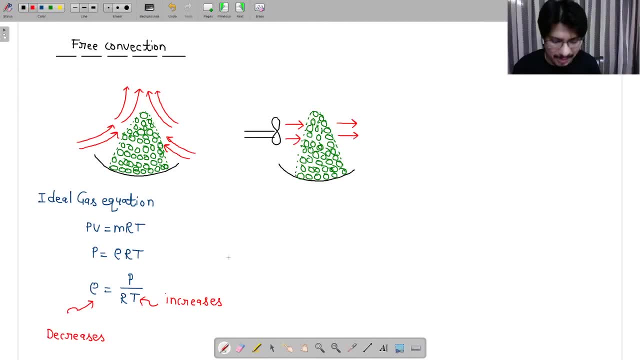 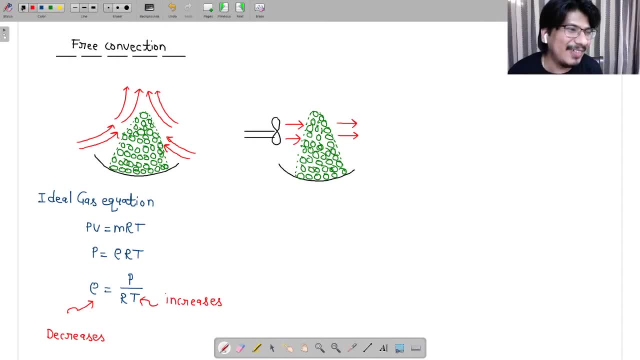 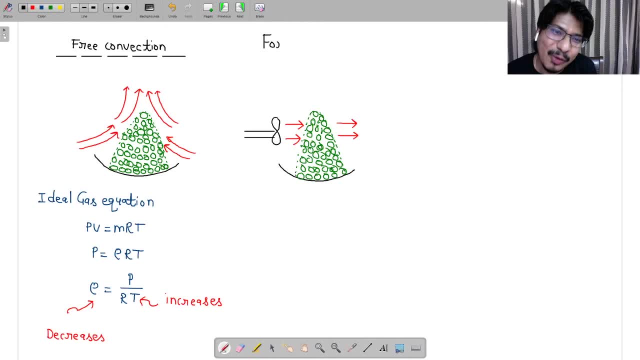 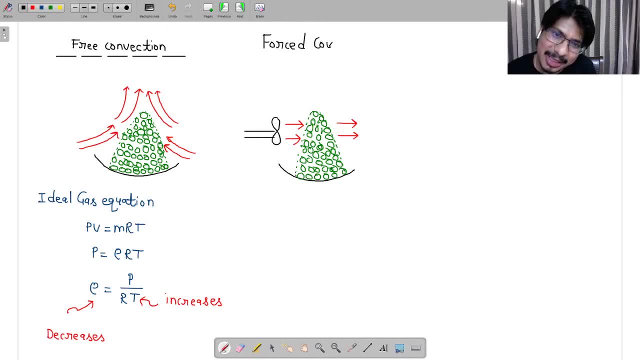 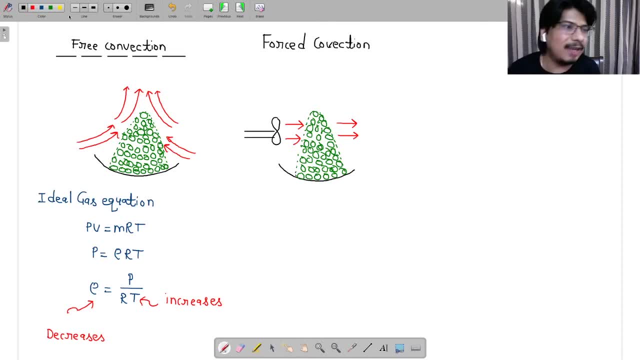 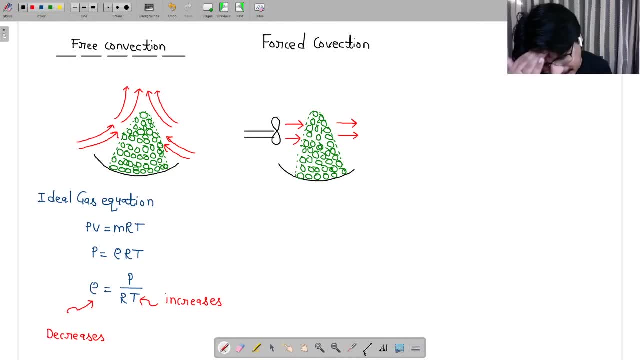 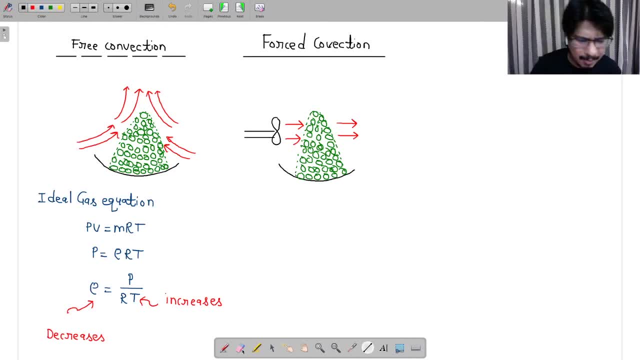 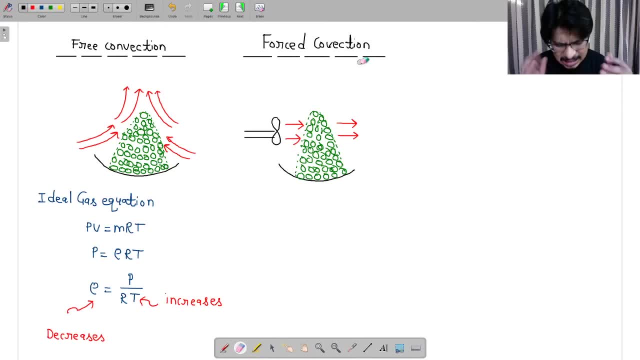 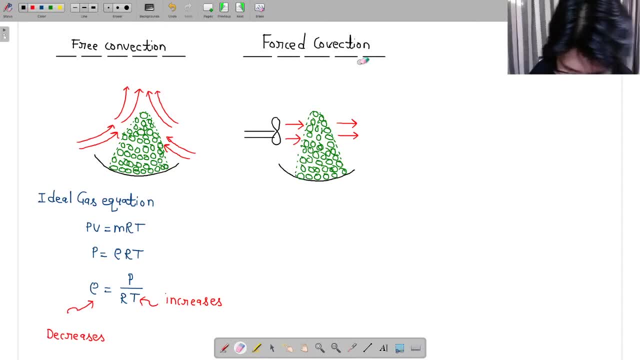 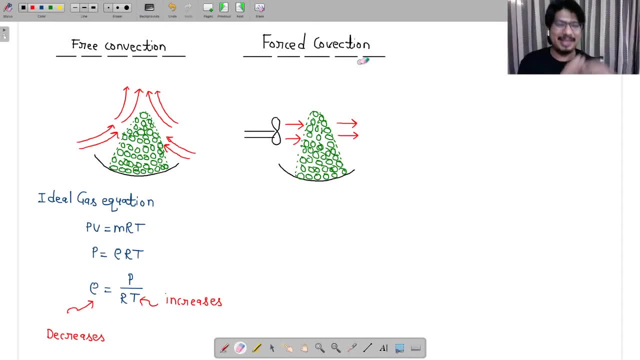 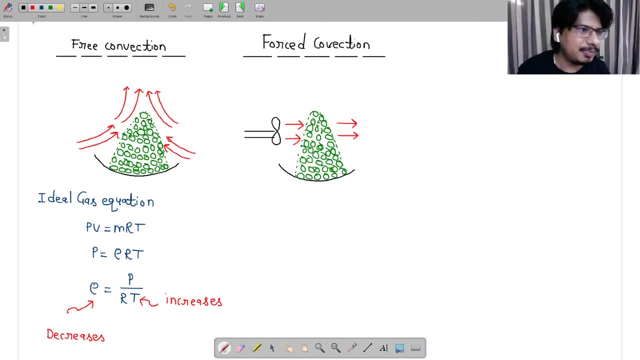 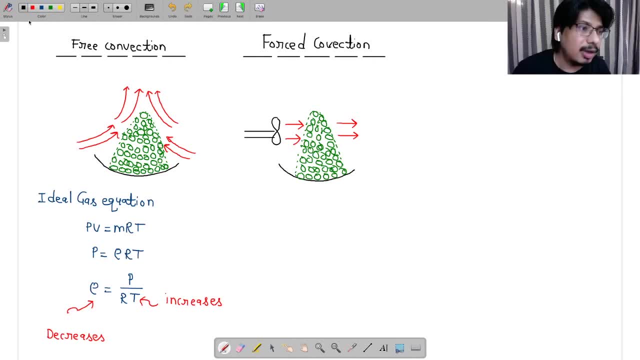 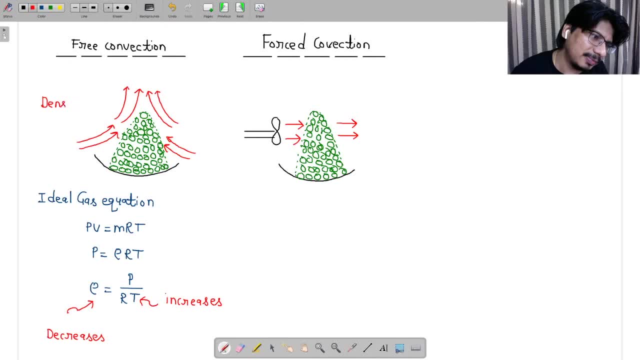 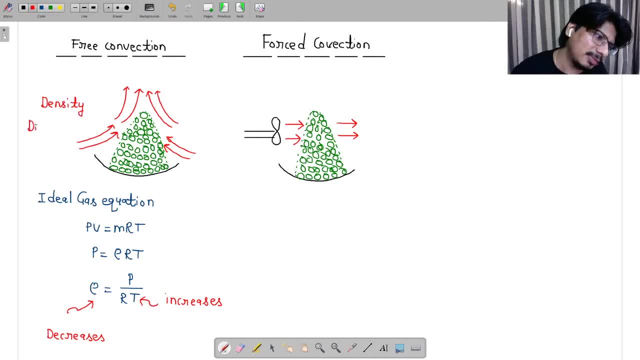 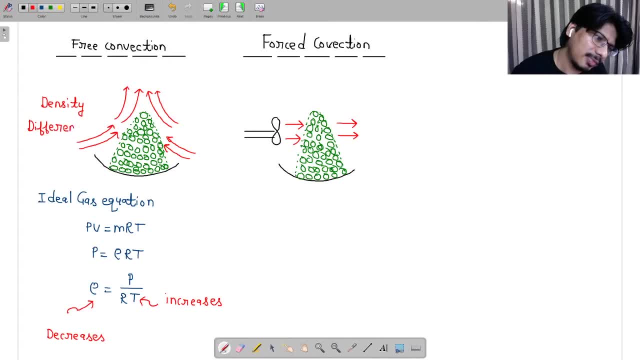 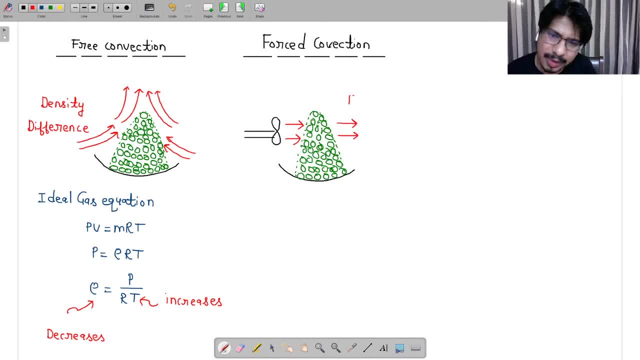 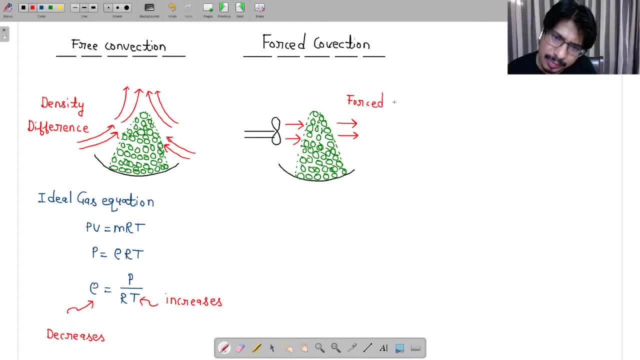 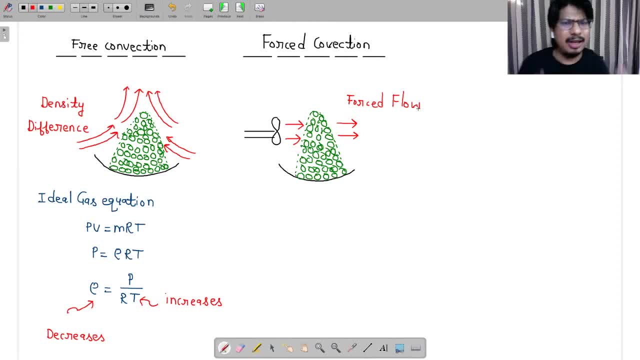 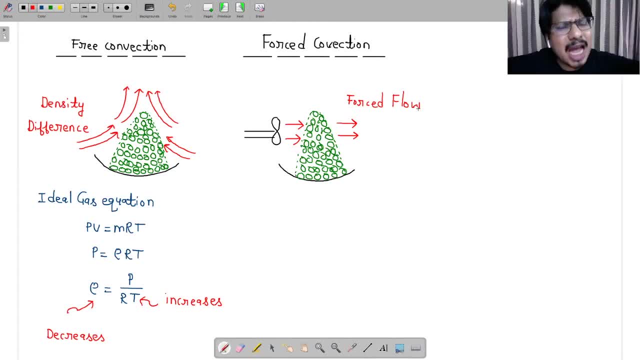 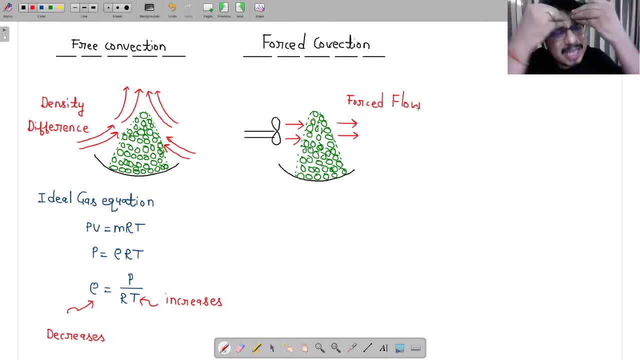 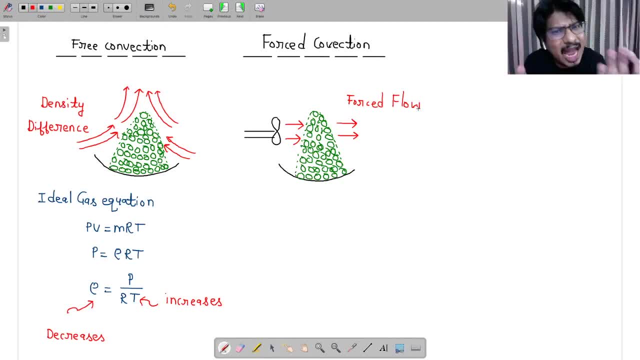 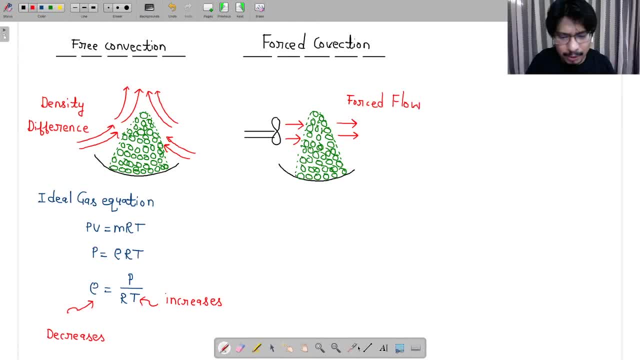 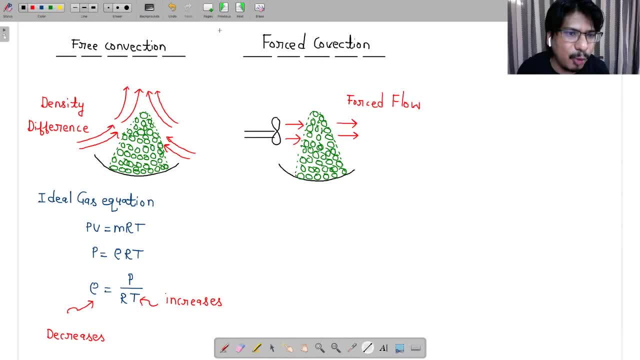 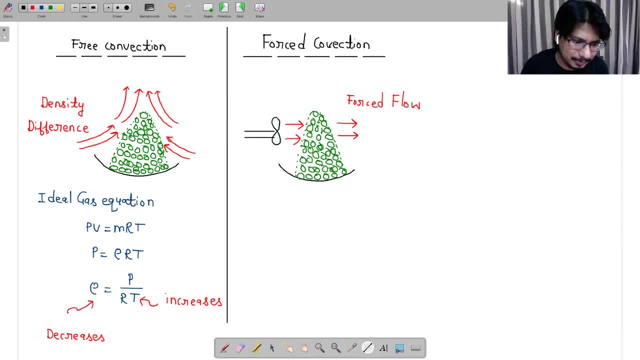 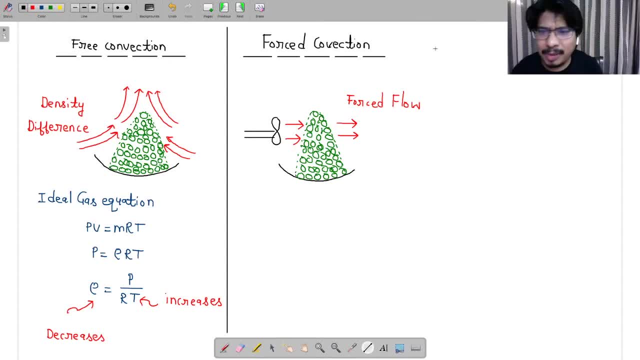 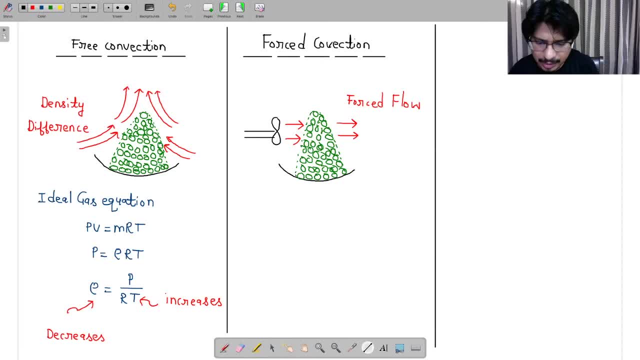 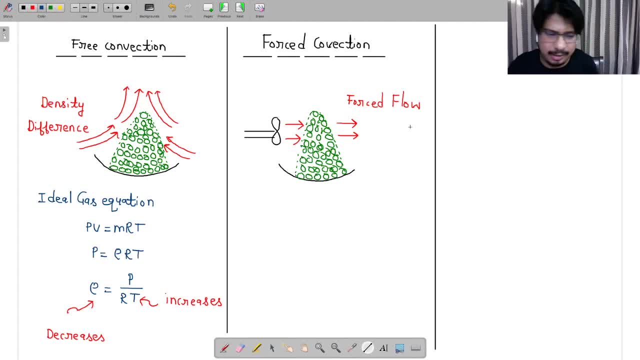 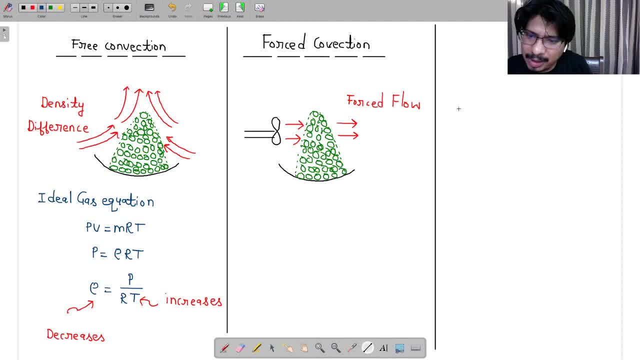 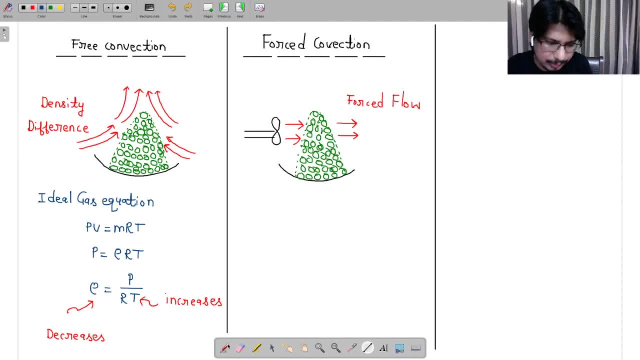 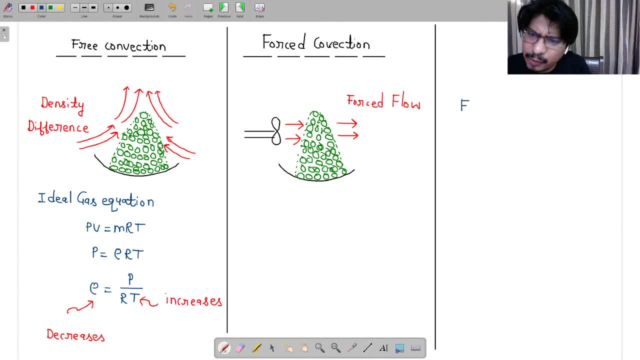 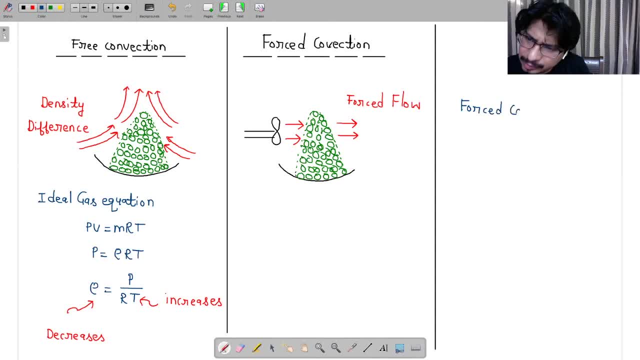 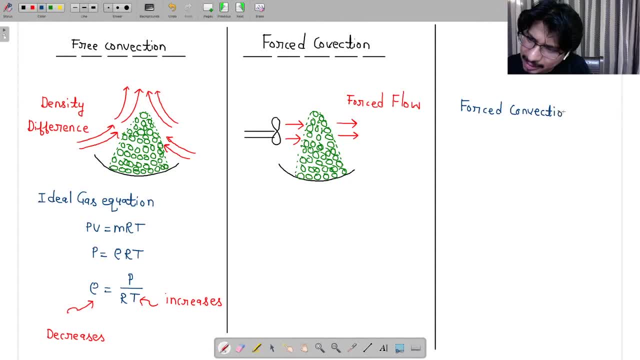 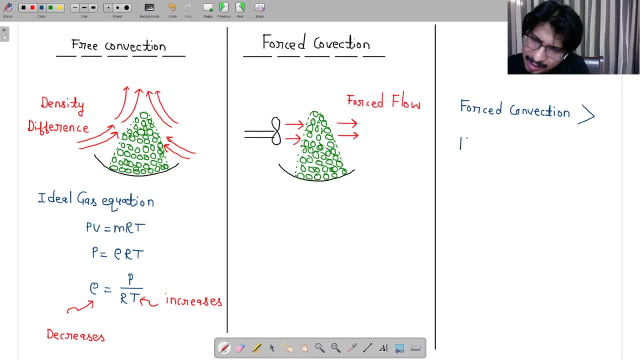 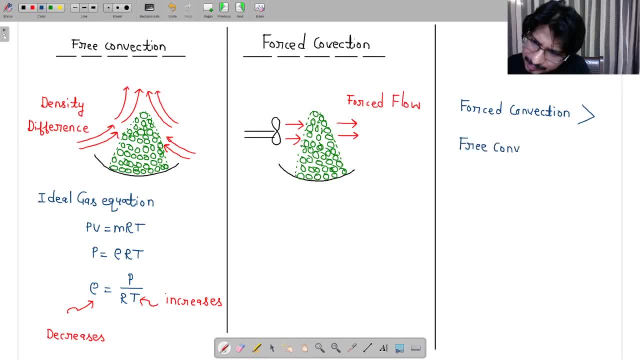 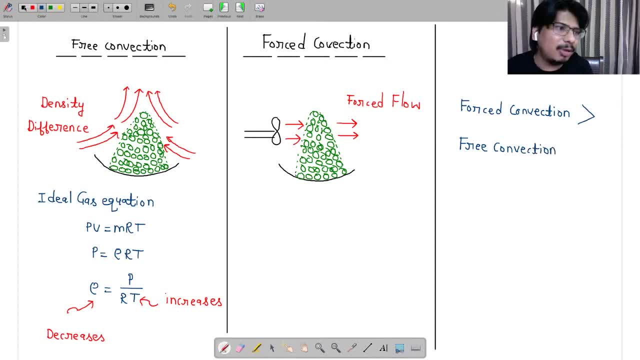 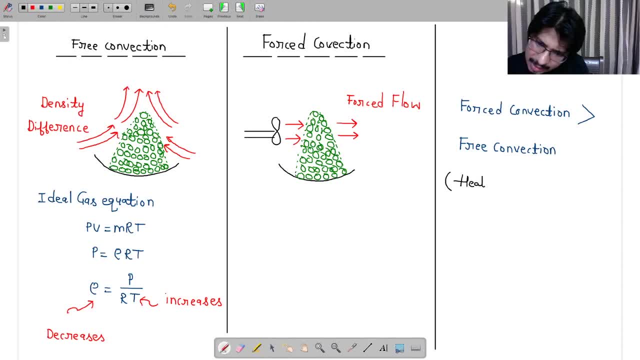 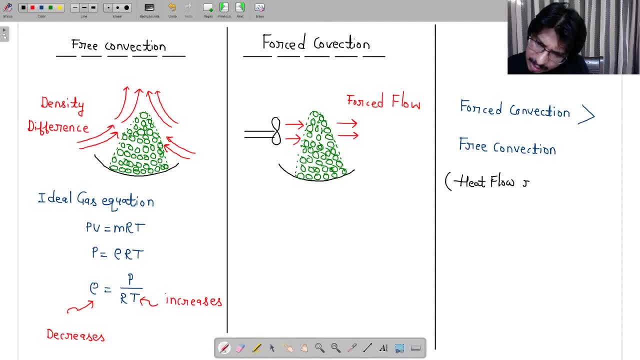 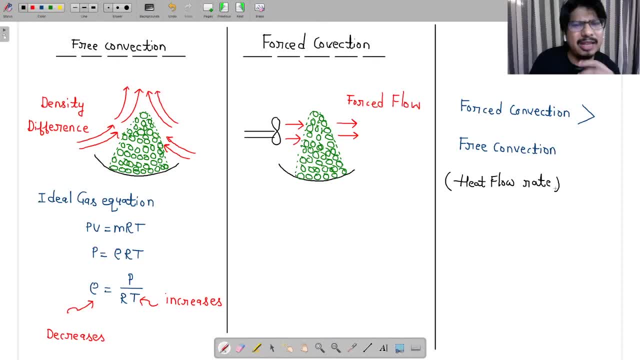 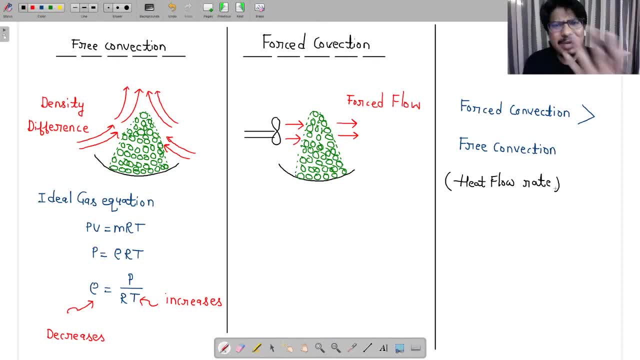 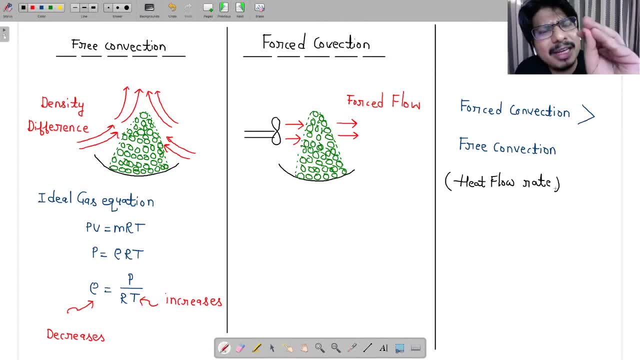 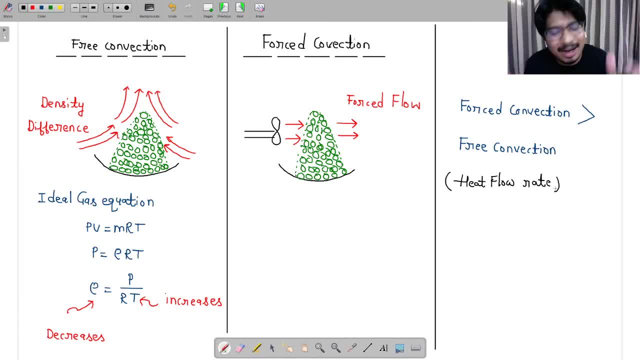 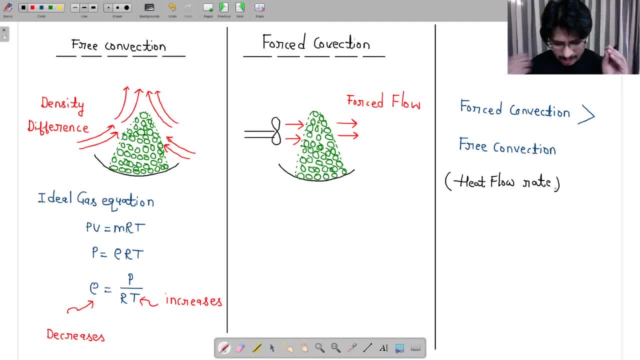 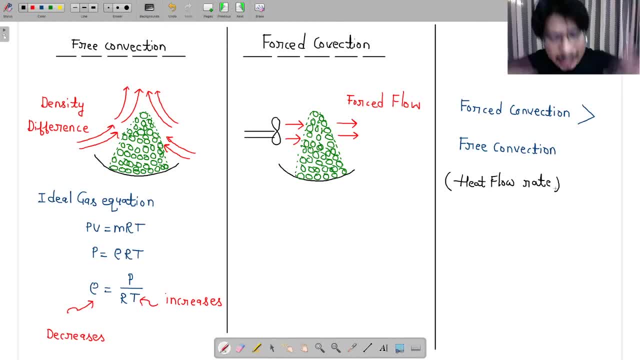 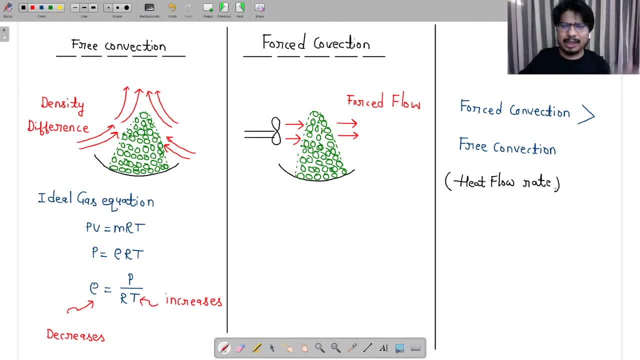 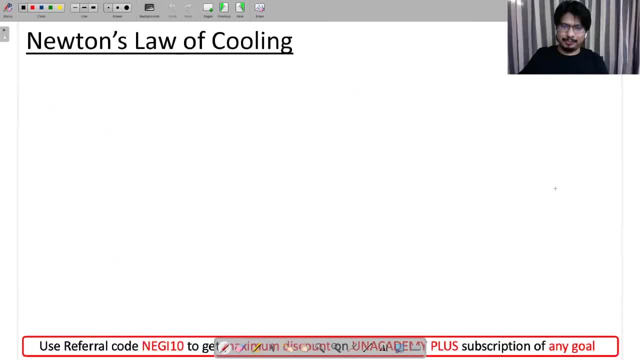 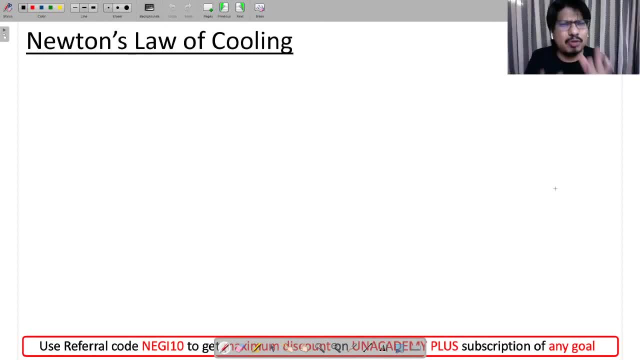 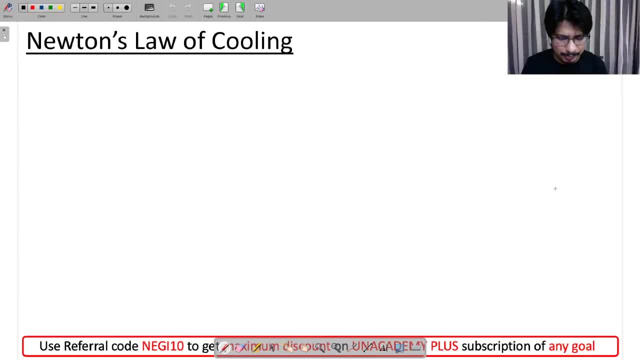 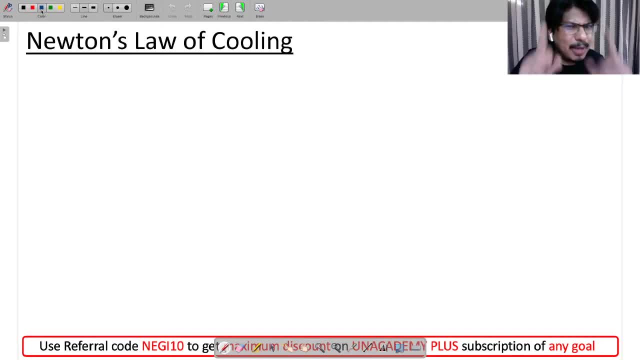 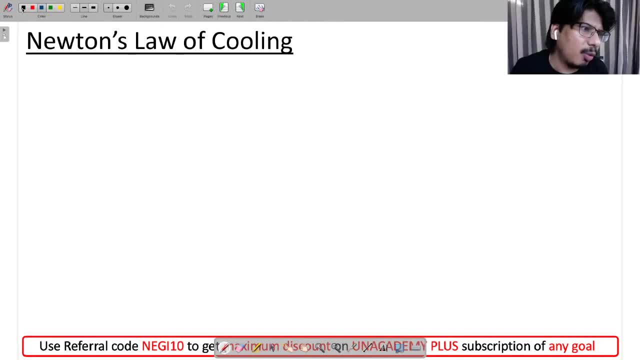 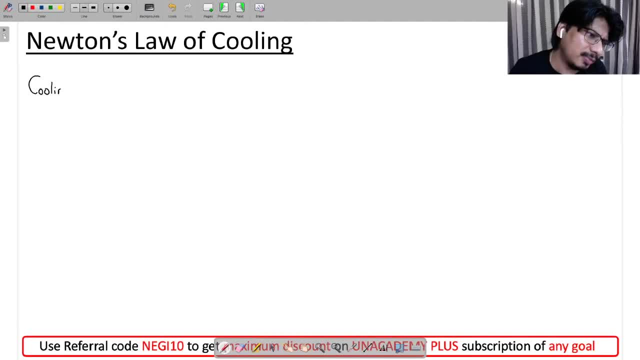 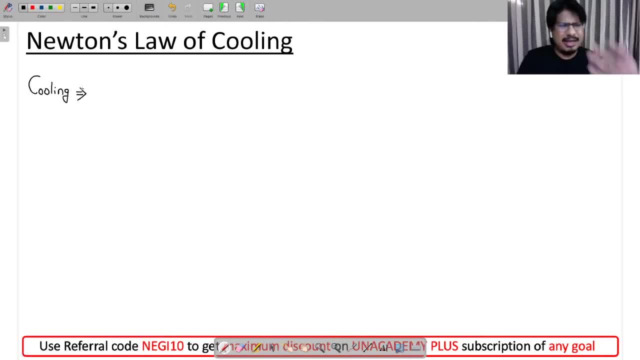 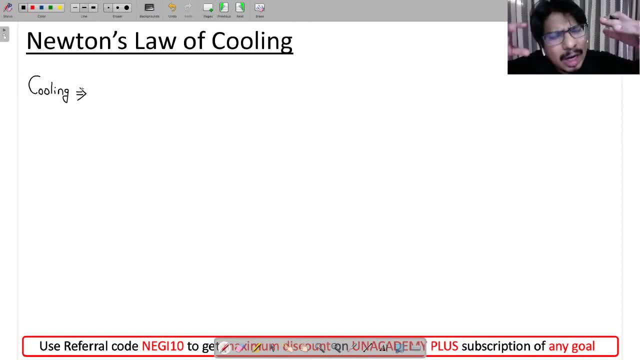 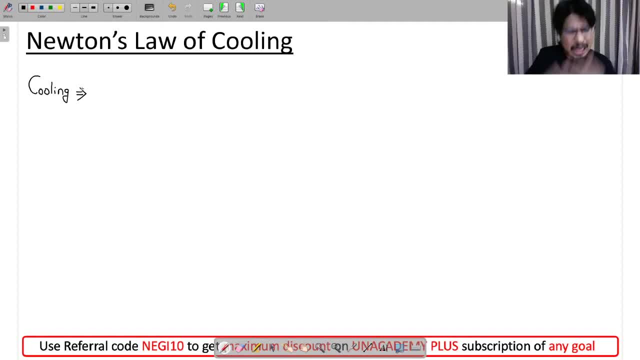 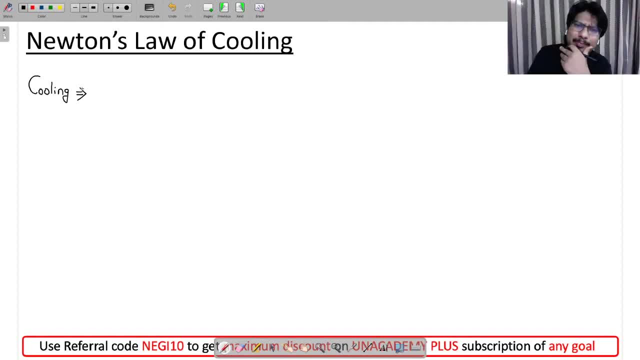 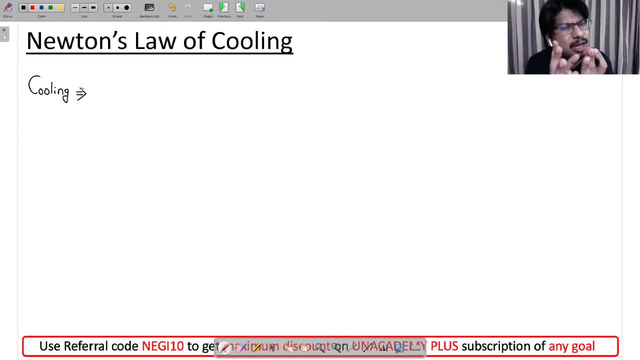 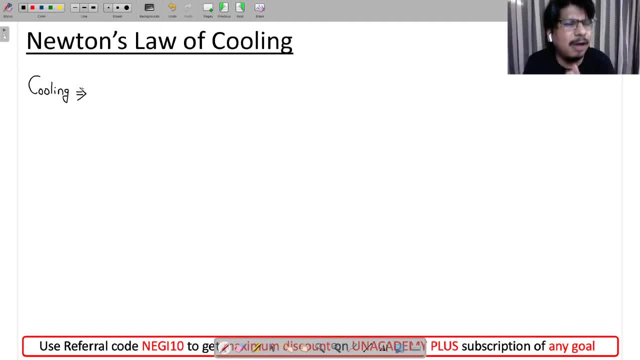 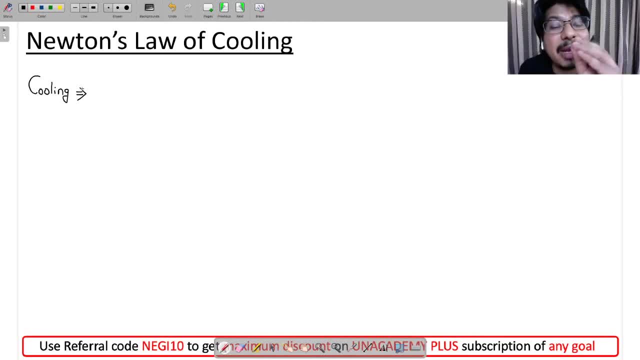 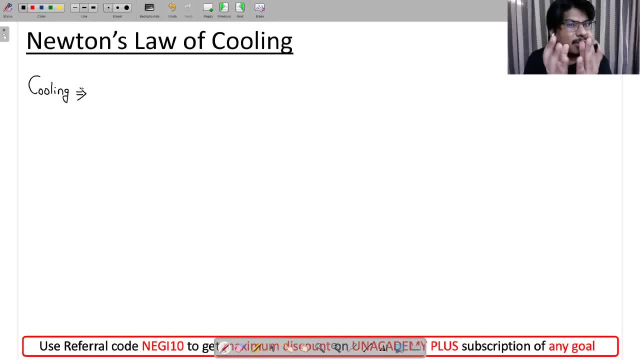 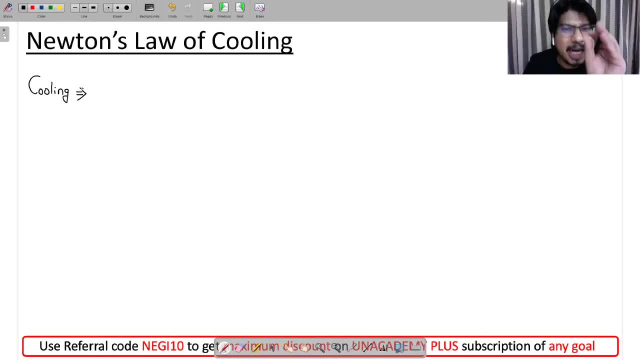 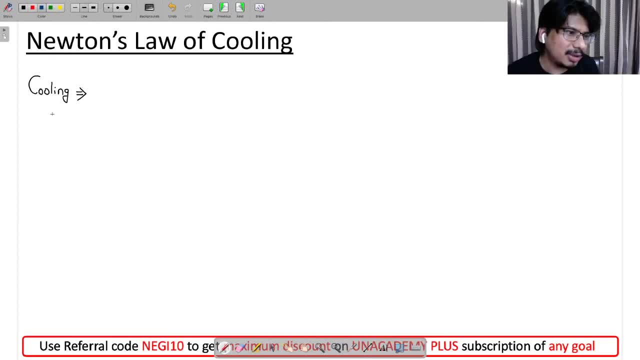 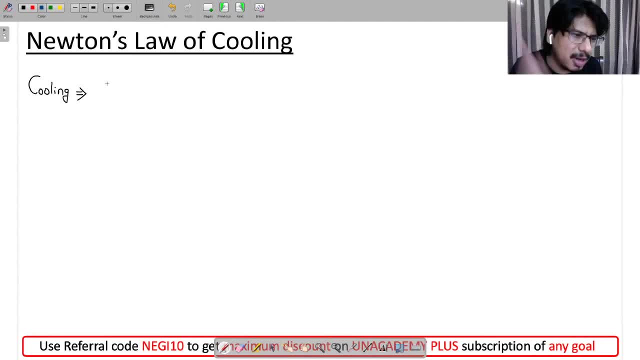 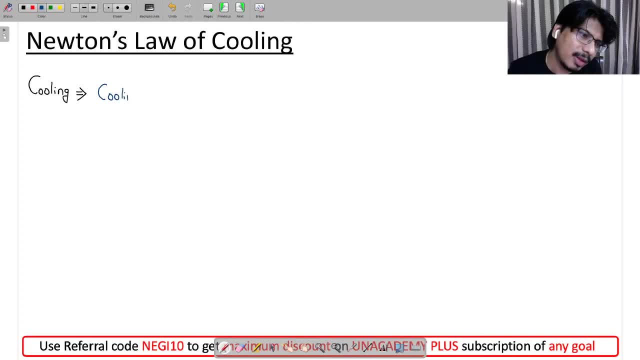 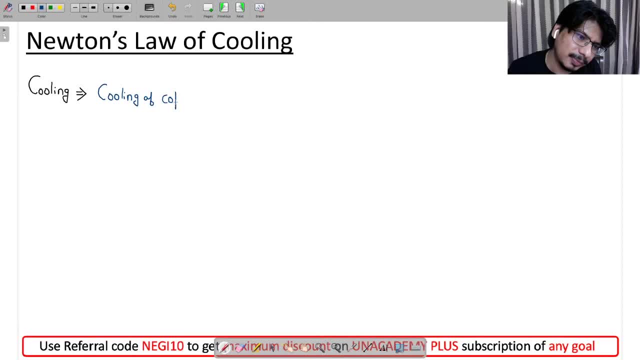 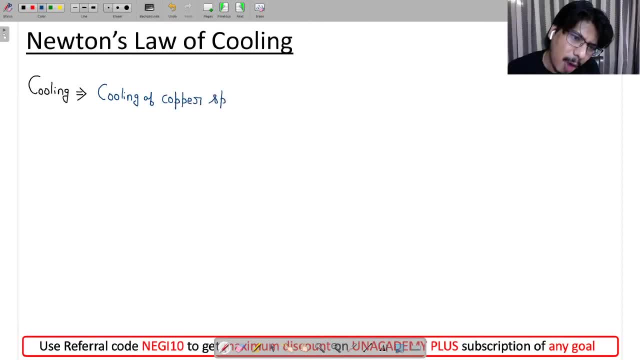 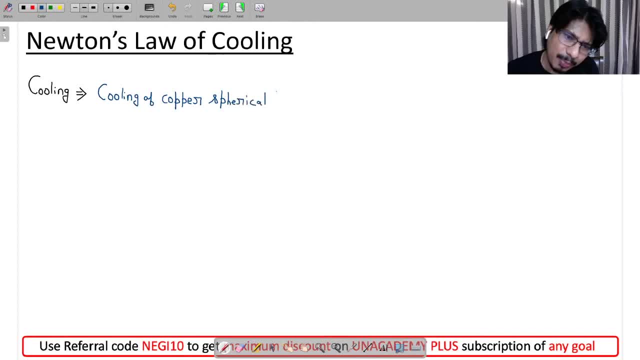 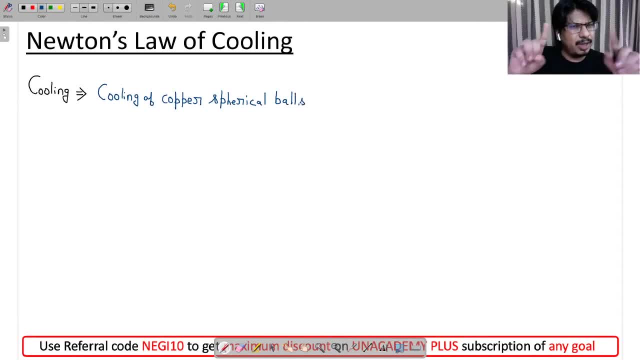 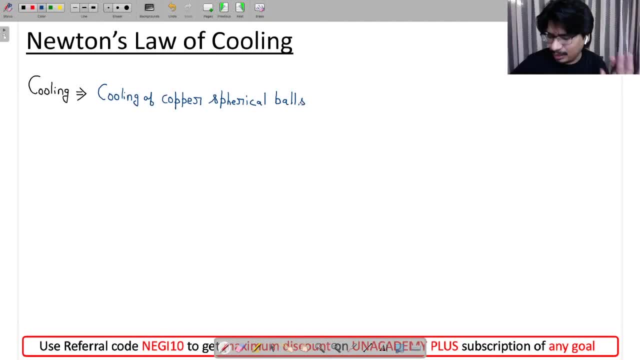 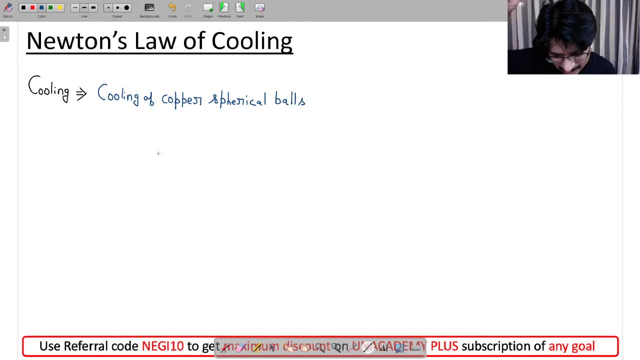 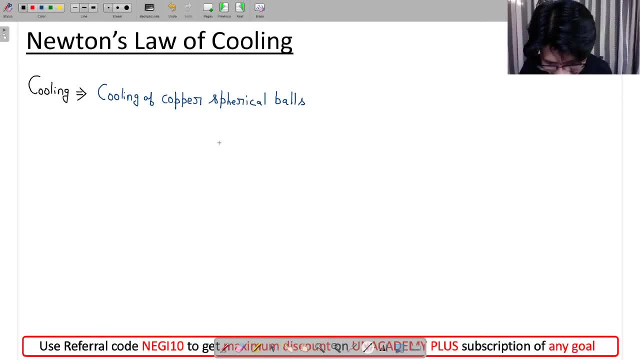 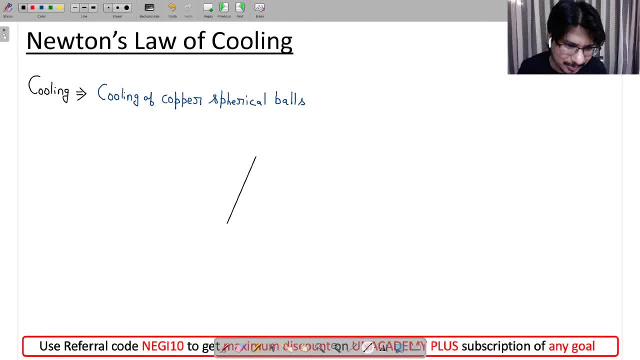 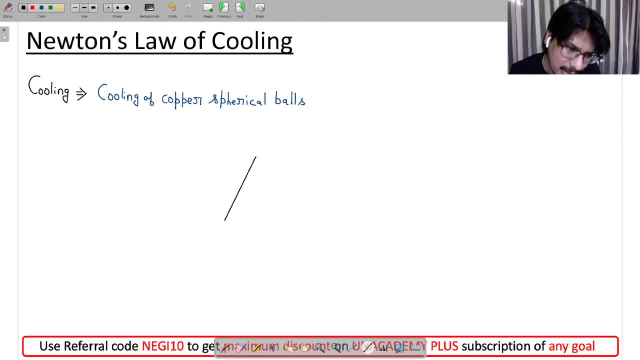 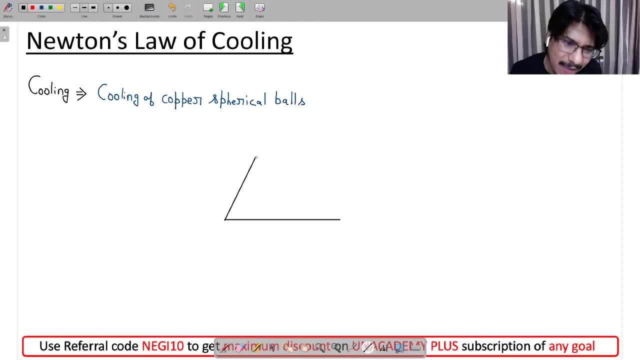 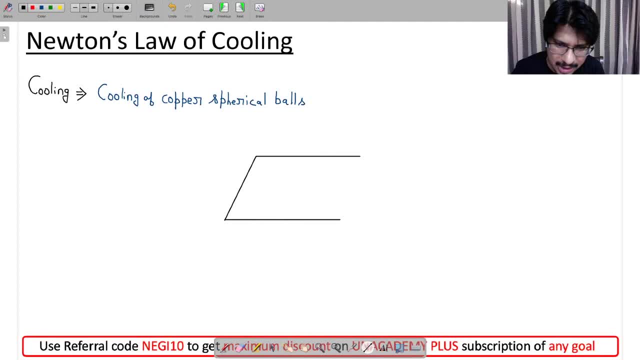 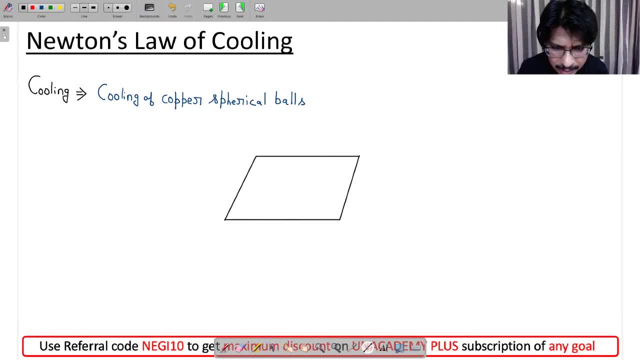 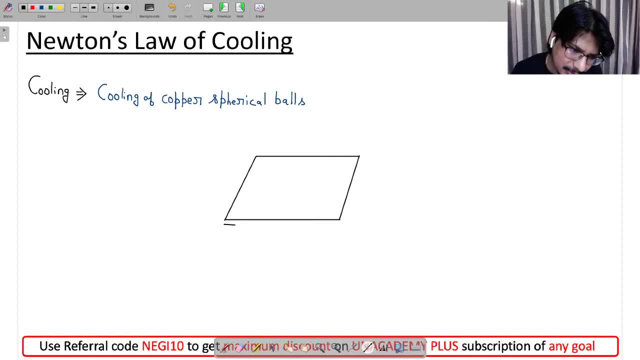 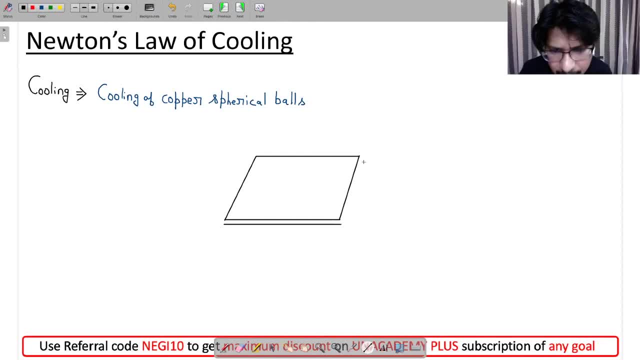 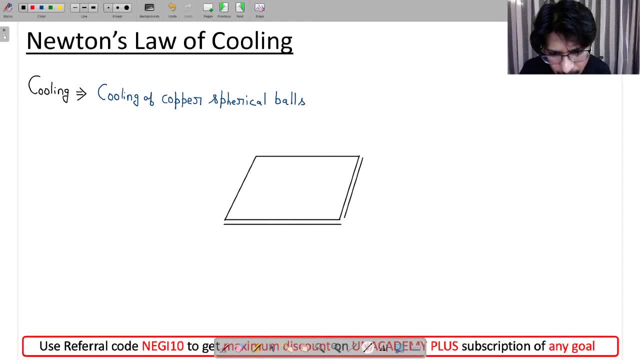 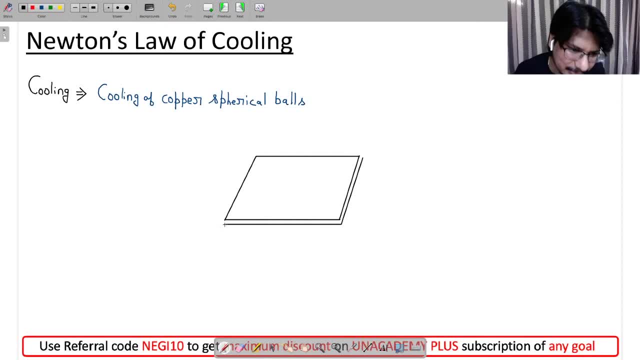 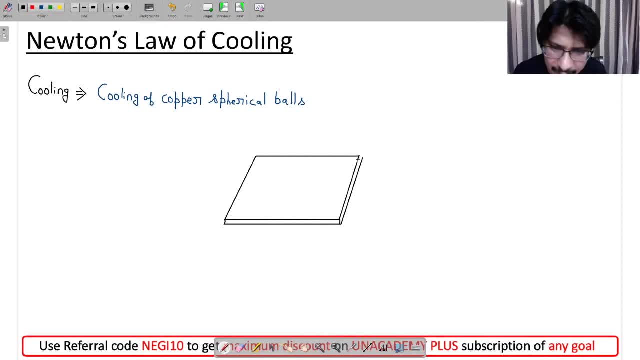 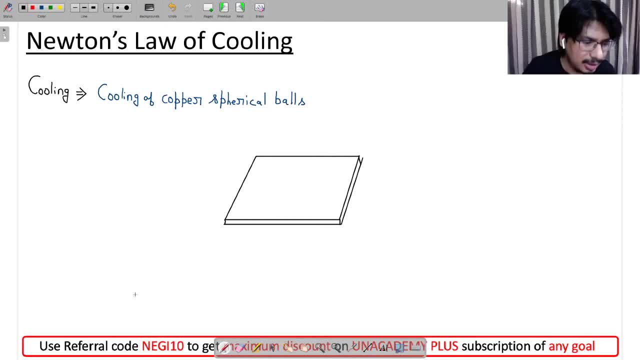 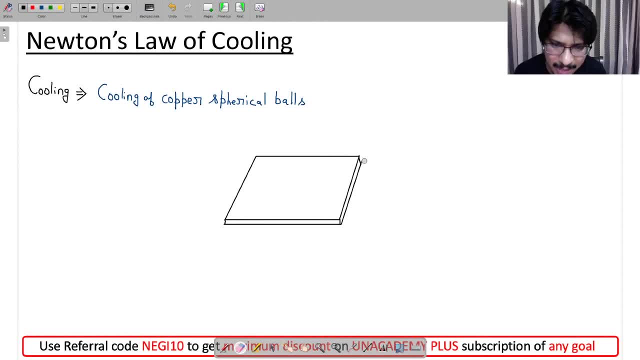 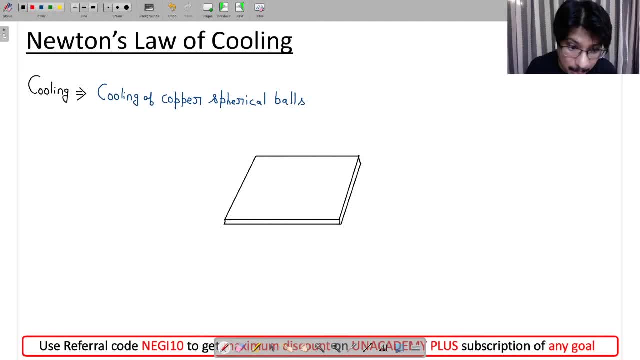 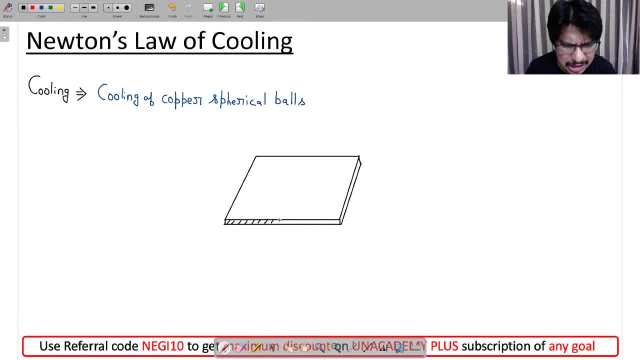 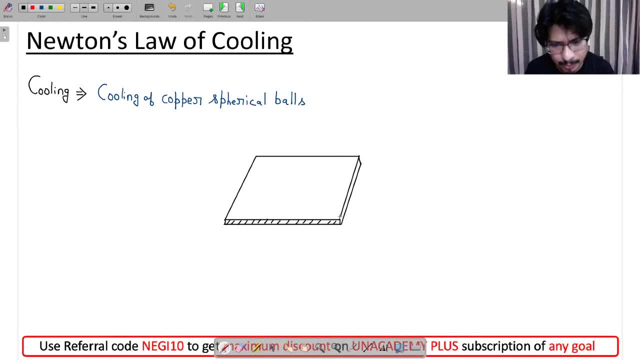 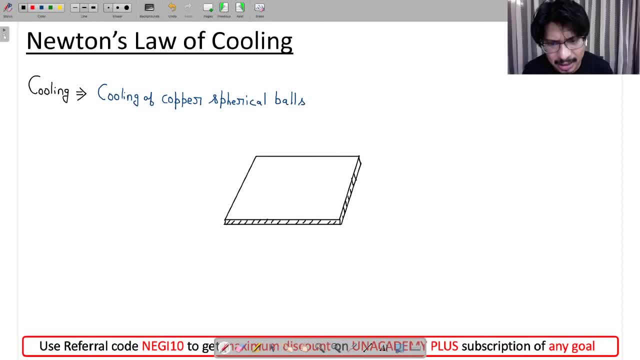 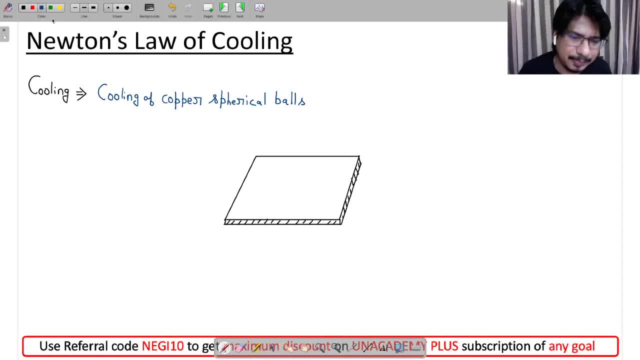 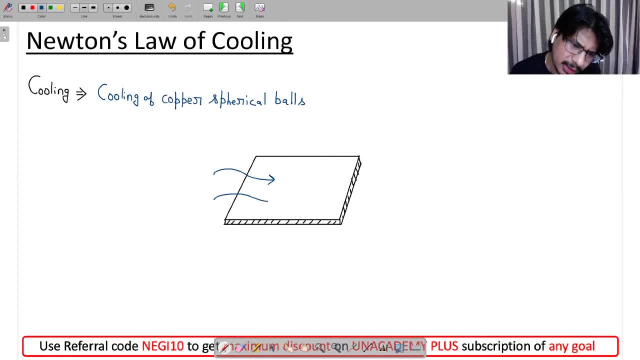 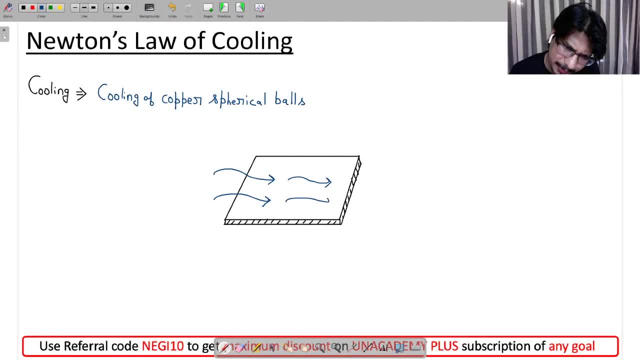 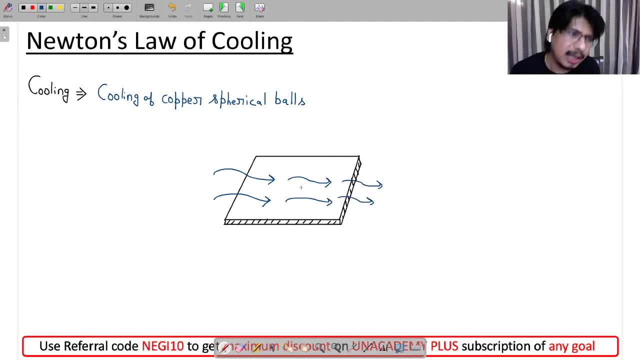 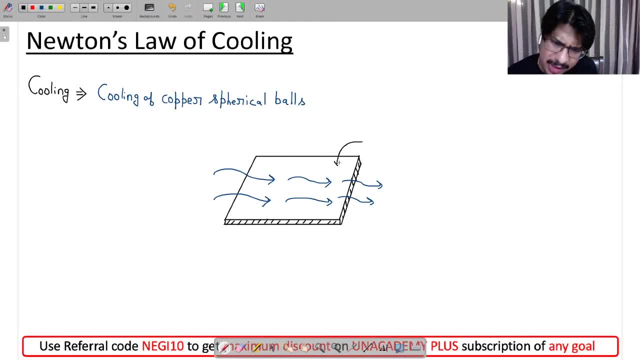 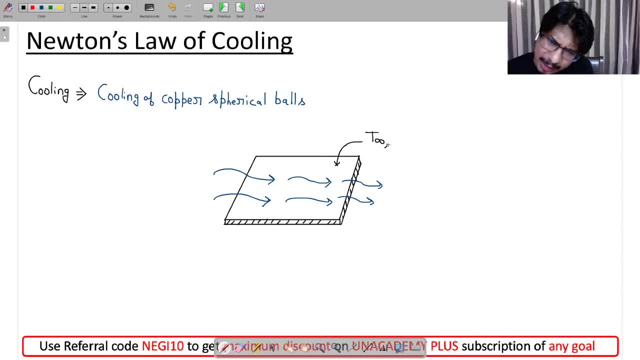 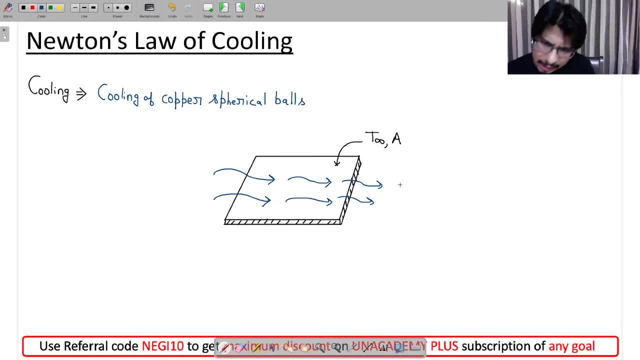 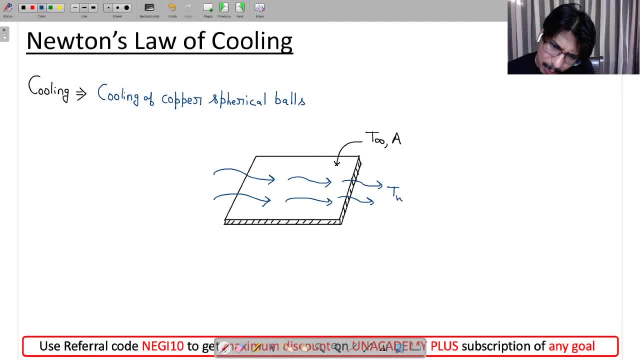 when someone is saying conduction, what comes in your mind? first thing, The temperature of the surface is Tw. Let us assume I am assuming, I am assuming. Let us observe carefully what I am saying. Let us assume Tw is more than Tn. 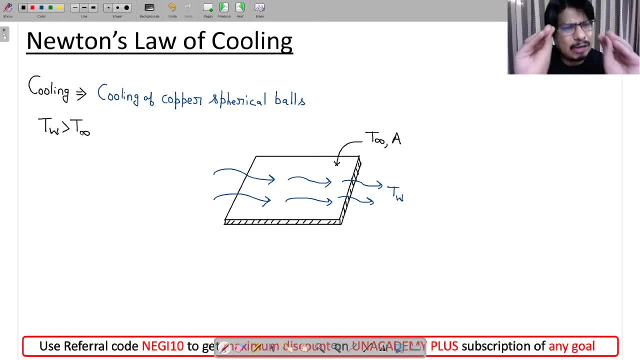 Now, if Tw is more than Tn, First of all, tell me what will be the mode of heat transfer. What will be the mode of heat transfer? It will be 100% convection. Why are you saying convection? Why are you saying convection? 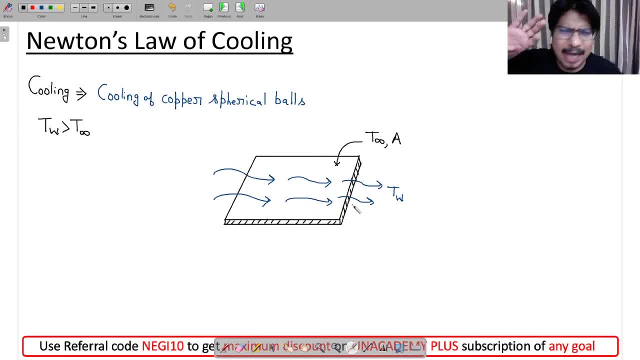 Because the fluid is flowing. There is some macroscopic bulk motion. There is some macroscopic bulk motion, 100%, It is convection. There is no doubt Now if the temperature Tw, This plate temperature, is more than the fluid temperature. 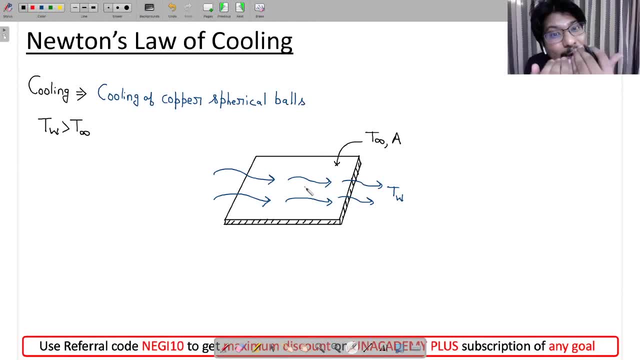 What will be the direction of heat flow? The heat will be flowing through convection, via convection, from the plate to the fluid. So look at here. Let me say this temperature difference is delta T. Let me say this is delta T. 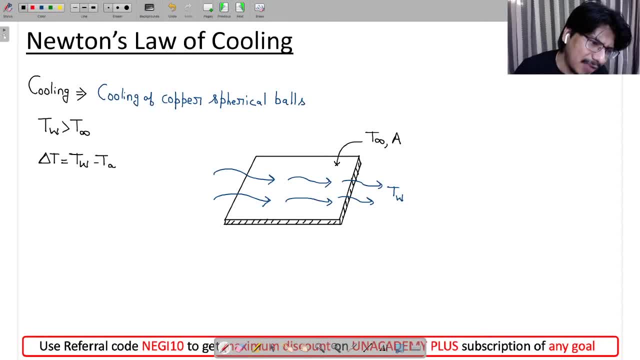 Tw minus T. This doesn't mean I can have reverse. also, If the fluid is having more temperature than the plate surface, then 100% heat transfer will be from fluid to the top surface of the plate by convection. So you have to remember this. 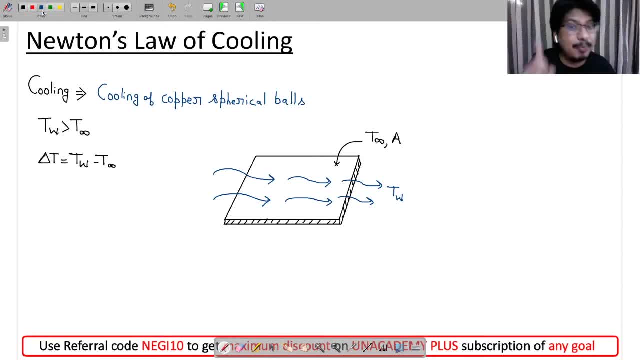 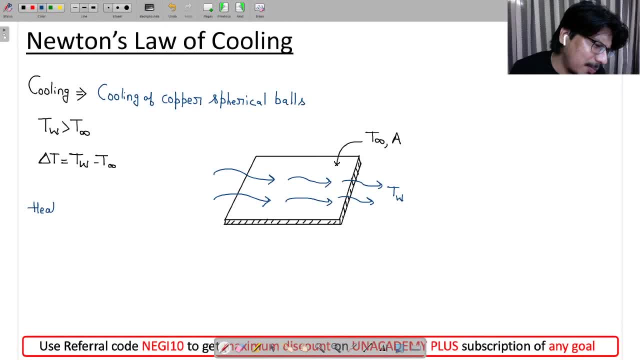 Look at this carefully. Look at this carefully. This is very important. This is very important. Heat flux conducted According to Newton's law of cooling heat flux conducted. Any intelligent student of the class can give me the answer. What will be the unit of heat flux? 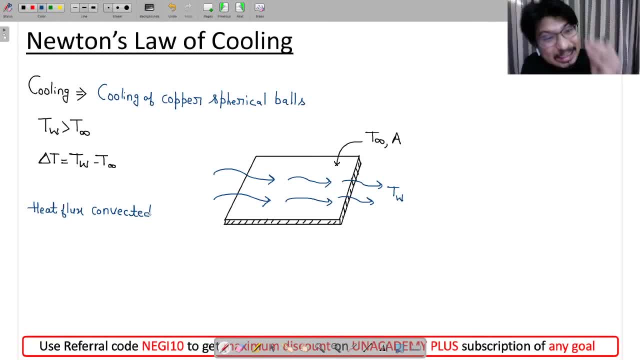 Tell me what will be the unit of heat flux. What unit of heat flux will be there? What will be the unit of heat flux? What will be the unit of heat flux? Heat: What will be the unit of heat flux, My friends, What will be the unit of heat flux? 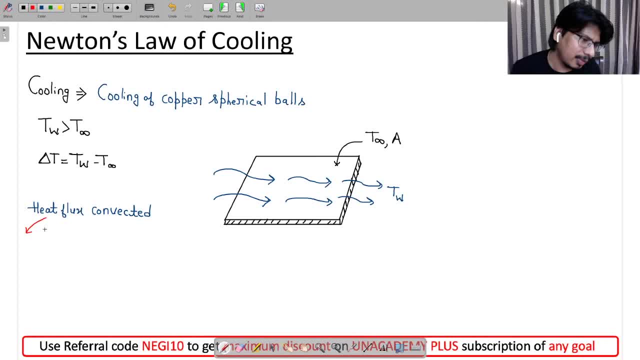 What will be the unit of heat flux? No, What is wrong, Naseem? what is wrong? Yes, Yes, Yes, Yes, Yes, Yes, Yes. Excellent. Flux means per unit area. So heat flux, Convected heat flux unit, will be Watt per meter. My friends, please take it positively, Remember heat flux means watt per meter square. 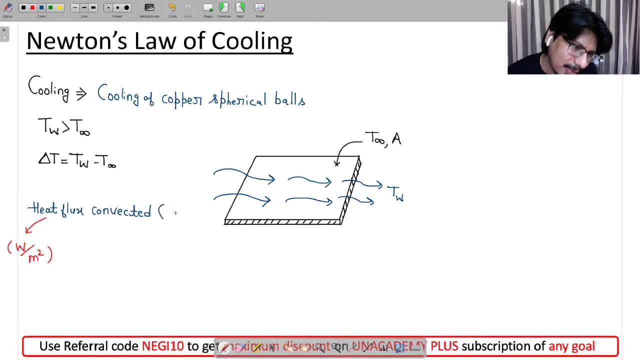 So heat flux Convected Q dot, This will be Equal to Newton's law of cooling. This will be directly proportional to. It will be directly proportional to Temperature difference. This will be directly proportional to Temperature difference. What does temperature difference mean? Delta T: What is the meaning of temperature difference? 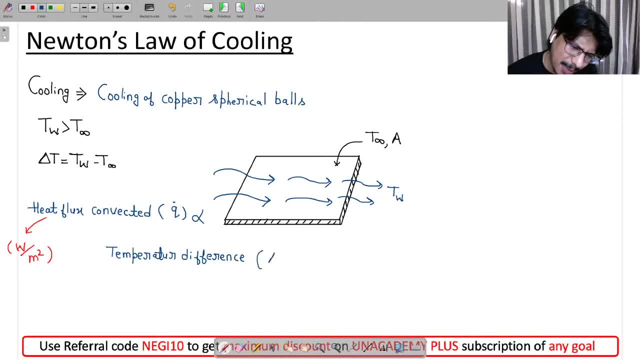 Delta T. Those who are online Press the like button. Why are you shy to hit like? Why are you shy to hit like? Don't be shy at all. Come to my class, Press like, without hesitation, Full effort, Full freedom. Press like. I have given you full freedom, Enjoy it. 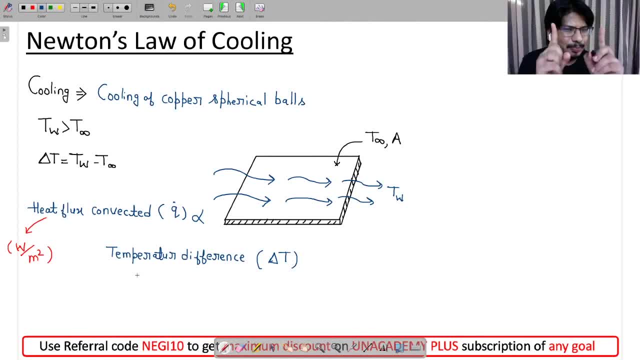 Each and every moment you enjoy. Come on Now, look, Whenever it is directly proportional, So we will remove it. The moment I will remove this directly proportional, Something will come And this is your HX. What is this HX is Now? look, Listen carefully. I am telling you a very important thing. 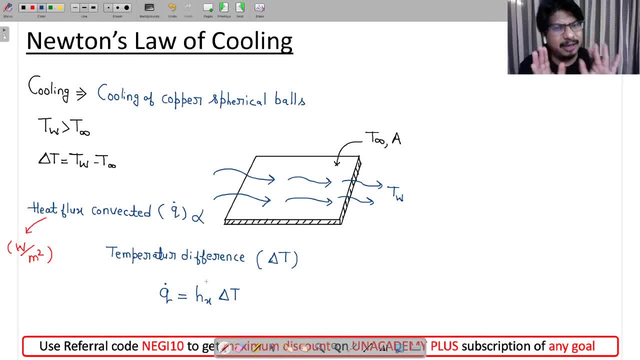 Heat flux Convected will be equal to HX delta T. Keep a crystal clear concept. For example, See what I mean to tell you. Please listen carefully. Please listen carefully. Let me say I want to find heat flux In this small area. DA, We will see carefully, We will understand things very well. 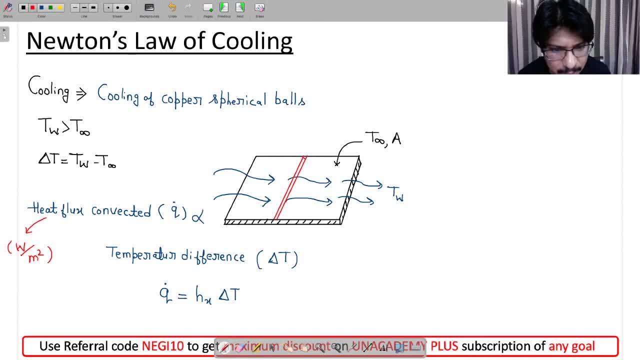 What I am saying is absolutely fine. Please listen carefully. Let us suppose this is a small area DA Where I want to find What is heat flux. getting convicted Now listen carefully. Let me say here: The heat transfer coefficient is HX, Heat transfer coefficient is HX, So heat flux here will be. 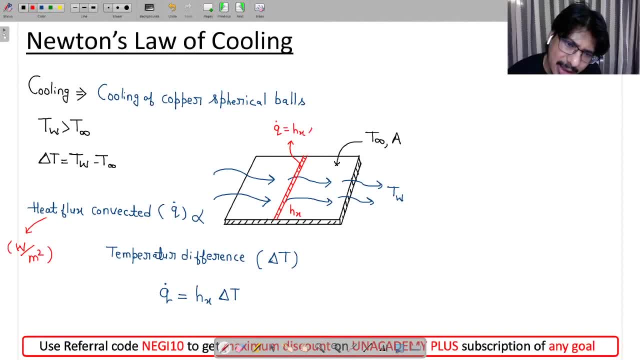 HX into delta T. Abhi main aya par HX into delta T. Abhi main aya par HX into delta T. what is the meaning of writing x? listen carefully. you people do so many mistakes, so remove your bad concept. why i'm writing this x over here? because heat, this heat transfer coefficient, is not 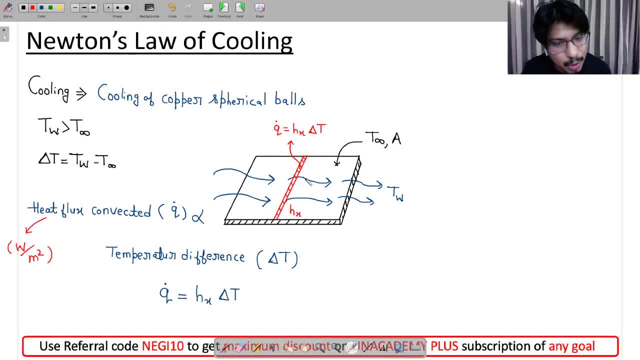 constant. it is not constant. it is going to change as the distance from the leading edge changes. whatever is this edge, this is leading edge, this is the trailing edge, as the distance from the leading edge, as the x distance. please try to understand what i'm saying. this is: 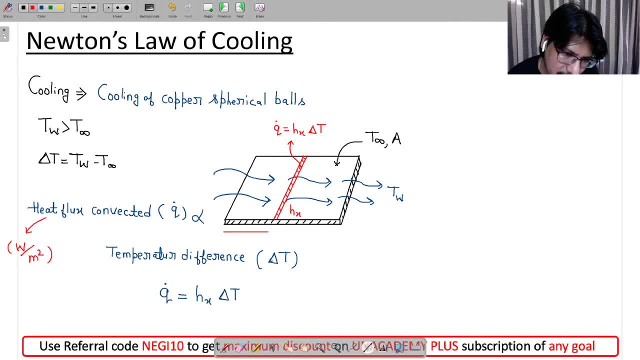 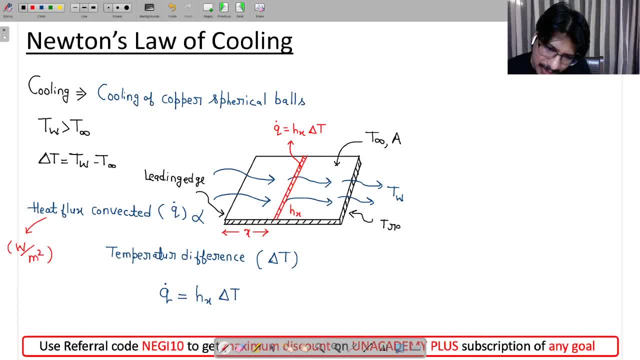 known as trailing edge. remember, Come back. i have wrote the training. ok, listen carefully. you have to write for the entire area. now say'm, cannot you tell me what will be the heat convicted from the entire area? entire area, this entire area. how much heat is getting convected from here? tell me this. 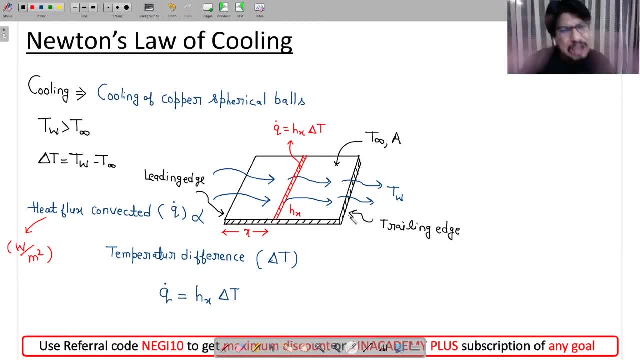 I am not in such a small area. I want to find from the whole plate for a whole plate, how much is the rate of heat getting convected. so I will tell you about that too. now listen carefully. what will happen there. I will be telling you. please observe, please observe. 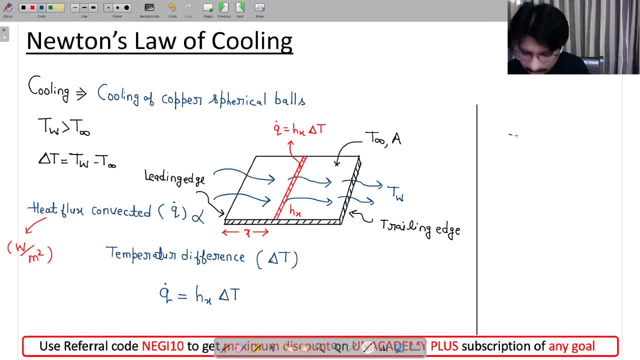 please observe, see what will happen. heat flow rate getting convected from the whole plate will be H bar A, delta T, delta T. you know what is delta T. you know, there is no doubt what is delta T. everyone knows what is A, you know. A is the area of this plate. 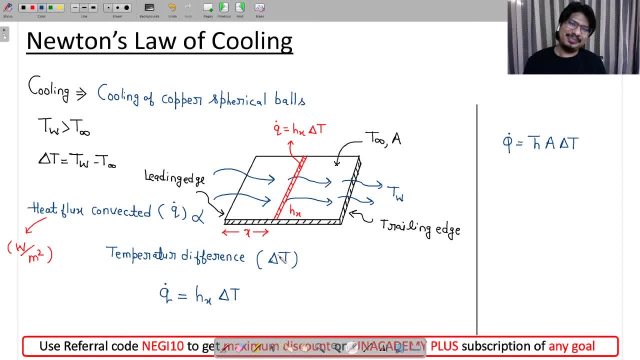 surface area of this plate. What is H bar? what is H bar? what a beauty, what a beauty, what a beauty. see this H x was local heat transfer coefficient. local heat transfer coefficient, excellent, excellent, excellent students. And this H bar is what 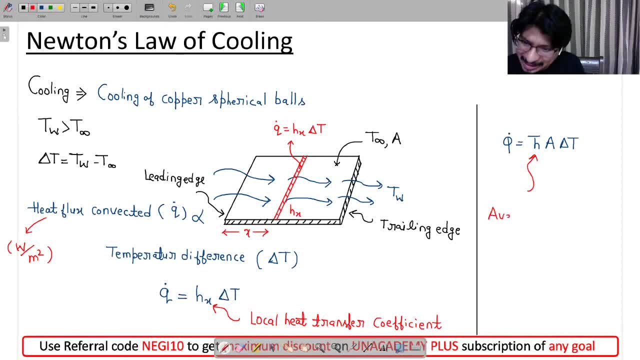 H bar is what H bar is what Average heat transfer coefficient? Dekho, I will be telling you, kya hai difference. mai aapko bilkul simple language mein samjhata hoon. I will be telling you in very simple language. 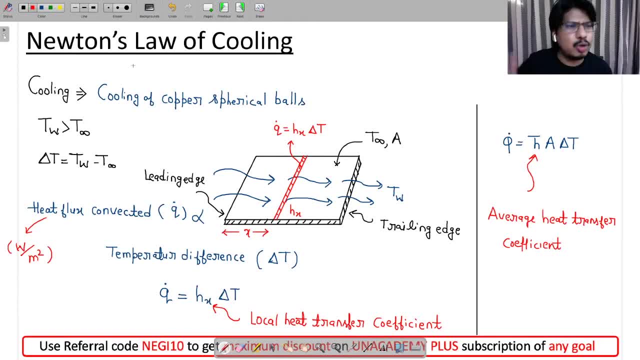 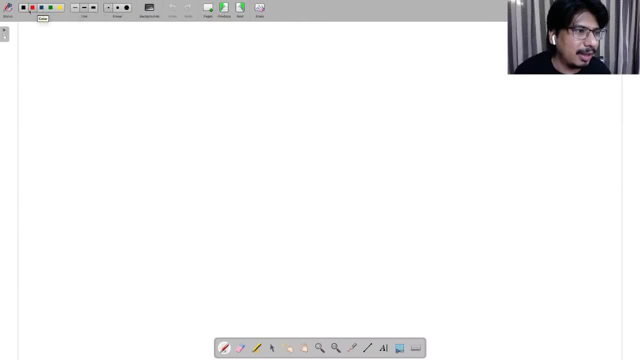 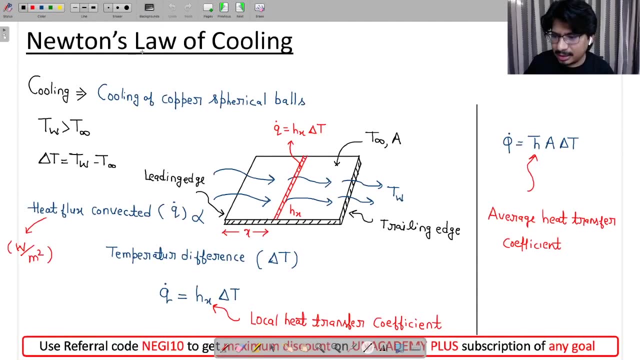 Dekho. those who are not able to understand what is the difference. I will be telling you in very simple language. listen carefully, Look at here, look at here, abbilkul. simple language in very simple language. yes, yes. 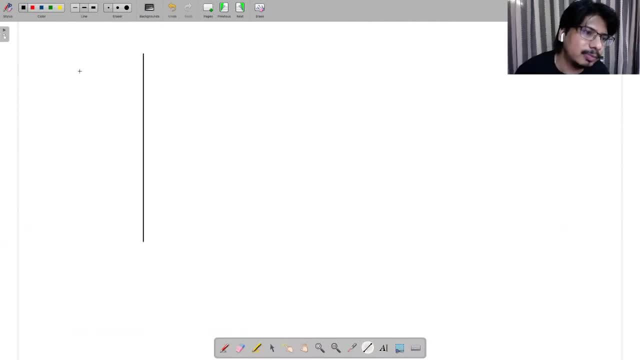 in very simple language, I will be telling you. dekho Chalo, look at here. let me write the year also. year likh lete hain maal leje 2018, 2019, or, it is very dangerous, year 2020 ka. kya ho gaya, re baba? I don't understand. very dangerous. 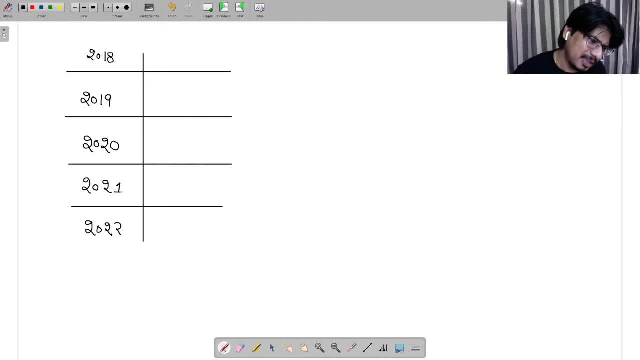 very dangerous. Chalo, Chalo, Chalo, Chalo. Now listen carefully. Let us suppose 2018, our Prithampyare, our Prithampyare, let me say in 2018, our Prithampyare. 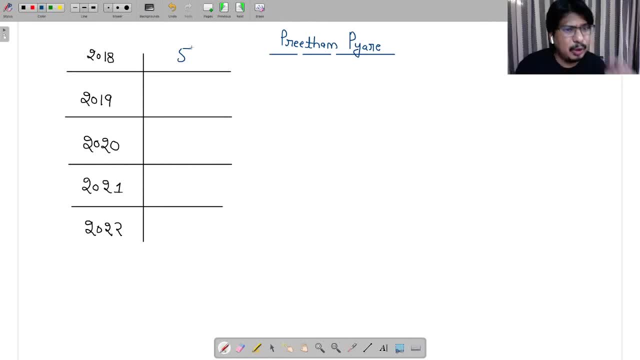 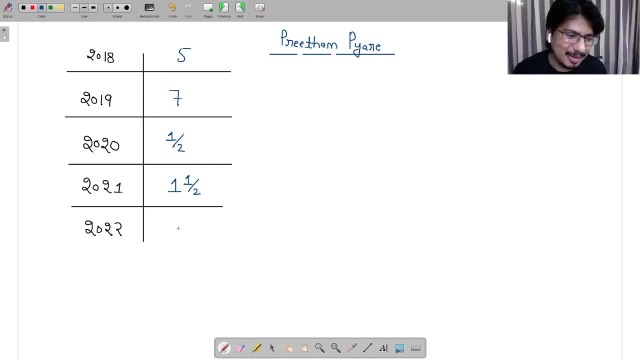 Now look, if I ask you, if I ask you in 2020, how many girlfriends Prithampyare is having, You will be saying this. So this is basically a cheques at a particular location, At a particular location. 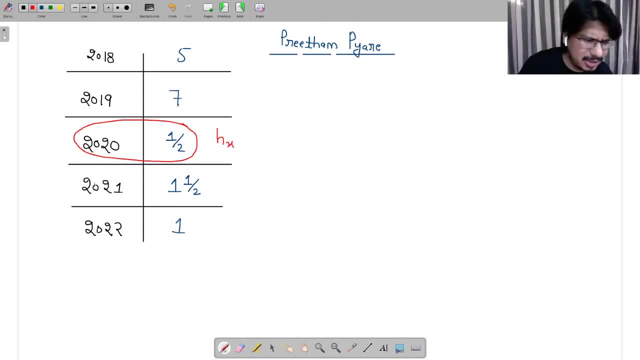 In 2018, this was a cheques. 2019, this is a cheques, this is a cheques. So at a particular location, if you are defining, you will be having the local heat transfer coefficient. But if I ask you Prithampyare, no problem. maybe in 2020 you are having half girlfriend, doesn't matter. 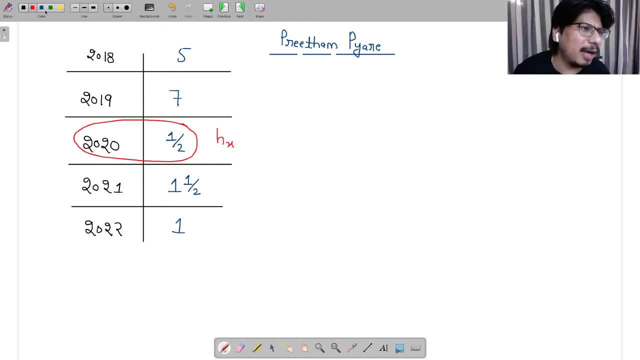 On average you are having how many girlfriends. So let us try to find out the average of Prithampyare- Average. how much is the average of Prithampyare? Tell me how much is the average. Average is how much. 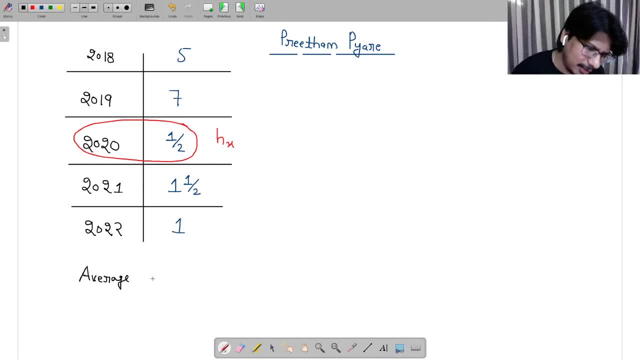 5 plus 7, 12, 12, 12 and 3, 15, right 15 divided by how many years? 5 years, Well done, well done Being a mechanical engineer. having this average is extraordinary. 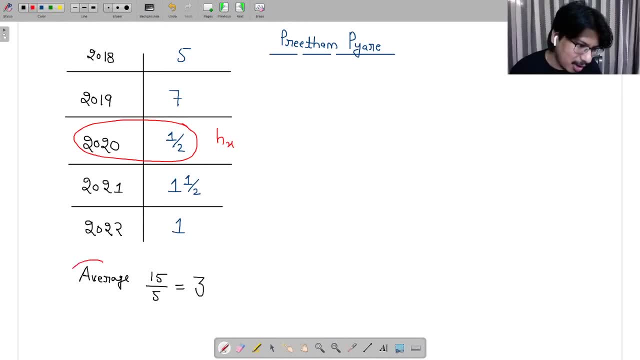 So this is your, this is your average heat transfer coefficient. Is it clear to everyone? Yes, yes, yes, Yes. So are you clear now? Has everyone understood Everyone is clear now. What is HX? what is H bar? 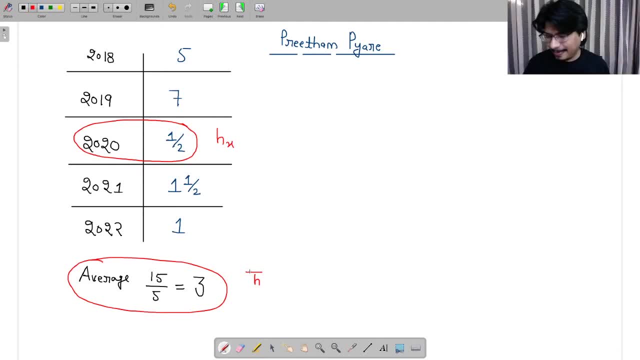 Everyone is clear. Tell me, tell me, Okay, okay Now. excellent student, excellent student. Now look carefully, carefully, carefully, carefully. come back, come back, come back. Yes, Sometimes they are asking in interviews what is the meaning of film conductivity? 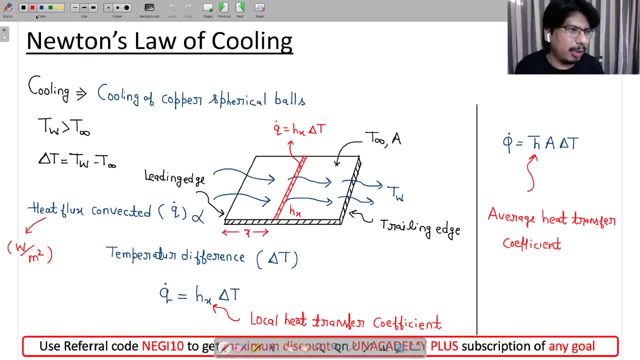 Sometimes they ask in the interview what is the meaning of film conductivity? So remember, please remember. this average heat transfer coefficient is also known as film conductivity. This average heat transfer coefficient is also known as film conductivity. Okay, okay, Look at here. 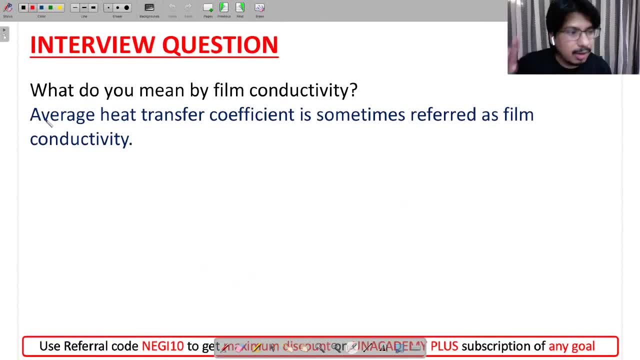 One interview question I am reading for you. What do you mean by film conductivity? Average heat transfer coefficient is sometimes referred as film conductivity. Sometimes the average heat transfer coefficient is in the mood of Pritam Pyare, so he also calls it film conductivity. 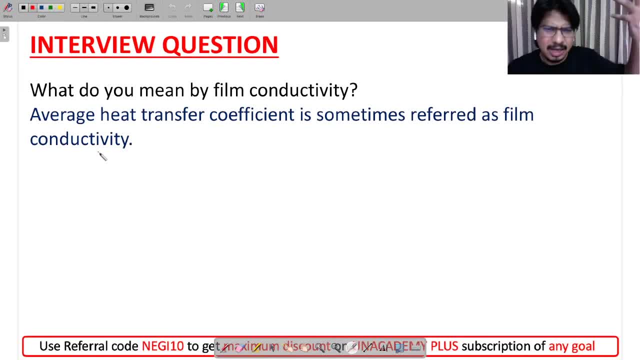 What is the problem? Yes, of course, it's quite possible. Hey, it's Pritam Pyare's mood. Sometimes he can call his girlfriend Aishwarya Rai also. What is the problem? Yes, of course correct. 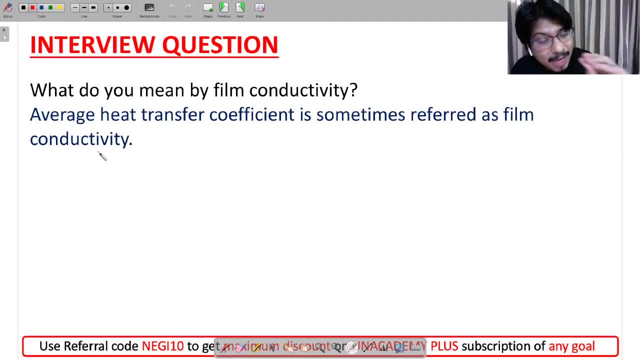 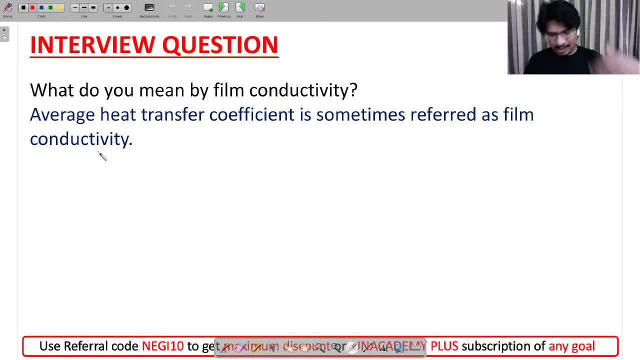 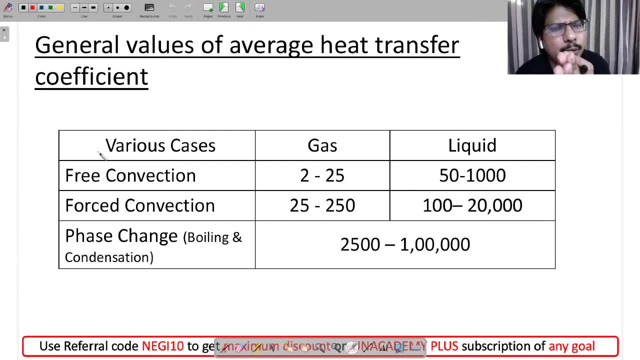 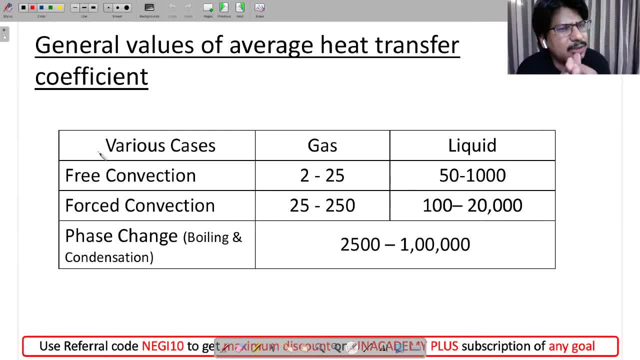 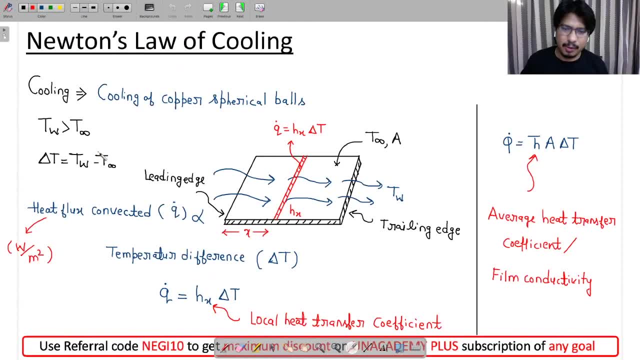 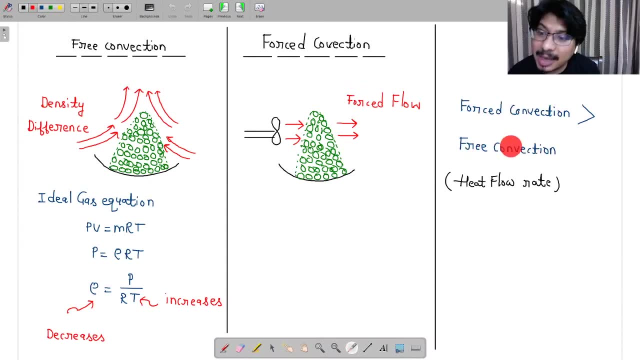 In case of. In case of In case of Close, the convection Heat transfer rate is more. In case of forced convection, your heat transfer rate will be more as compared to free convection. He can't. So I look at here. 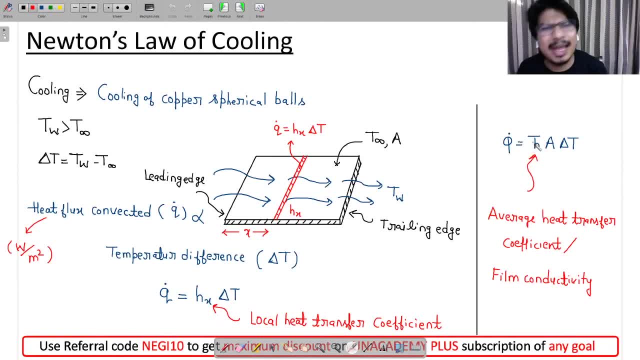 If this heat flow rate is more, 100% H bar is more no If heat flow rate. By doing this, you are having the forced convection, You are having interesting balloons, you are having faster cooling. if you are having faster cooling, what is the? 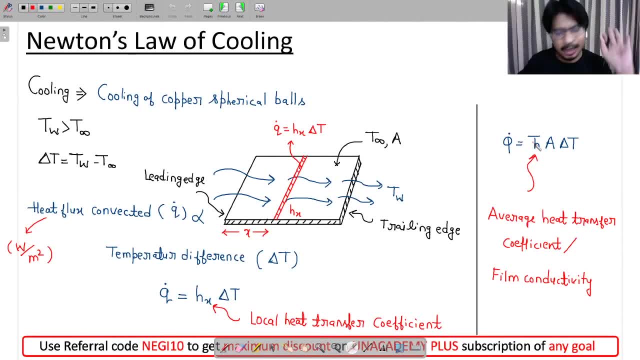 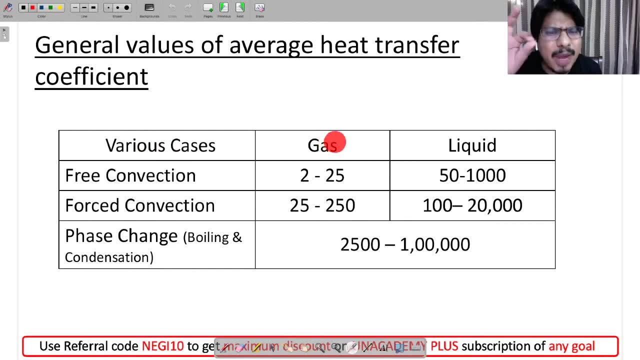 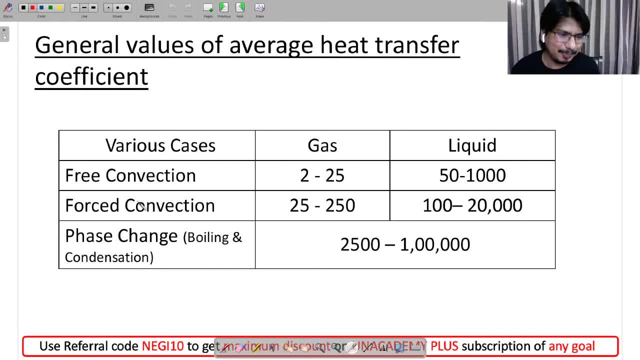 have the feel of the values. so look at here: if I am having free convection with the help of gas, the H bar is 2 to 25. if you do free convection with gas, then the average heat transfer coefficient is between 2 to 25. but if you are having liquid, then in case 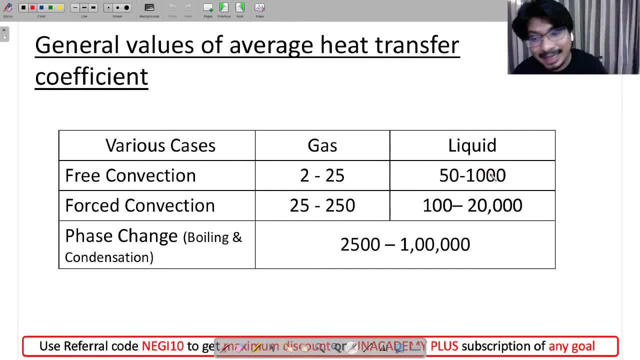 of free convection, this average heat transfer coefficient increases from 50 to 1000. if you are doing the force convection, yes, there is no doubt in case of force convection I should have more value of higher value of average heat transfer. 25 to 250 I'm having. if I'm having gas with the help of liquids, I'm having 100. 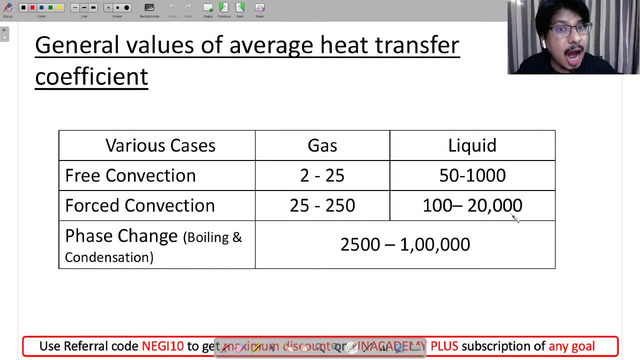 to 20,000 and, by the way, if your phase is changing- boiling or condensation- it will go to 2500 to 1 lakhs also. oh my god, 1 lakh, 1 lakh. now. the question is now. the question is, sir, what will be the unit? what unit are we talking about? what? 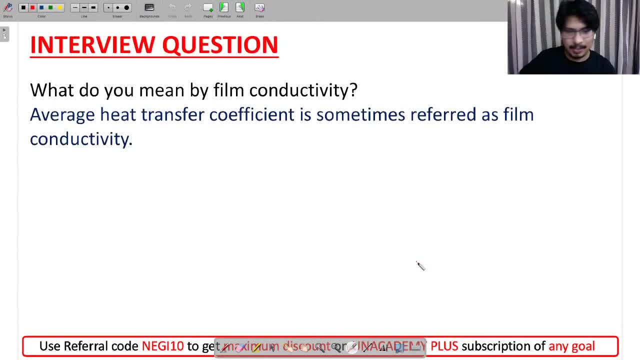 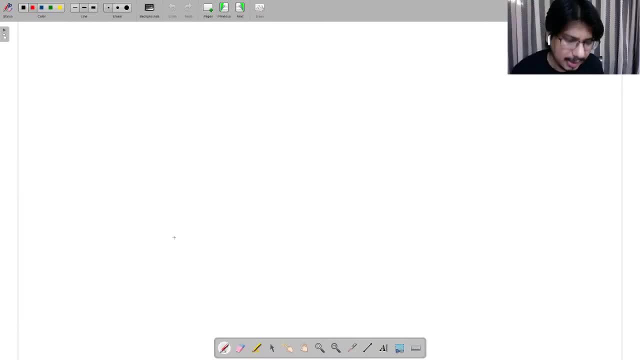 will be the unit of average heat transfer coefficient. so let me explain you map, explain, cut down what will be the unit of average heat transfer coefficient. listen carefully, listen carefully. the key Q dot is equal to excellent, excellent, very good, H bar, a, delta, T, beta. so can I write? can I write? 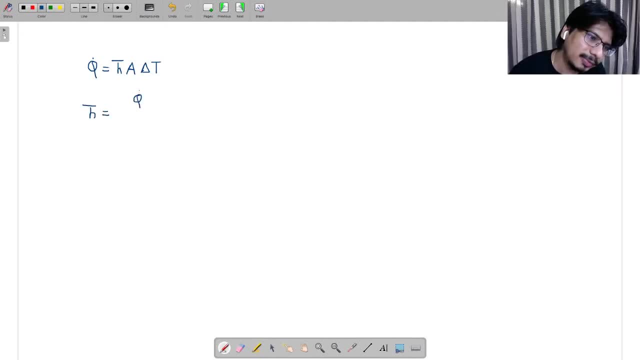 H bar is equal to Q dot you dot, divided by watt a into delta T below a Baba. what will be the unit? what will be the SI unit? what will be the SI unit of H bar? how he is a unit of H bar, what divided by what watt per meter square per Kelvin? 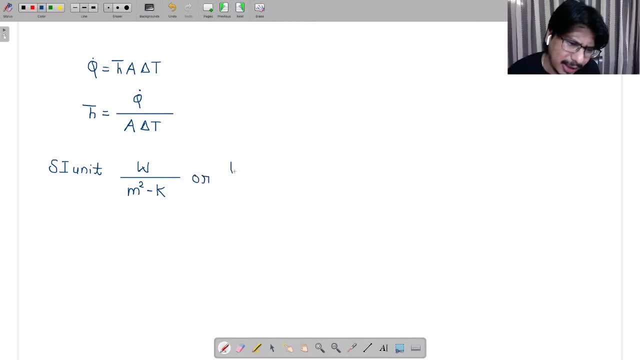 remember it is, or yeah, dricking it a Ek cheez aur yaad rakhenge. I can write in degree Celsius also: watt per meter square per degree Celsius. Don't be confused. Sometimes interviewer is asking you kabhi kabhi, wo aapse puchega in one watt, in one watt per meter square, in one watt per meter square per degree Celsius. 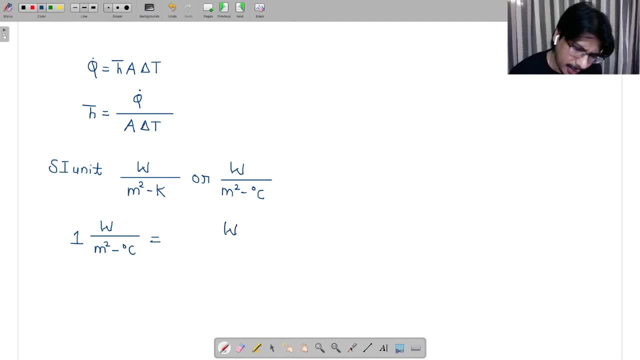 how many watt per meter square, per Kelvin, you will have? Don't start calculating one by two. seventy, three, how much will come? Aare, namune, aare, namune, look at here, look at here, it is the delta T. 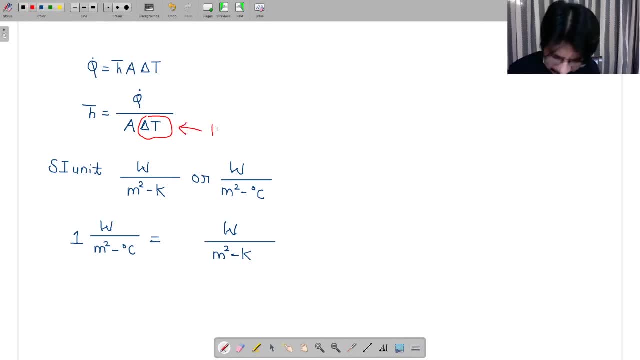 What is the delta T? What is delta T? Delta T is what Delta T is what Everyone tell me. what is this delta T? Aare? this delta T is temperature difference. This delta T is temperature difference. Ye jo delta T hai, ye aapka temperature difference hai. 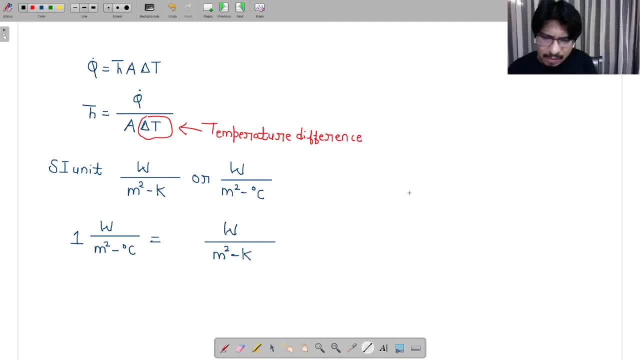 And doesn't matter whether you have degree Celsius or Kelvin scale, temperature difference will always remain same. Temperature difference to beta aapka same rehne wala hai. For example, mai aapko detaun ek example. Let me give you one beautiful example. 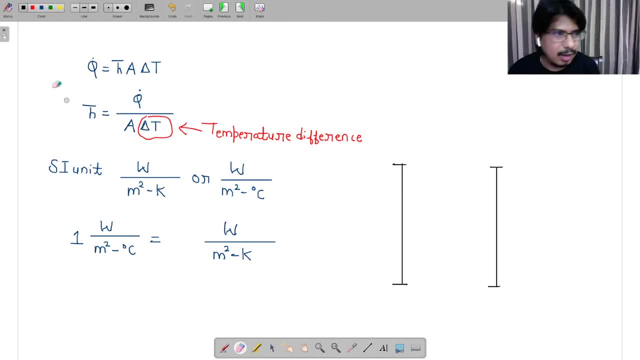 Let us suppose. Let us suppose on this axis. I am taking degree Celsius, ice point, zero degree Celsius, steam point, hundred degree Celsius. Here it is 273.15 Kelvin. If I take the exact value here, you will be having 373.15 Kelvin. 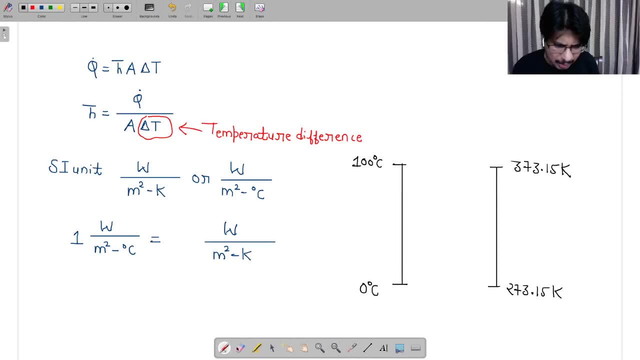 Correct na. Let me take. let me take chalo, kuch toh value lete hain, kuch toh values lete hain, let me take. let me take few values. okay, 25 degree Celsius. 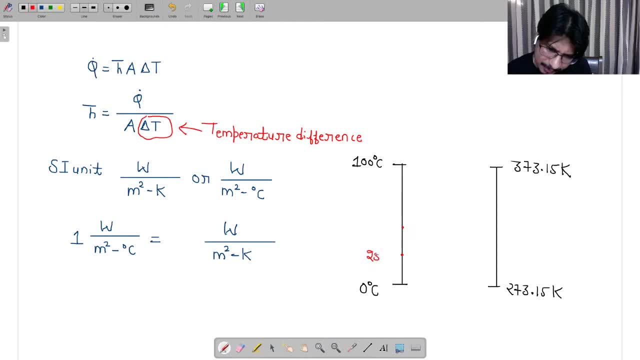 Let me take 50 degree Celsius, 25 degree Celsius, 50 degree Celsius. What will be the value of 25 degree Celsius in Kelvin scale? Kelvin, mein kitni value. hogi beta, Bolo re baba, bolo re baba. 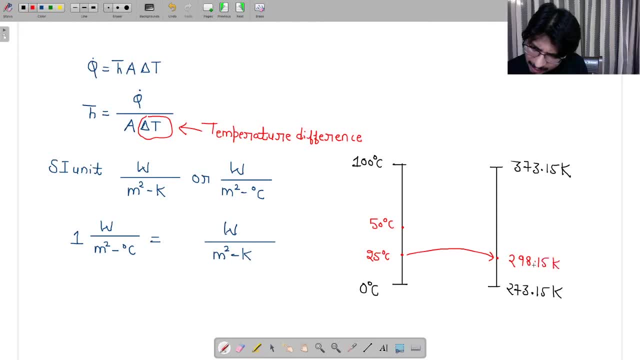 298.15 Kelvin Thike. What will be the value of 50 degree Celsius in Kelvin? Bolo re baba, bolo re baba, bolo re baba. 50 degree Celsius in Kelvin. how much? 3.5 Kelvin. 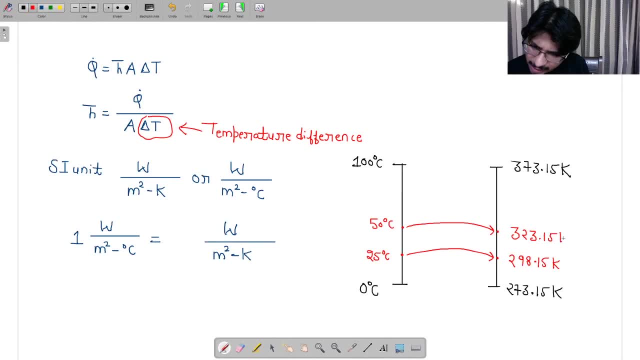 23.15 Kelvin. But if you see the difference, If you want to find the difference, Difference will come exactly same. Difference will come exactly same. Look at here: 50 minus 25 is how much 25 degrees Celsius. 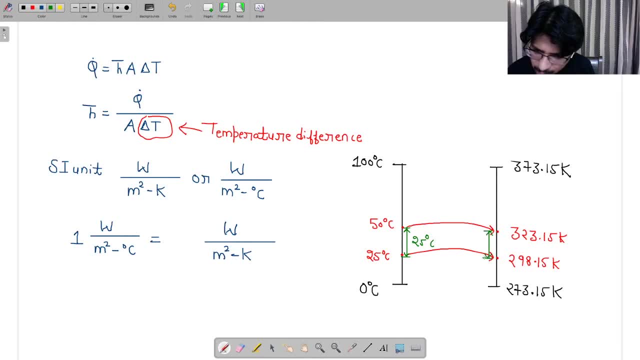 3.23 minus 2.98 is again 25 Kelvin. So always remember temperature difference is same, So please don't start solving. 1 watt per meter square per degree Celsius is 1 watt per meter square per Kelvin only. Yes. 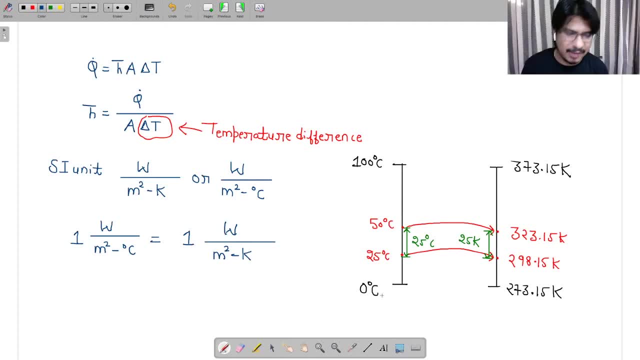 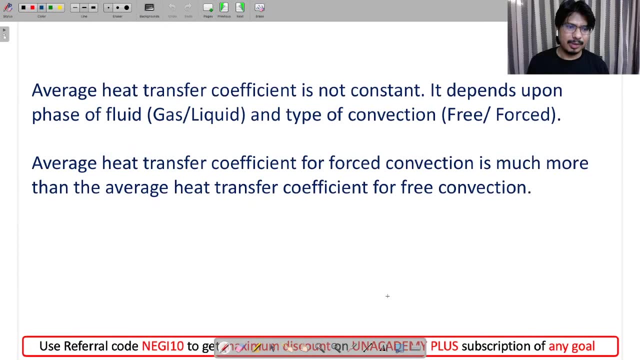 Yes, Is it clear to everyone? Everyone is clear: Shall we move forward? Will we move forward? Tell me, Will we move forward? Will we move forward? So see, Yes, Yes, Yes. Average heat transfer coefficient is not constant. 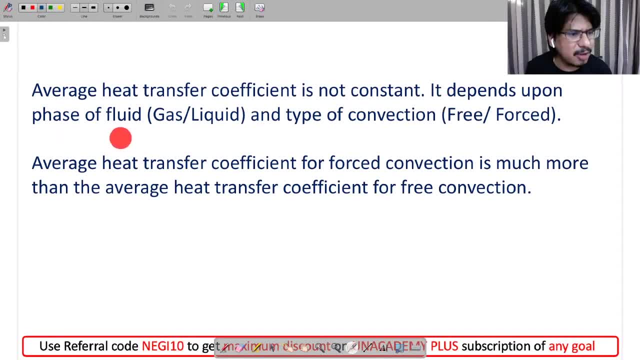 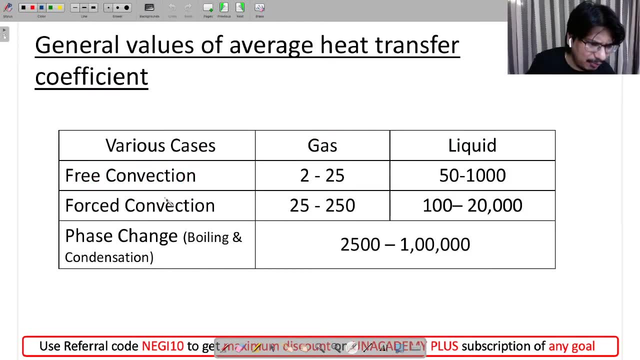 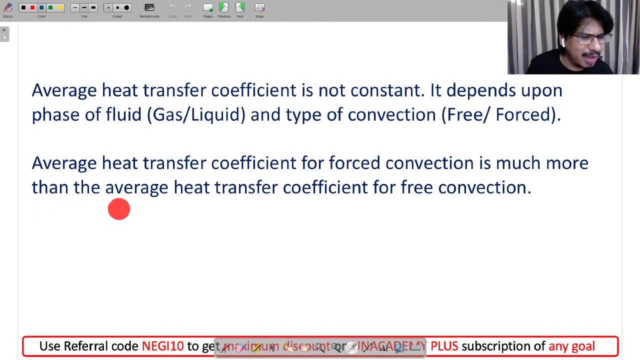 Of course we have seen it is not constant. It depends on the phase of fluid and type of convection. What is fluid? Is it gas or liquid? Whether I am getting free convection or forced convection, Average heat transfer coefficient for forced convection is much more than the average heat transfer coefficient for free convection. 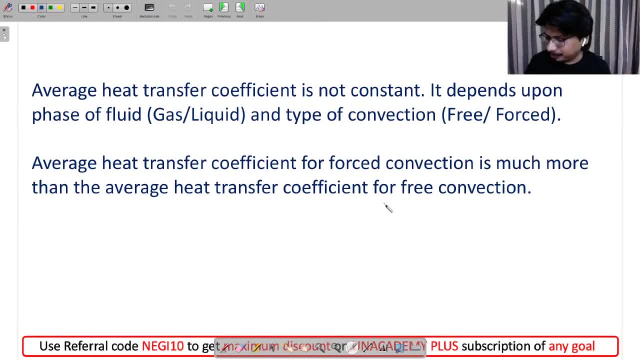 Is it clear to everyone? Tell me, Is it clear to everyone? Are you clear up to here? Are you clear up to here? Are you clear up to here? Very good, Very good, Excellent, Excellent, Excellent, Excellent, students. 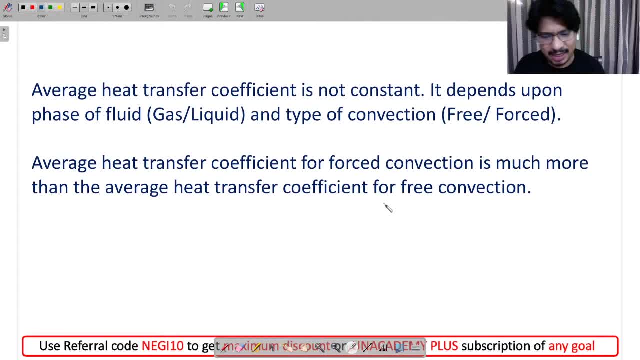 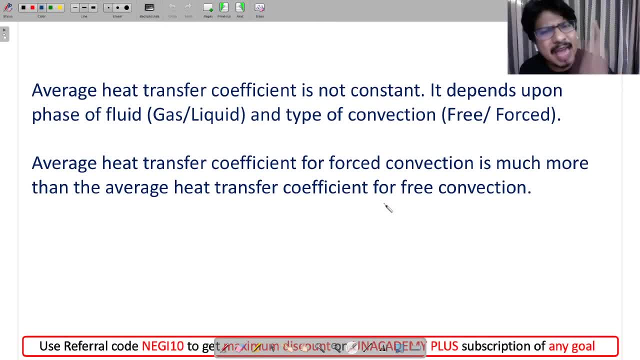 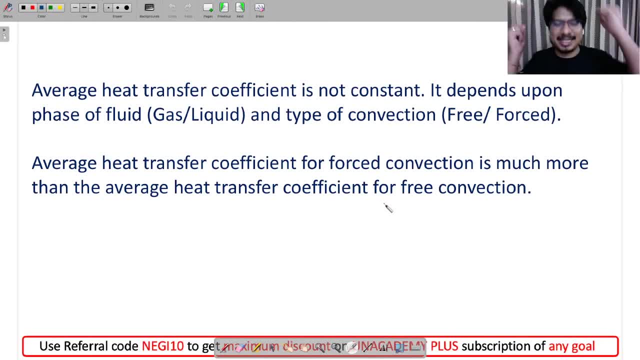 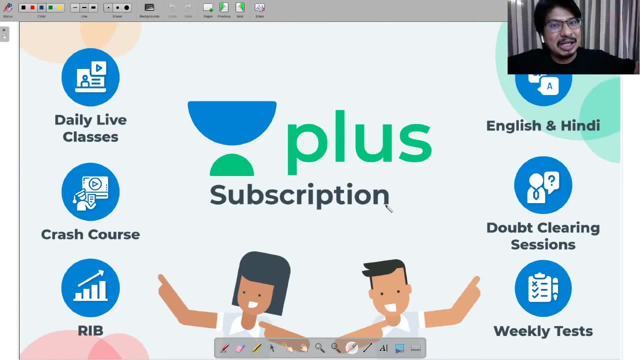 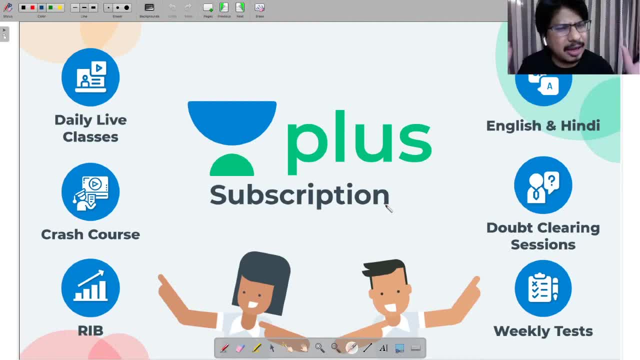 Aaj se bitta nai batch start ho gaya hai, Nai batch Unacademy Creatrix team ke nai batch start ho gaya hai. You know, aapko pata hai, kaun-kaunse batch start ho raha hai. 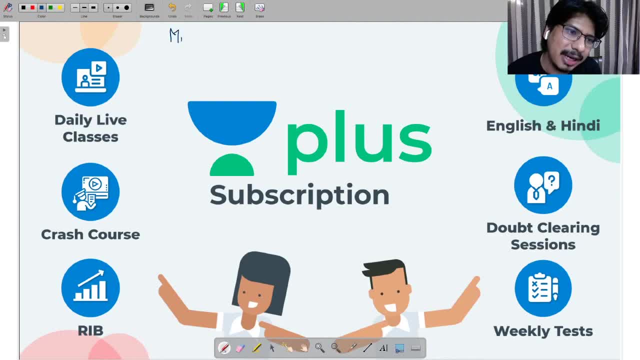 Kaun-kaunse batch start ho raha hai re baba. bolo re baba Mission Gate and ESC. From today we are starting English batch. we are starting today. Start kar diya re baba English batch. start kar diya aaj se. 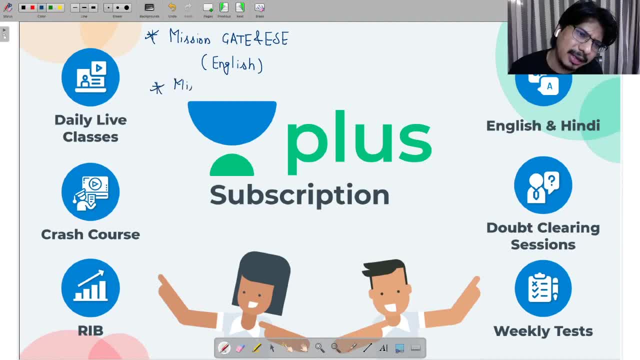 And another batch also. we are starting from today only Mission Gate and ESC 2021, 2022.. Mission Gate and ESC Hindi batch is also started from today only. In this English batch. I will take the subjects in both batches. 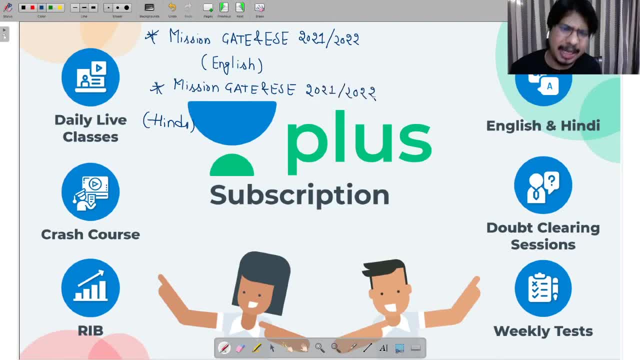 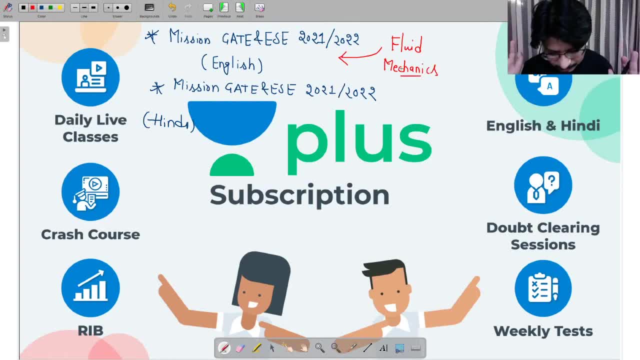 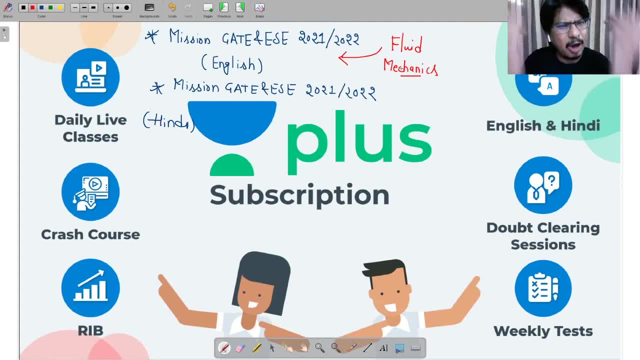 Yes, Balrajoo, Our mission is getting launched like missile. Now, listen carefully. Today evening Abhi aapko Class khatam karke. I am going for the plus Jama Jooojamo Fluid mechanics. I am going to discuss. 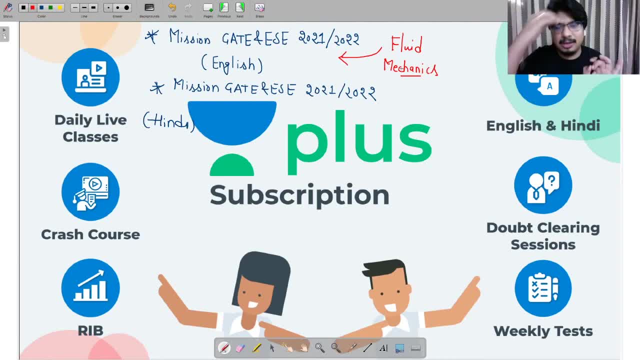 120 plus hours or whatever the classes I will take. that will be applicable for Get ESC in Ring Services examination, Civil services examination as well as upcoming IRMS, also Technical slaves- same. We will be solving previous gate questions in Ring services questions And civil service exam. 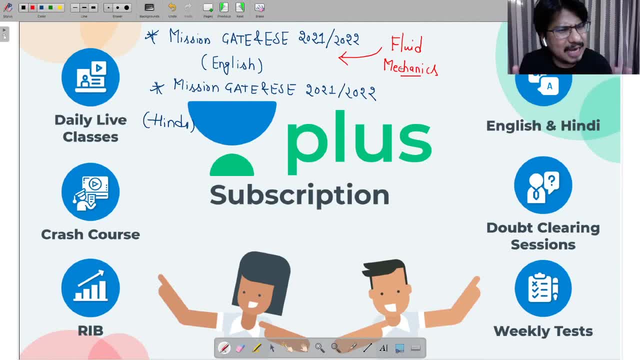 civil services questions also. so, my friends, please understand, please understand. there is no doubt you people are asking: sir, definitely, we are going to take the classes on youtube, there is no doubt. but there is a difference between youtube and an academy. plus, you people are attending the special classes also. you can understand how beautifully we are interacting with each other. 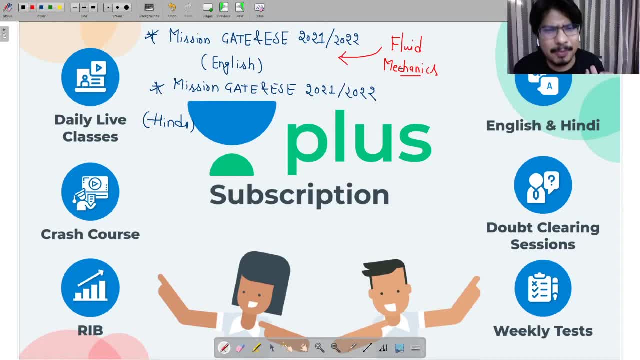 how beautifully we are interacting with each other on an academy plus youtube generally. what happened? the biggest drawback is: youtube was never meant for education. it was never meant for education. we are trying to bring it on, but unfortunately there is a lag. always it is very difficult to have two-way communication on youtube. whatever i'm saying. whatever i'm saying. 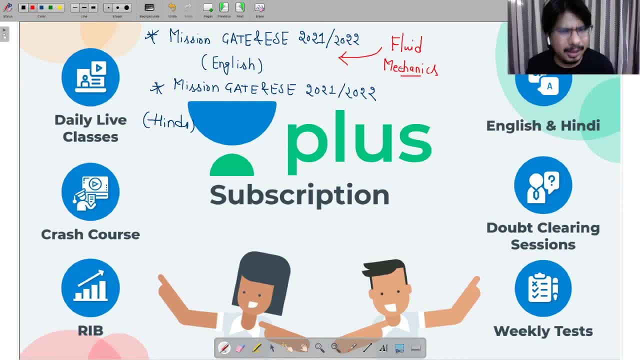 it is reaching to you people. maybe after 45 seconds or one minute. by that time i will be in rhythm, faculty will be in rhythm, and they will keep on saying the other things. they cannot wait for one minute, right, it's very difficult, but on an academy, plus the beauties, it. 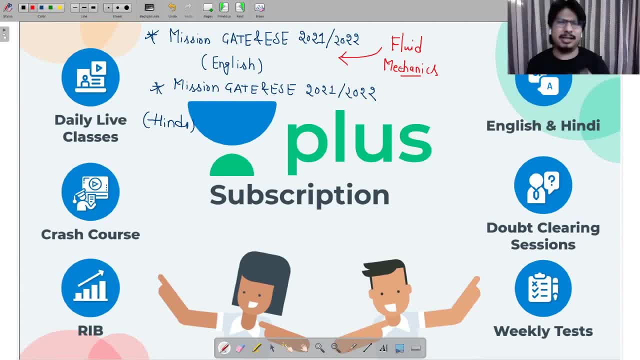 is real time. if you want personalized guidance, if you want to get the rank- i'm not saying on youtube 100%- whatever we are committed we will do, don't worry about the content, don't worry about the content, content. we will not never compromise, either on youtube or plus, that these are not our. 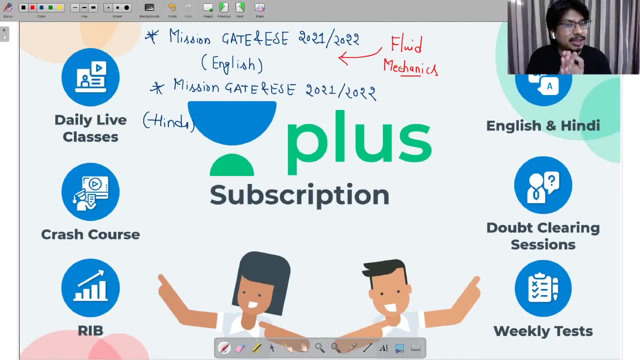 ethics? definitely, we will stick to the content, but try to understand. on plus, every day you are having six hours class, personalized guidance, so if possible, if possible, try to join an academy plus as soon as possible if your financial condition is supporting. it is not compulsory, but financial conditions support you so you can give yourself a chance. you can give a chance to yourself. 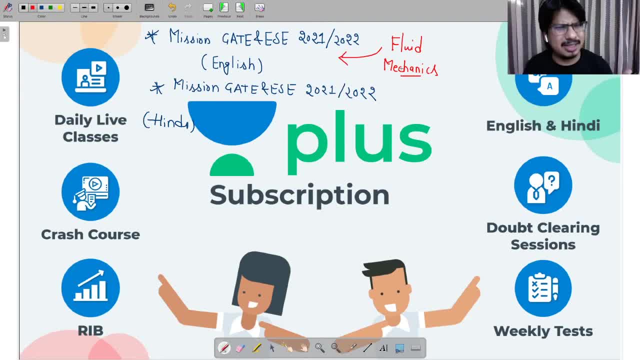 yes, i will give the hundred percent to my this competitive exam attempt. this year. they go, don't worry, in any competitive exam, two things are very important. two things are very important: revision part and practice part. so we are taking care of that. we are taking care of that for. 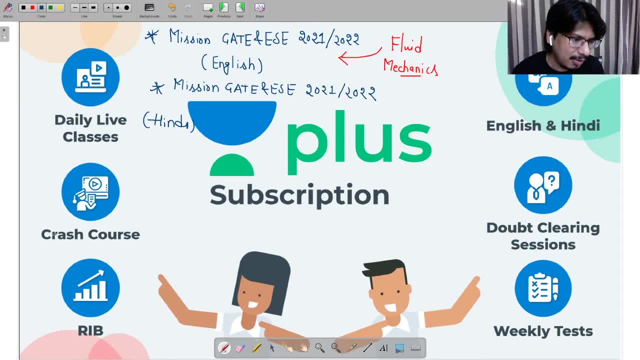 revision part. for revision part we are having crash course. for revision part we are having crash course. for revision part we are having crash course, whereas for practice part we are having rank improvement back where we'll be solving three thousand to three thousand five hundred questions. so you can attend these classes also. 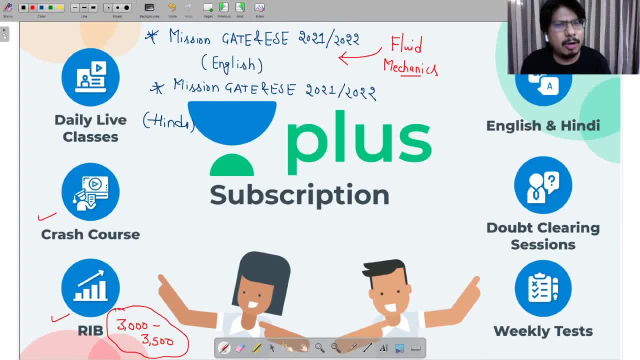 you are able to attend the syllabus. you are able to attend the revision classes. at the same time, you are able to attend the practice classes also. you are able to attend the classes also off recording classes. also. the way we have planned our schedule, we have planned in such a way that morning and evening 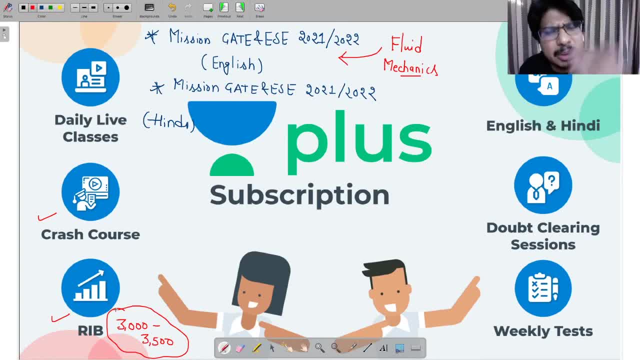 so if you are working professional doesn't matter. if you are college going student doesn't matter. early morning and late evening, you can see the live videos and live videos. the beauty of the unacademy platform is: every fourth class is doubt clearing session. every fourth class is 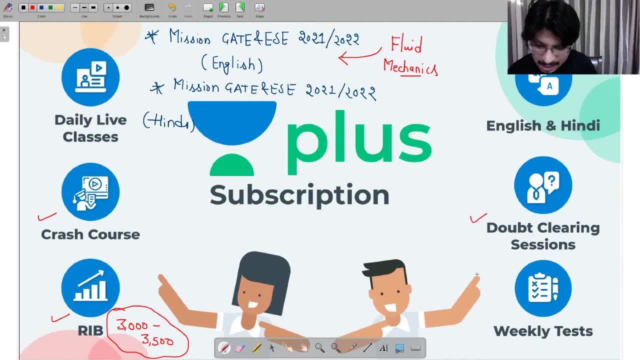 doubt clearing session. every fourth class is doubt clearing session and every week we are conducting the test and we are conducting the live classes. this youtube is lagging, but when i'm saying live classes means one-to-one interaction. the moment i'm saying something, it is reaching to you and 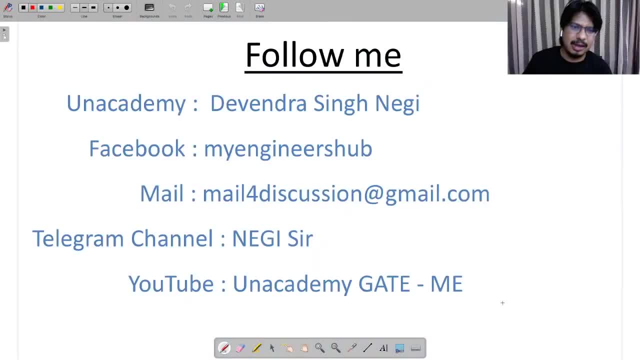 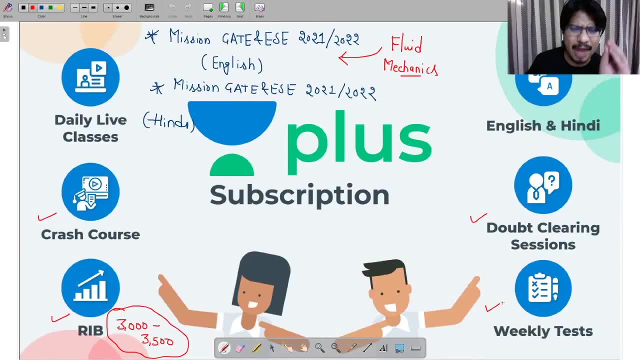 immediately. you are typing and you are replying. that is for live class, now, now. now, if you have any doubt, if you have any doubt regarding how to pay the fee, what will be the duration of the course? look at here. let me give you some details. you people will be interested.